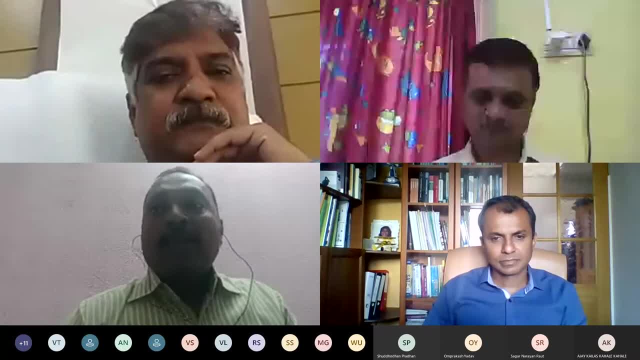 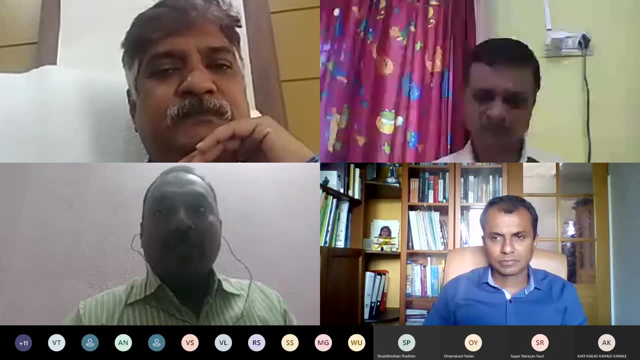 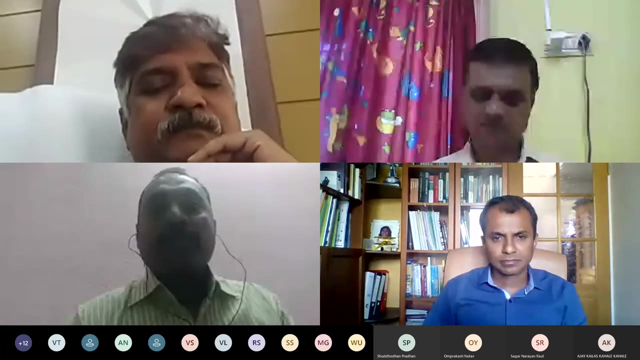 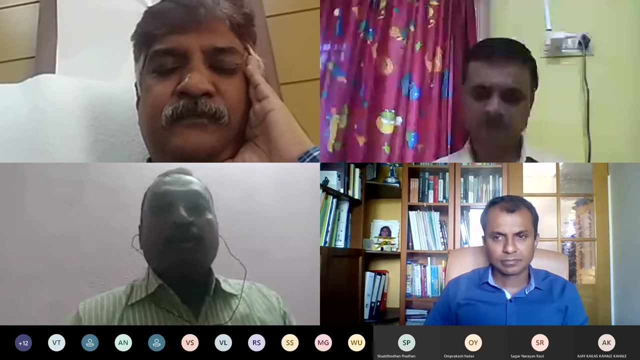 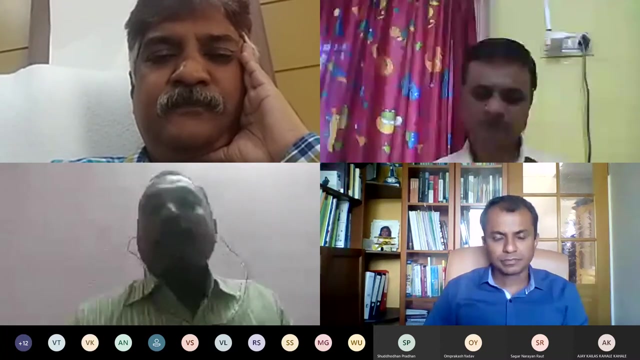 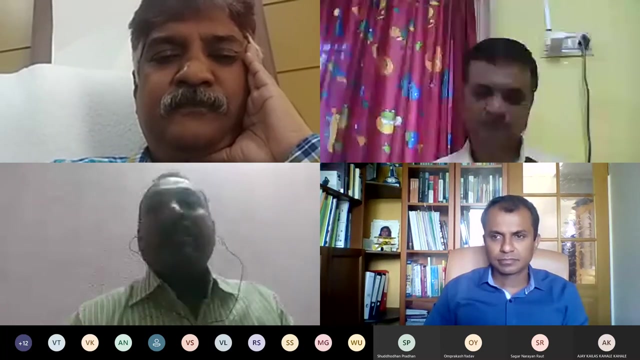 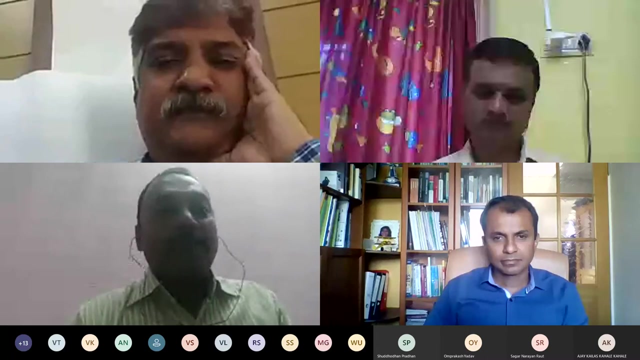 Concept Validation Study for Fusel-LG WIC Filling Propulsion Investigation, Combined Cycle Engines and Logistics. Schönbrunnen, Ant. excellent research partners with NASA International grup-WIC Talent Foundation. AA đang mel is 24.. we are very much happy and pleased to have you today with us, dr erwin. now i request. 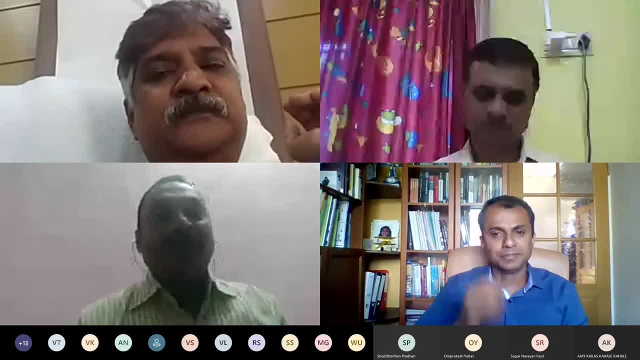 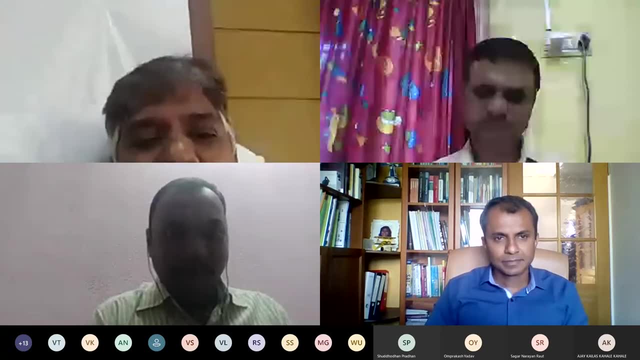 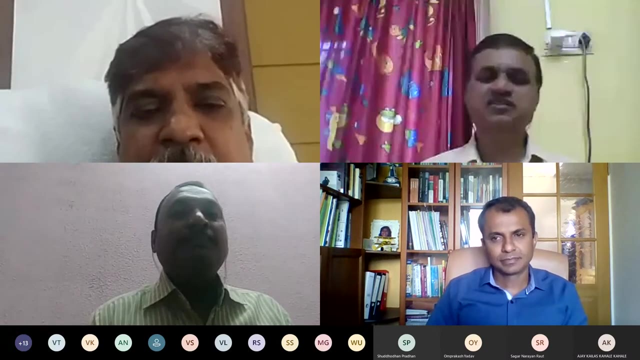 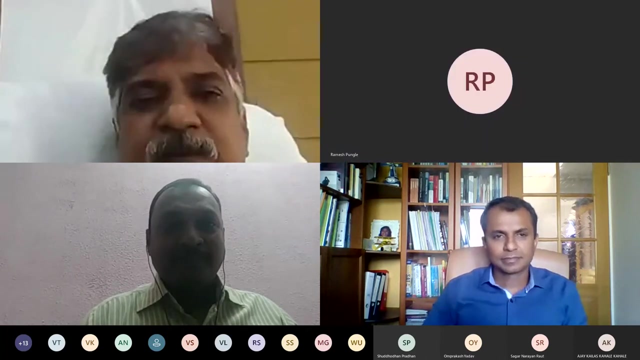 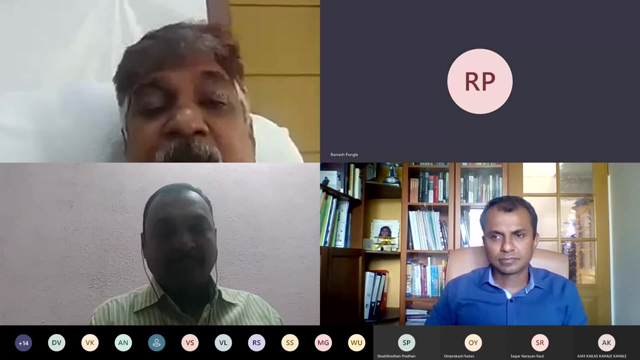 a principal, dr abhijit vadekar, to share his views. sir, yes, i'm audible. yes, sir, yes, sir, uh, good afternoon everybody, uh, with the due respect to the idols of lord buddha, buddhi, sattva, bharat, ratna, dr b r m vadekar, the keynote speaker and our 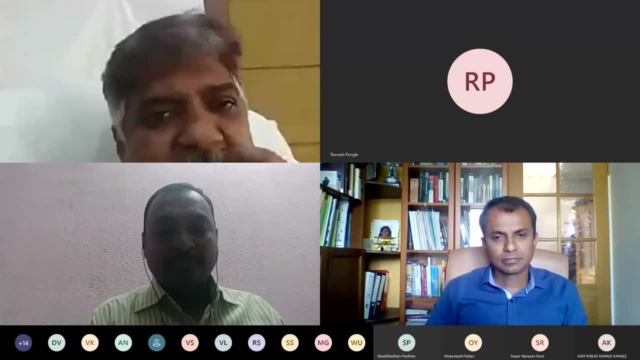 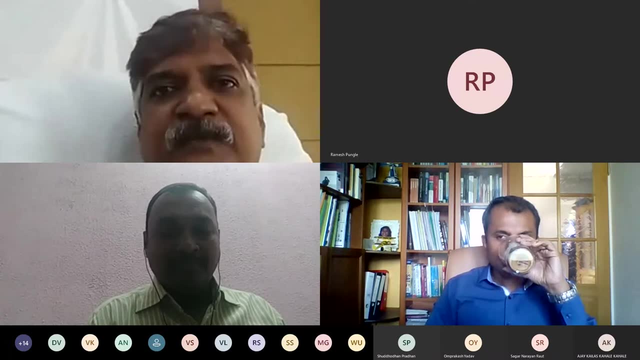 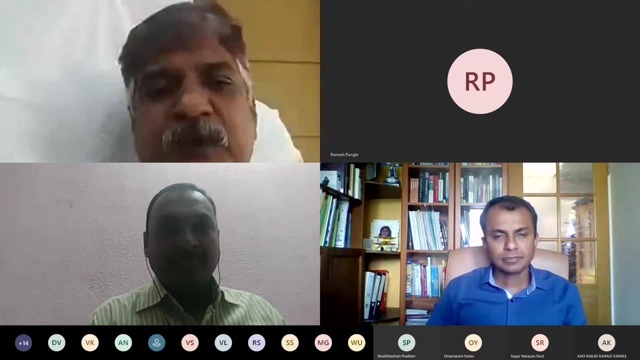 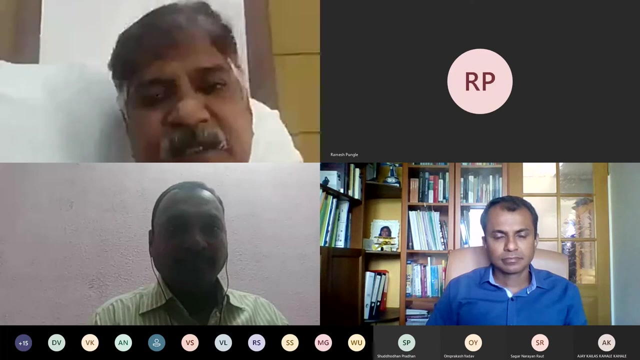 own member of the ps family, our alumni dr arvind rao, associate professor delt university of technology netherland, head of the department, dr kungley, professor prashant pandit, all the faculty members, all the participants and my dear friends. at the outset, it gives me an immense pleasure. 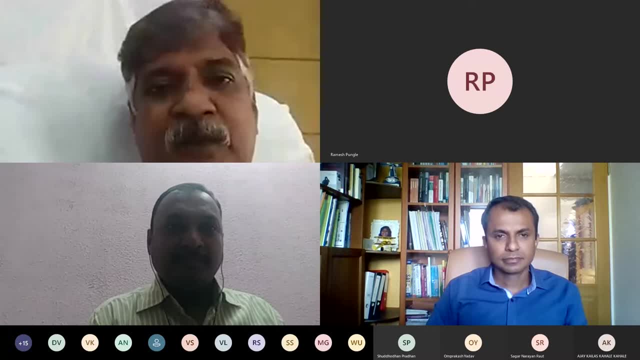 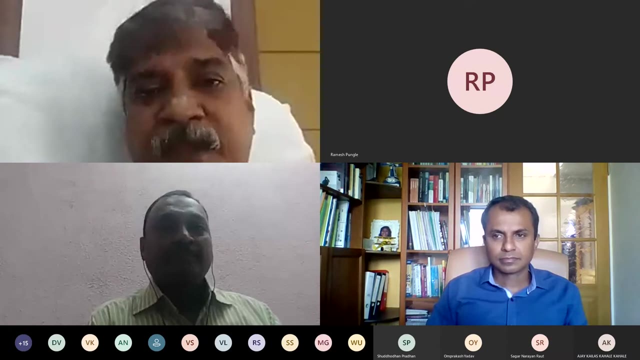 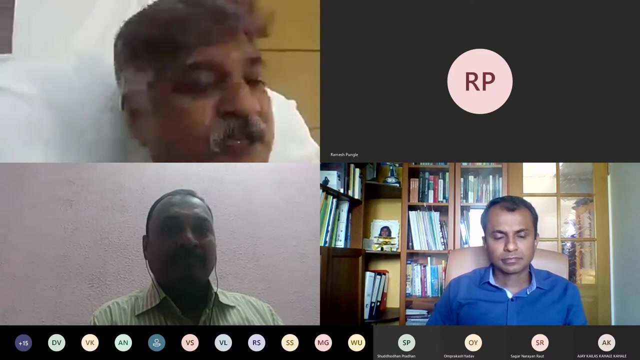 to to say that our own alumni's are come forward and accepted this invitation on behalf of myself and my institute, all the faculties. i extend my warm welcome to dr arvind rao as well as thank him for accepting our invitation for this webinar on the topic. 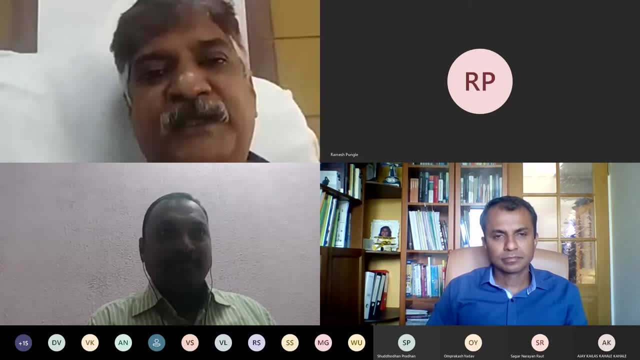 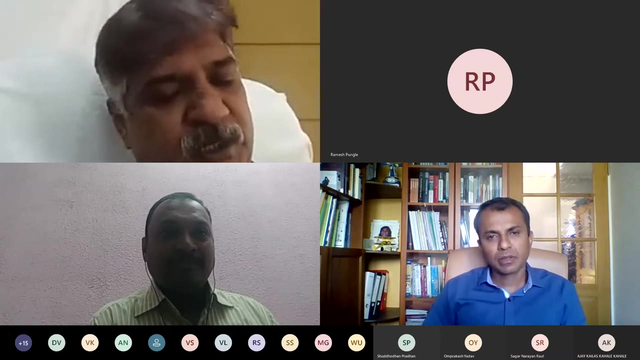 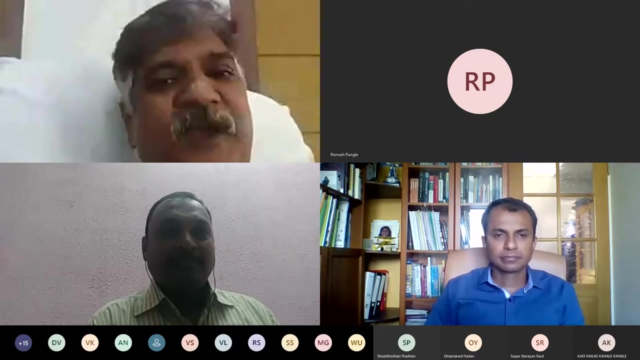 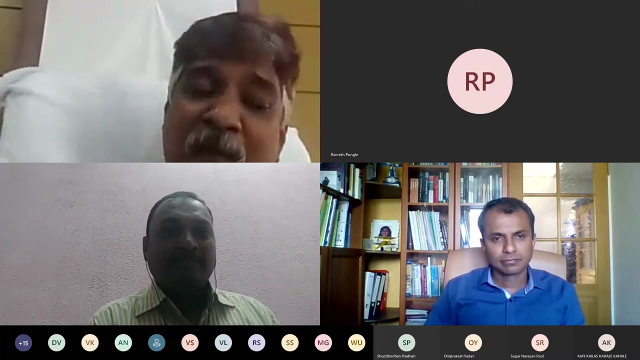 the aircraft propulsion, as everyone of us know that the objective of the People's Education Society is to promote education, not only education, but to promote intellectual, moral and social democracy. So Dr Arvind Rao is the product of PS, is the best example of an intellectual the moral. 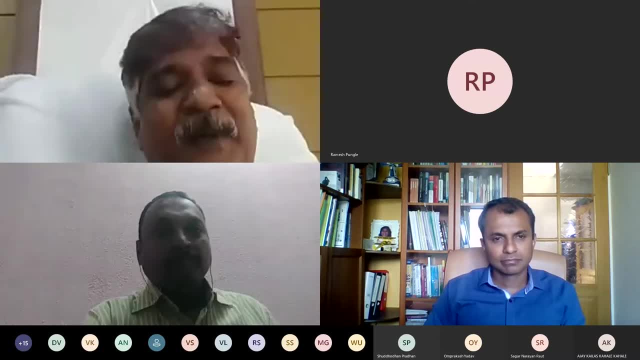 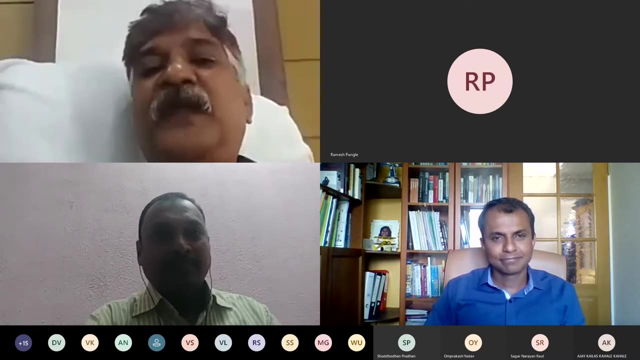 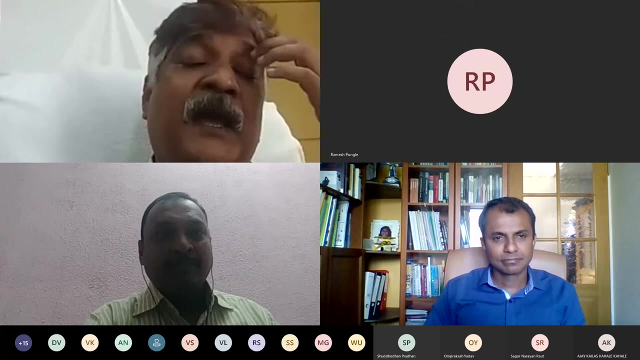 and the social commitment how he has been again connected and accepted by accepting our proposal and educating our people, our own people. So I once again thank him. Second, I congratulate the head of the department and his team for organizing such a good webinar. 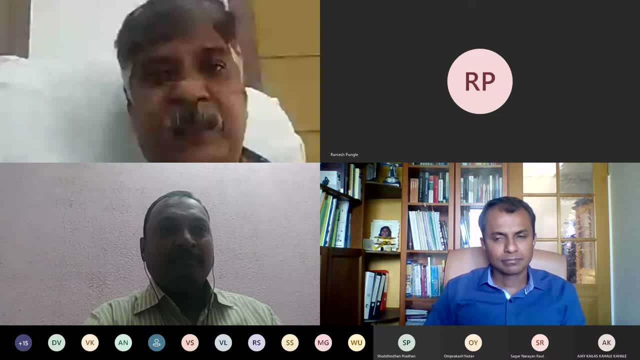 and selecting such a nice topic. So again, Professor Punggle told in his webinar in the introductory speech that he wants to connect all the alumni and invite all the alumni to come and participate in this. So I congratulate him. Thank you very much. 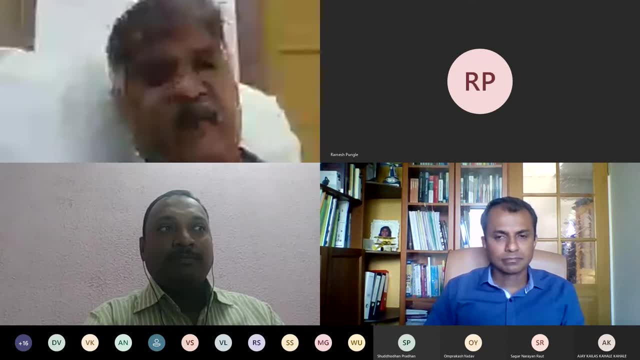 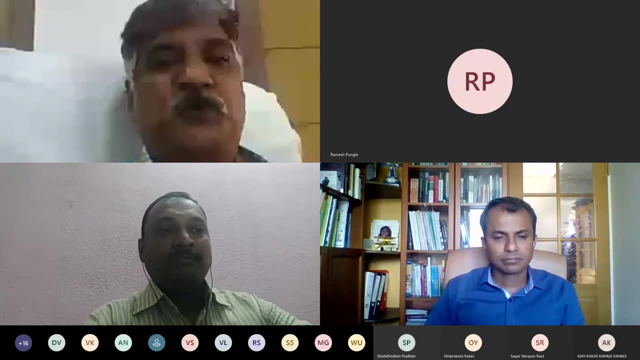 I wanna thank all of you very much And the way I'm representing I want to teach the students. they want to feel recognized in the webinar series and teach the students. It is the need of an hour When we say that we want to make our students as well, as the faculty is also required to 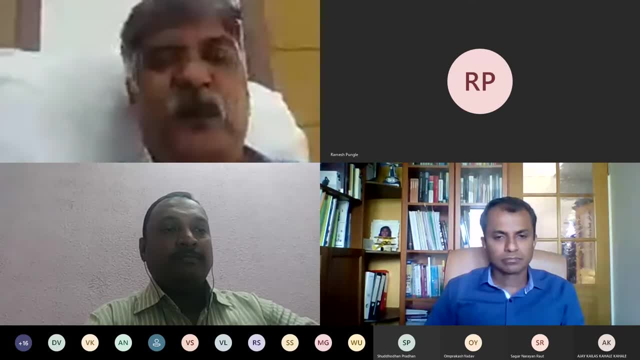 be upgraded. We are required to know the outside world. So the Covid has taught us a lot many things. It was not possible for Arvind to come to Arangabad and share his views. It was very difficult for Arvind to come to Arangabad and share his views on the UN, Joseph. 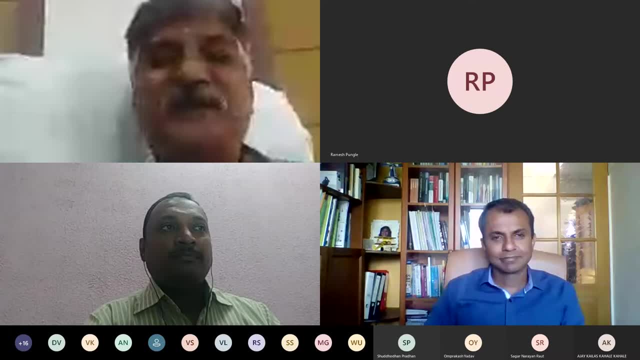 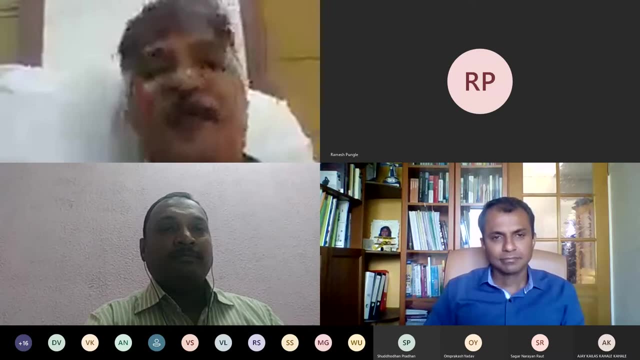 Institute which he all the time has prioritized, the work of the Pr Furkl, the IPC and other Jet experiences and teachers. so this platform has helped us to connect arvin. the covid has helped us, rather, i would say, to connect arvin and share his wish with our people. 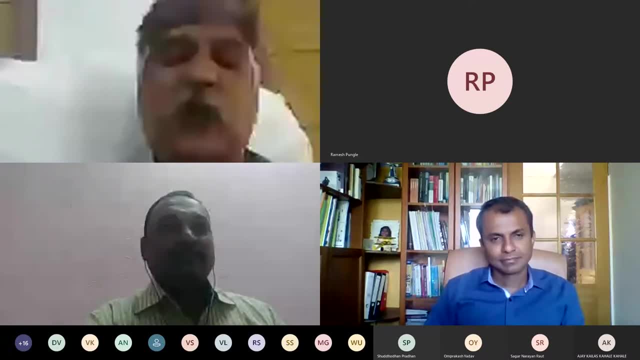 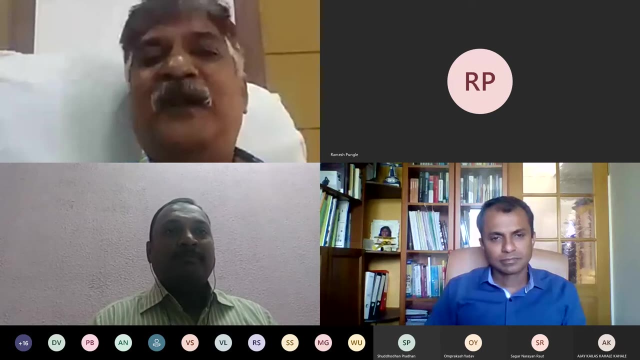 so, my dear friends, now this whole term is going to be online and we are required to take the maximum benefit of this, so i will not take much of the time we are running. already delayed this particular program. we were supposed to start at two o'clock but because of some technical problems, the program has been delayed. i will not take much. 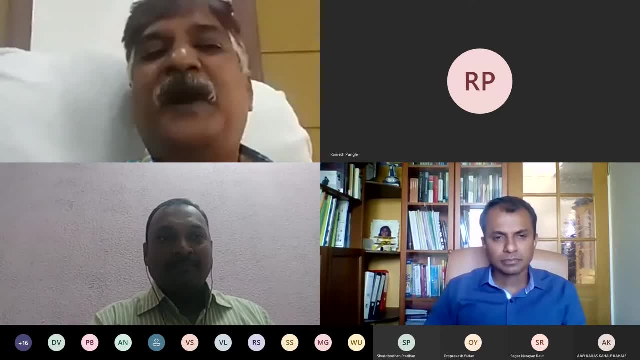 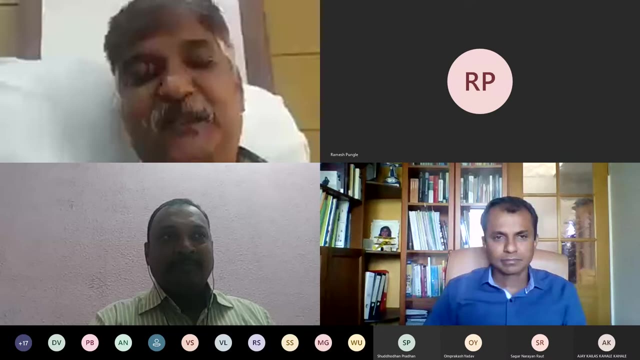 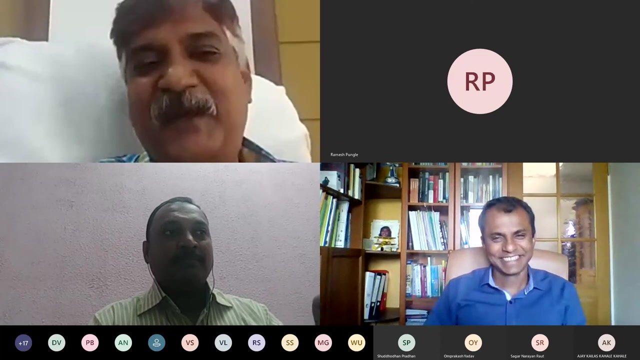 of the time. i once again wish all the participants, wish them a happy learning and wish everyone you for very good luck. and again, pungal sir has wished me because it is a very nice day for me. today is my birthday and arvind is delivering his speech and really when he was there as a student, 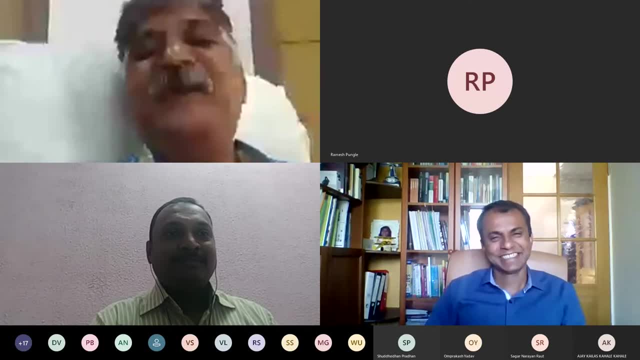 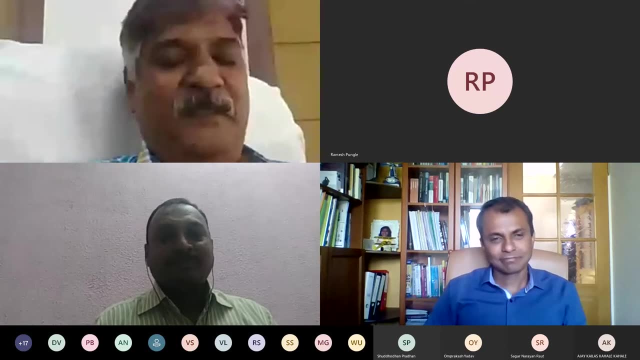 i used to call him as a scientist. really he has brought all my dreams come true and really he is a scientist. everyone of the participants have been at this platform for years and a half and if our participants were there on this platform should patiently listen to him and 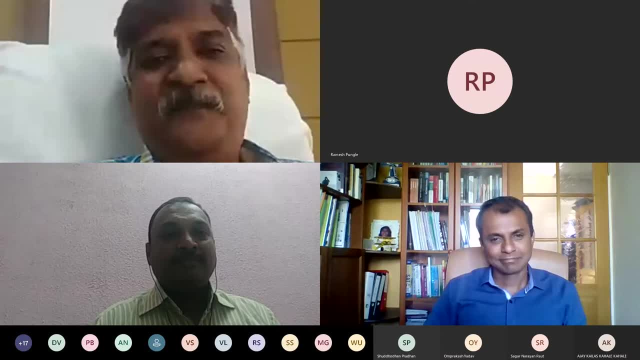 be connected with him in forthcoming years. i am confident as and when we require any of the help from our alumina's, they come forward and they are ready to help us. i also express my willingness that arvin should connect with you people on Italia. bara, you see in комнаt. 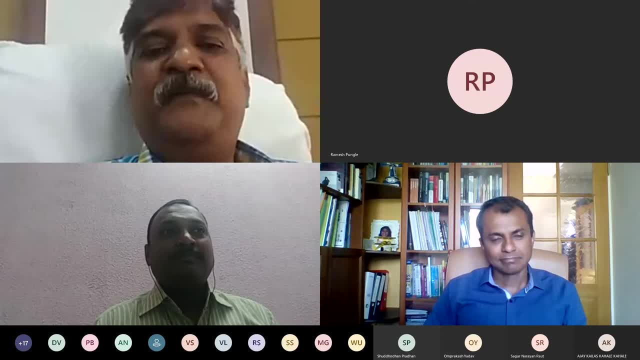 you know we are connected to each other right now, from iran, everywhere. we are asking that people understand. you should know that you are already a diyor, so that it is very much with this institute. he is very, he has a very strong platform in the research, so there should 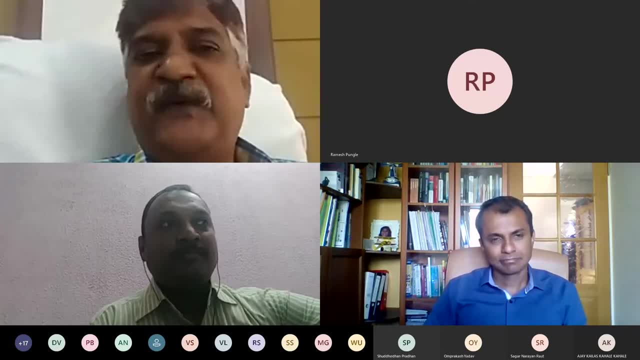 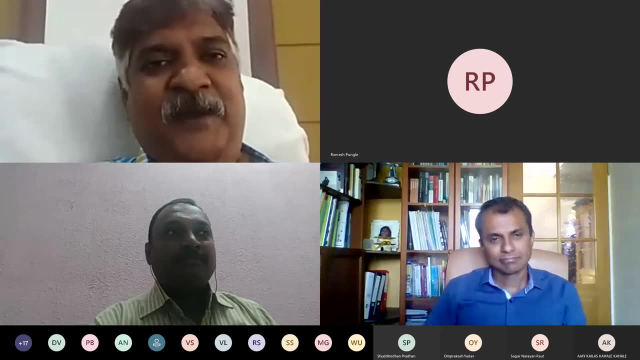 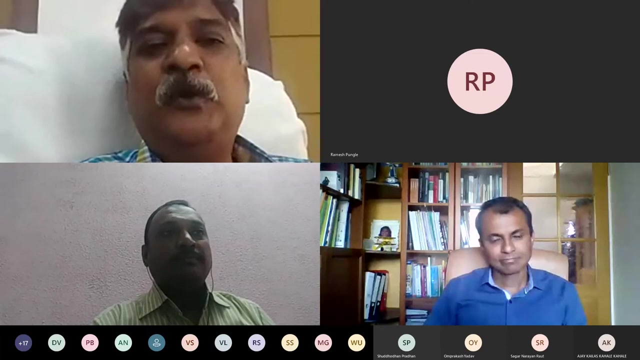 be a contributory research works with the faculties. he should strengthen the research activity in his institute. okay, so this is the desire which i feel sincerely: that he should come forward and collaborate with us as far as the research activity is concerned, so that students will get an hands-off experience to work on the live projects. unless and until we don't work on 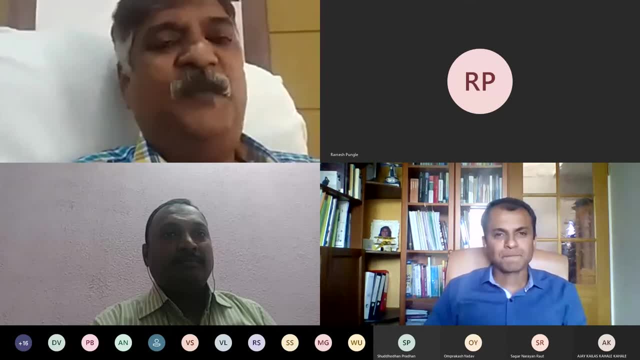 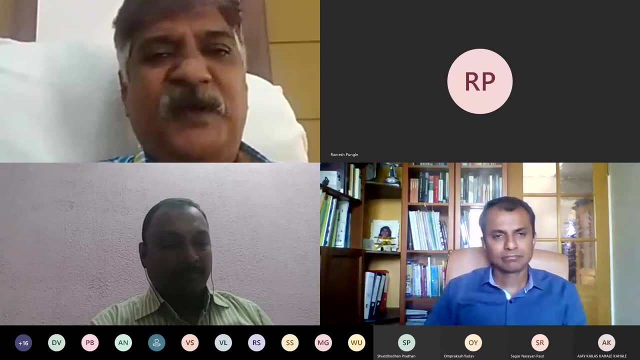 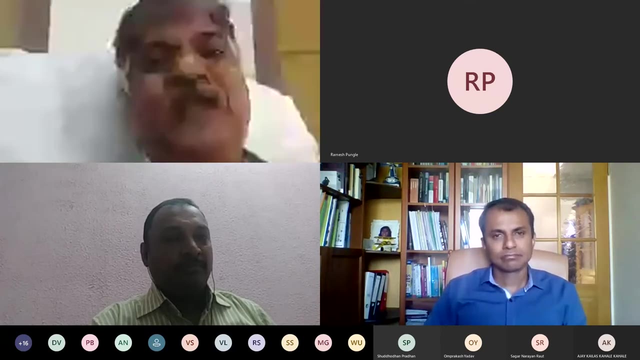 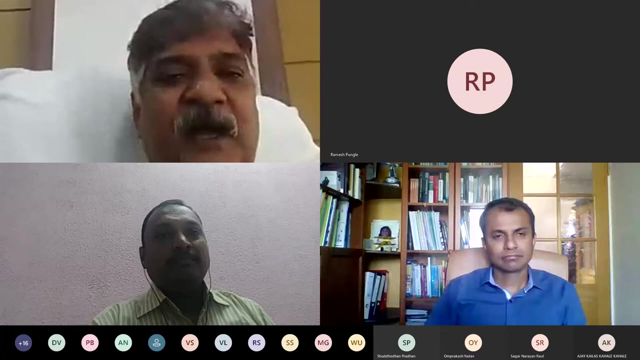 the live projects, the students. we cannot say they will become employable. things have changed. engineering has become interdisciplinary. any person can learn any of the subjects on the engineering. those days have gone. only the student, students from the computer science, uh, you to learn only about the software engineering. now everyone has to be, uh, accept the change which is. 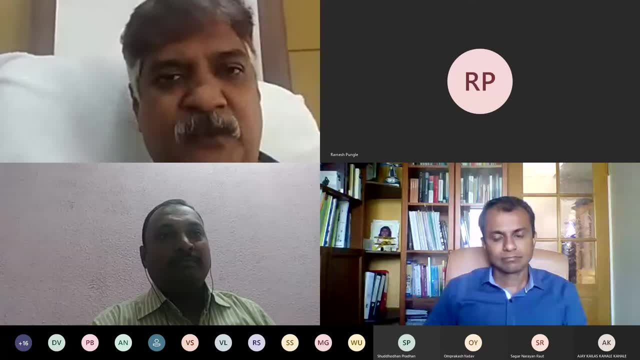 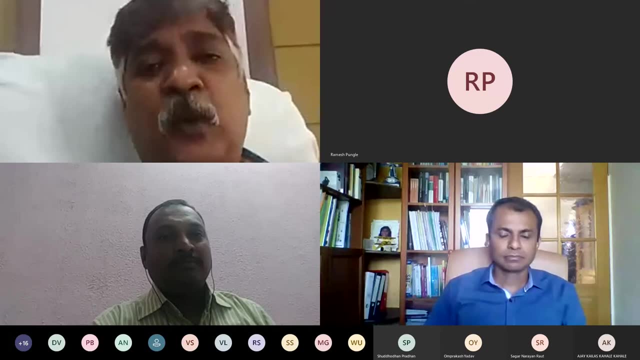 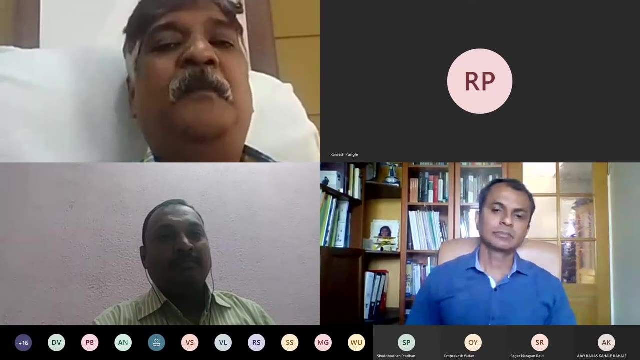 uh, which has taken place in the industry. so it is the world of an automation and we are required to know a lot, many things. in addition to the core subjects. we are also required to know about the software engineering. we are required to know about the python, machine learning and whatnot. 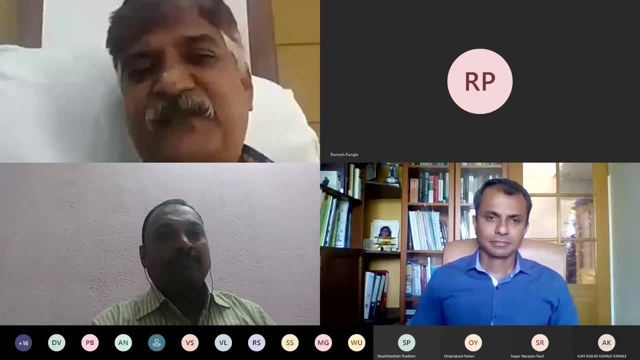 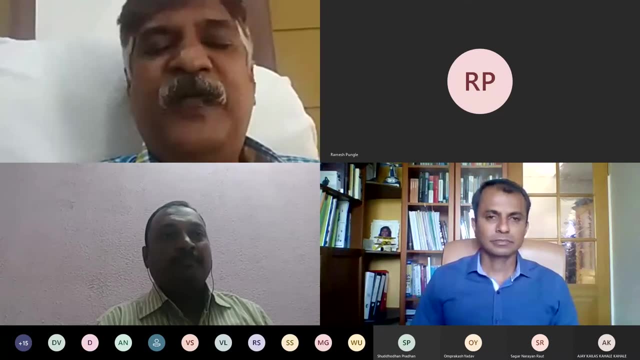 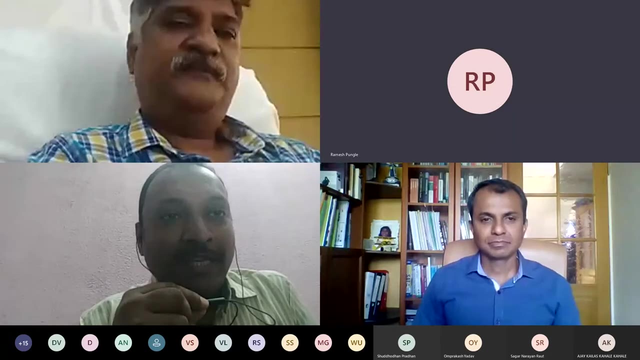 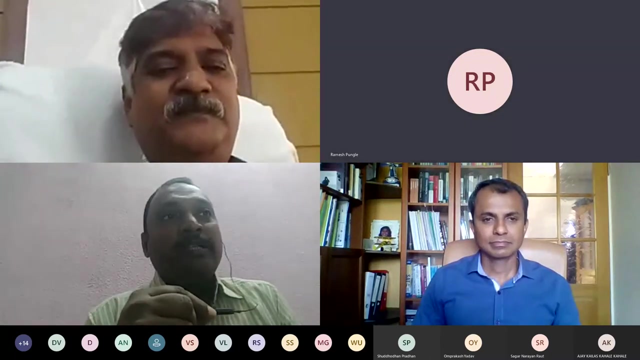 artificial intelligence. so, my dear friends, i once again thank you for the patient hearing and, uh, wish you a very happy learning. thank you very, very much. thank you, sir, and wish you once again happy birthday. now i request all the participants to fasten their seat belts and i call our honorable guest. 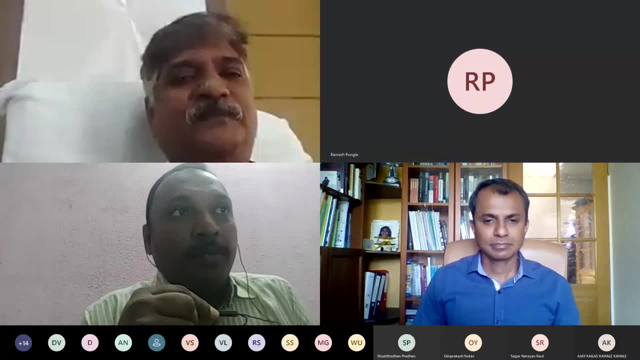 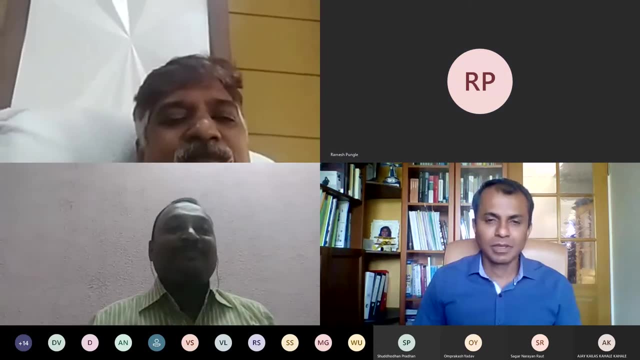 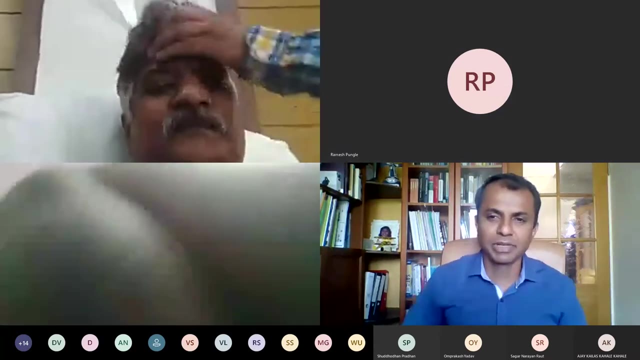 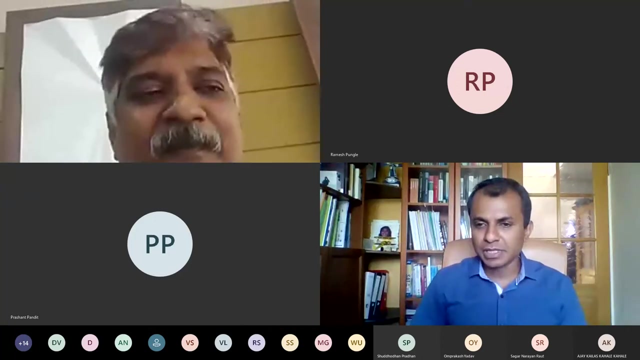 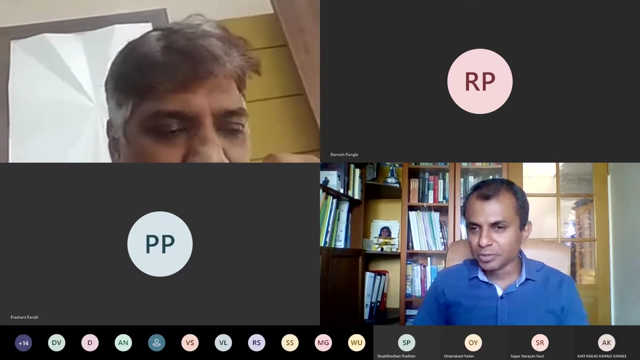 speaker, dr arvin browser, to share his variable thoughts about the fundamentals of air, air, aircraft and the development of the aircraft, and the development of the aircraft and the development proposition. so over to you. um, thank you, uh, thanks a lot for the nice introduction. uh and uh, first of all, like it was, 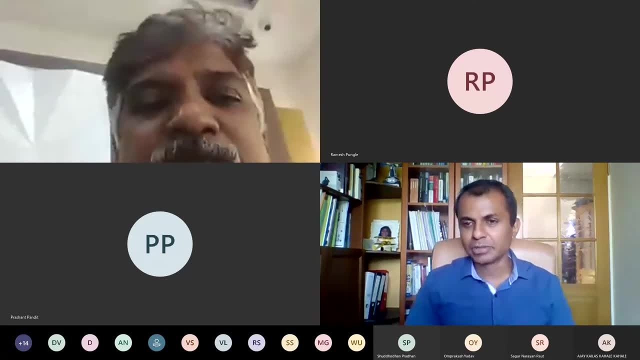 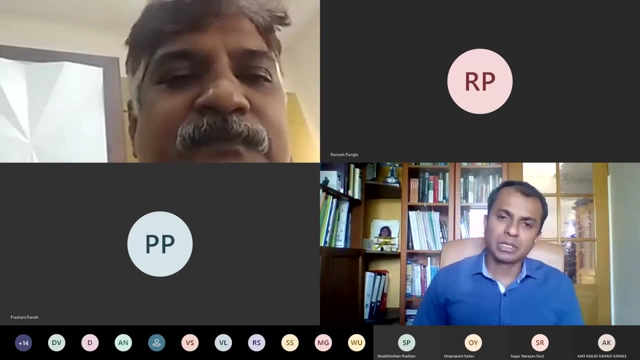 it's very nice to connect with you all. uh, once again, happy birthday. uh, radical professor, and i also see some of my, some of the older faculty members who have joined. uh, i saw Mr dohbe as well as mrtheiteh. so good you all. So, as Professor Variga was mentioning, you see that COVID situation. 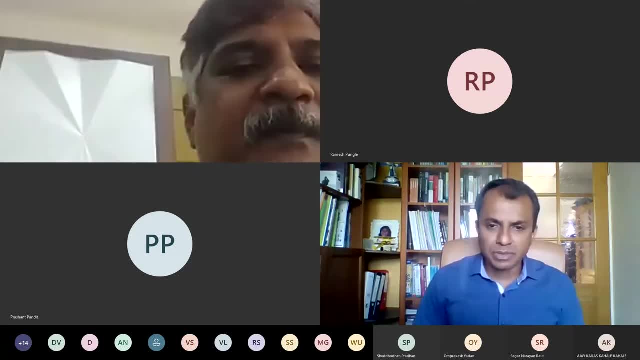 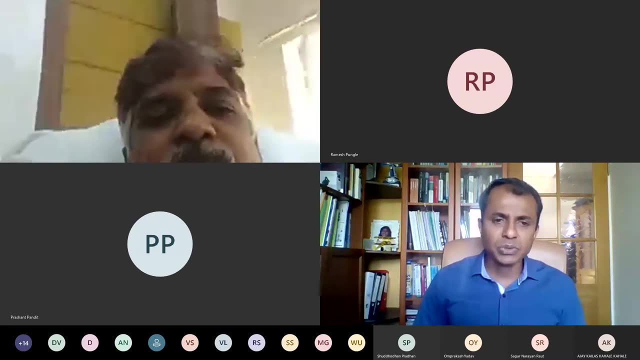 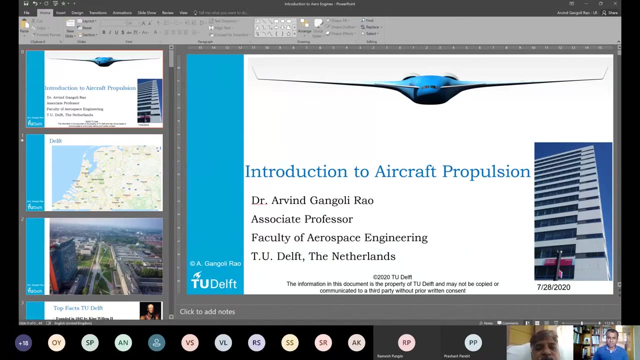 also gives us kind of opportunity, and that's and that's how we can connect now. So what I'm going to do today is present to you the fundamentals of a very short introductory lecture on fundamentals of aircraft propulsion. okay, Can you see my? can you see the slides? Yes sir, yes sir, we can see. Okay, let me see if this 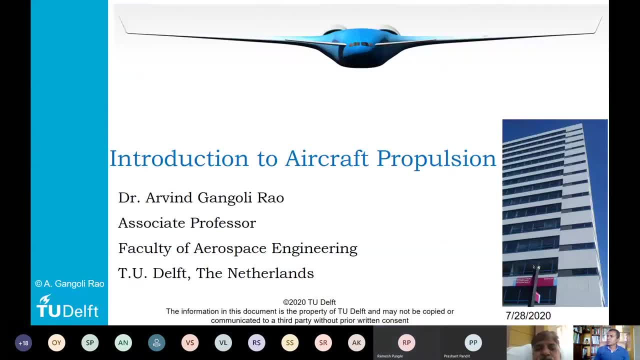 works. What about now? Yes, sir, we can see. Yes, sir, it's visible. Okay, great, okay. so what I would suggest is that, in case, if you have any questions, what you could do is, of course, I will take questions at the end, but, in case, if you want, if you, 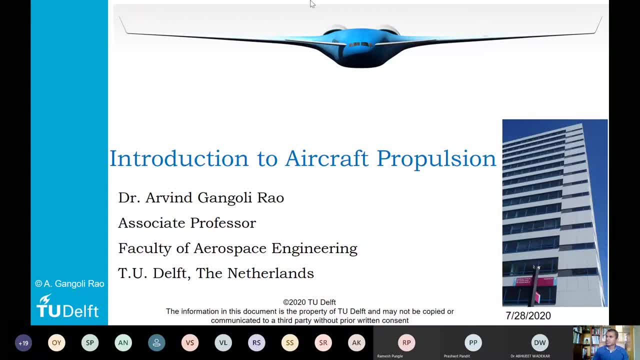 have any questions in between, you can always write your questions in the chat box and I will try to answer as I go, okay, So don't hesitate to ask questions. don't be shy. that is nothing like stupid question. you know, all questions are important and, as you, as Professor Variga was saying, I was from the first batch of 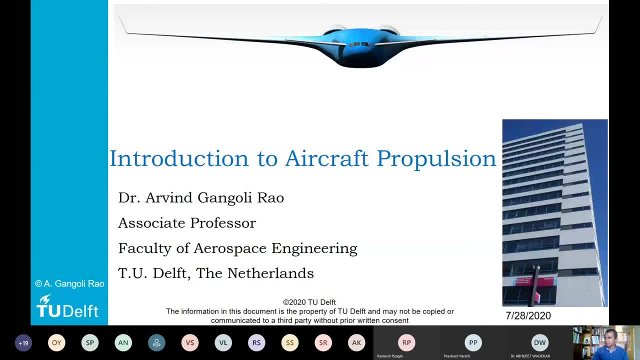 PES, and so this is. I've completed almost more than 20 years since we graduated. okay, and it's good to see you, Thank you. So let's get back to the topic we are already behind sharing. so, before I go to the the crux of the lecture, I would like to give a very short introduction to TU. 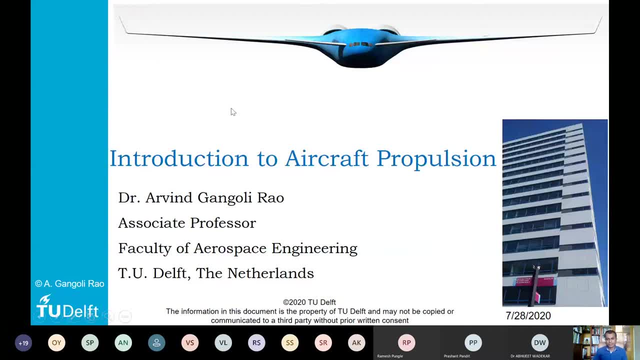 Delft, the Institute that I am working on in for last 12 years. so TU Delft is located in the Netherlands. Netherlands is a quite a small country, actually in the north of you, and this is the the map of Europe, and you see that here is. 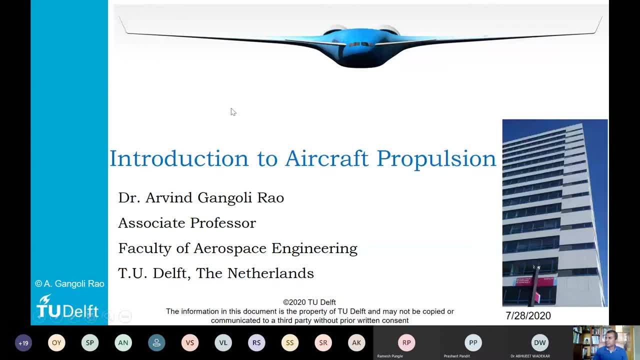 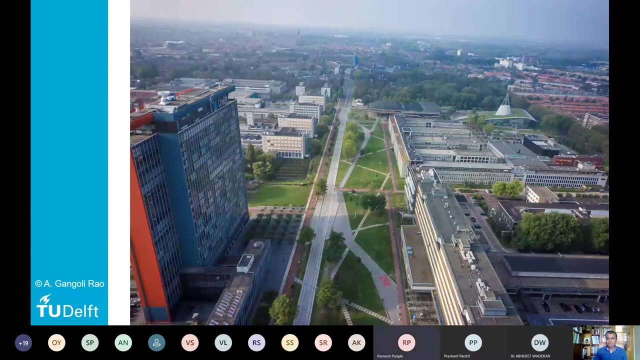 Netherlands, and Delft is a small town which is located between two big cities, so The Hague and Rotterdam, and that is quite an old town. it has a history of approximately 1200 years old. okay, and this is the view of the campus. this is the north side of our campus and what you see, this is our library. this is the 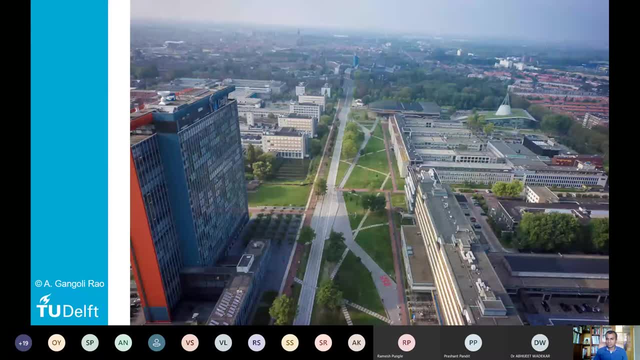 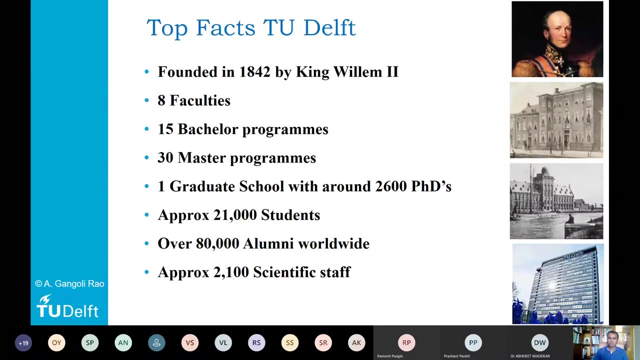 building this- mechanical engineering, electrical engineering, civil engineering and so on- and we aerospace is located on the south side of campus, which is not visible in this picture, so this is a view of our campus. um, just to give you some brief data or, let's say, information about 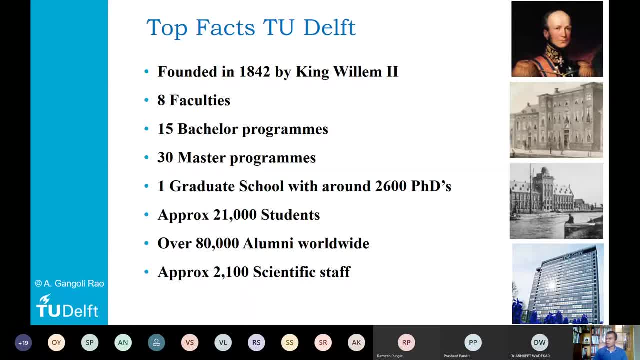 TU Delft. it's quite an old university. um was founded in 1940- 1842, sorry- by king William the second of the Netherlands. uh, at the moment, uh, we have uh what in India we call as departments, here we call as faculties. so there are uh eight faculties, which is like eight big, big departments. 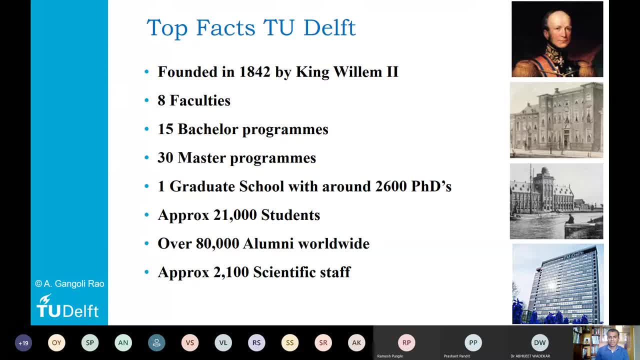 with approximately around 15 bachelor programs and 30 master programs, and the total number of PhD candidates in the university is about 600 and in total we have students on the campus with around 80 000 alumni is worldwide and the total scientific staff or the faculty members is approximately around 2000.. so it's quite a big technical university. 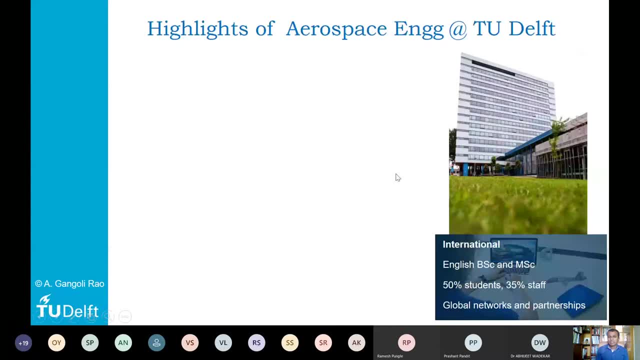 it's the biggest in the Netherlands and just to give you some highlights from aerospace engineering, so our department of aerospace was started in 1940, so actually during the second world war, um and um. we have approximately 1500 students in the bachelor program and approximately around 300 students in the master's program. okay, so by far we are the biggest. 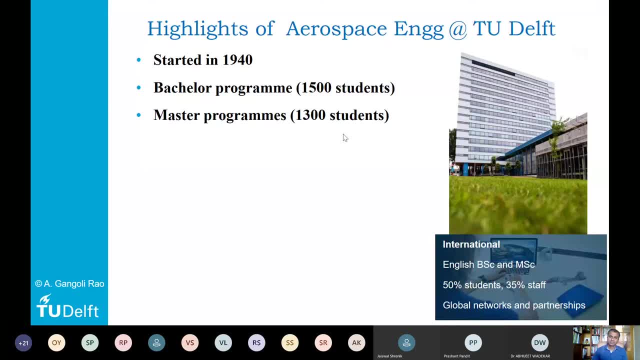 faculty of aerospace in the in the western world. okay, of course, apart from classroom teaching, we already have quite a good presence on online education, and that came very handy during the corona crisis, because we could shift the curriculum and we could do a lot of things in the classroom. 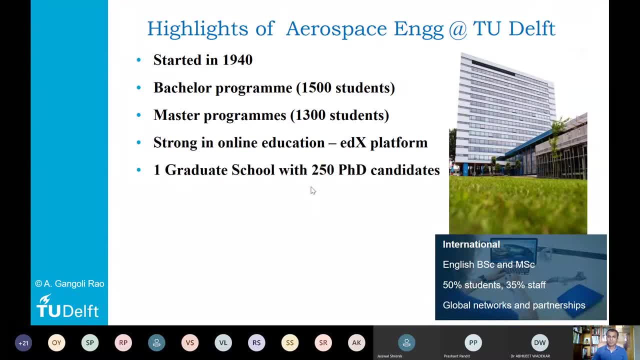 teaching. we already have quite a good presence on online education and that came very handy during the corona crisis because we could shift many of the things on online platforms very easily. we have approximately around 250 PhD candidates in our in our department and around 130 faculty members. okay, we are ranked fifth in the world. 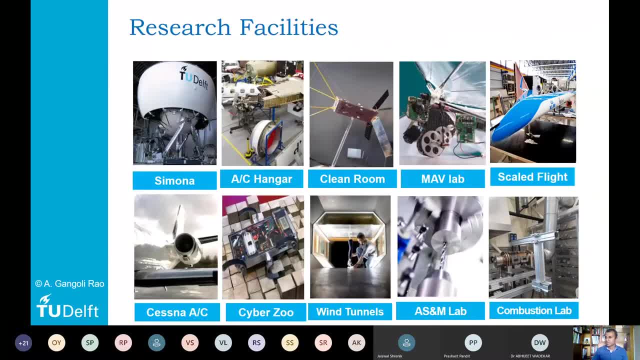 this year, yeah, and these are some of our facilities. so we do have a flight simulator. we do have, uh well, um has a very good history, uh, in terms of designing aircraft, so so we still have some of the aircraft that was designed. we have a clean room. 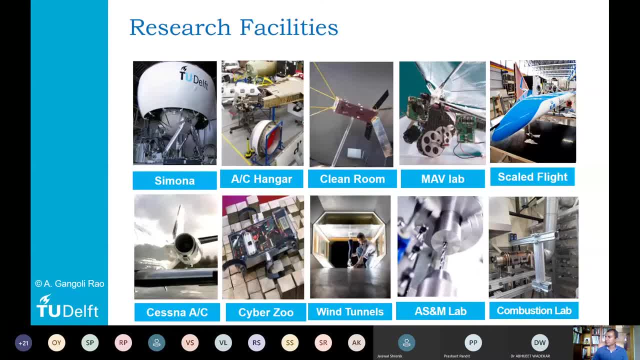 and this clean room is used to make satellites. we have currently two satellites orbiting around the world that were made here in delft. we also have a micro aerial vehicle lab and the vehicle lab is quite famous. uh recently got one million award from Lockheed Martin for a competition. 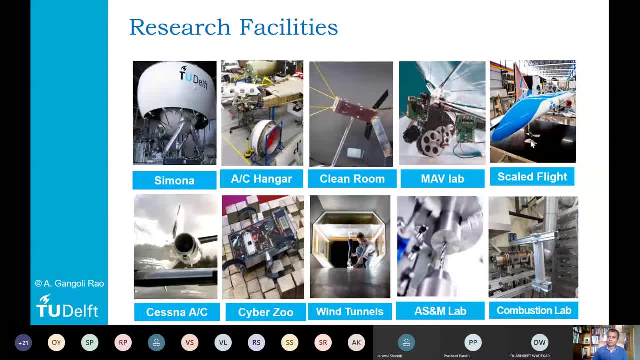 We have a scale flight lab where we do small scale flights to actually test them. We also have an aircraft, Cessna Citation, which we use for teaching as well as for research. We do have wind tunnels, a large number of them, actually 11 wind tunnels, so wind tunnels where? 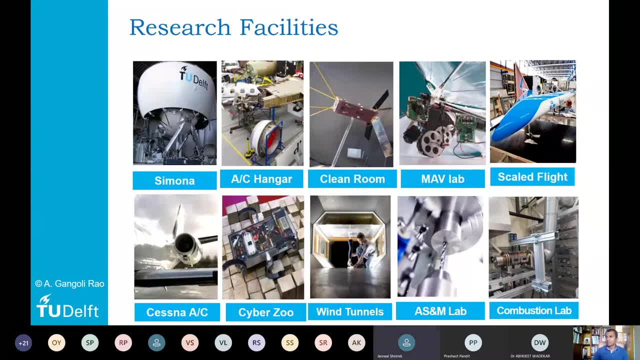 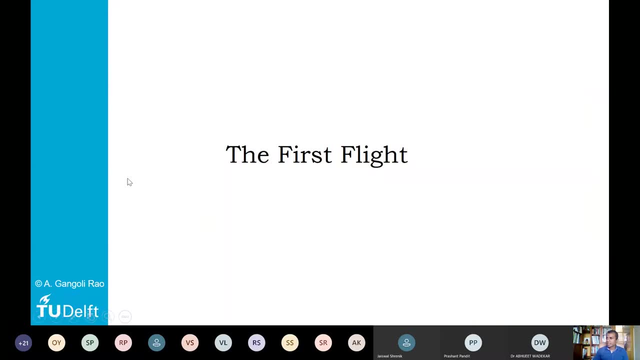 we can. we have flow speed from 30 meters per second to all the way to 8 kilometers per second, so hypersonic velocities. Of course, we have manufacturing lab and also a combustion lab where I am more active. Okay, so let's go to the topic and let's talk about the first plant. 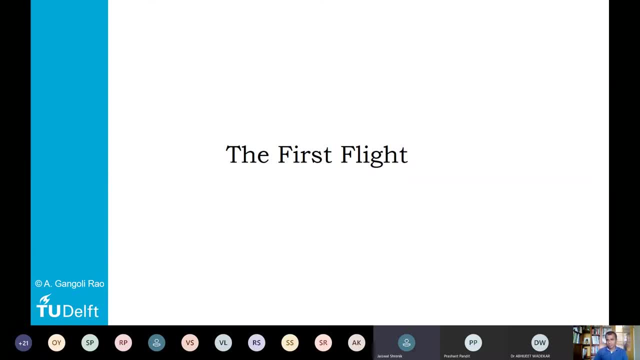 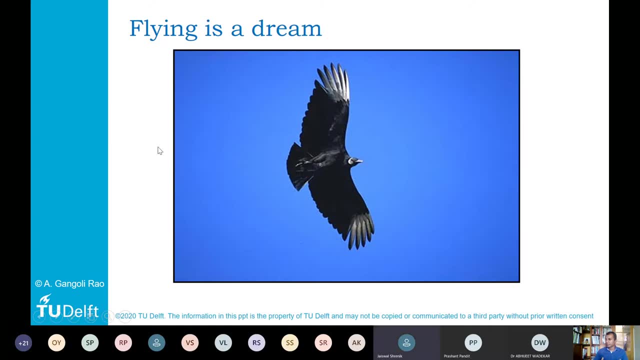 Okay, again, if you have any questions, please do not hesitate to put it in the chat box. So the first flight, you know, I mean flying is always has been a dream, you know, and whenever we see birds you think wow, I mean, they can fly, and can we do that as well? fine, I mean, I would like to. 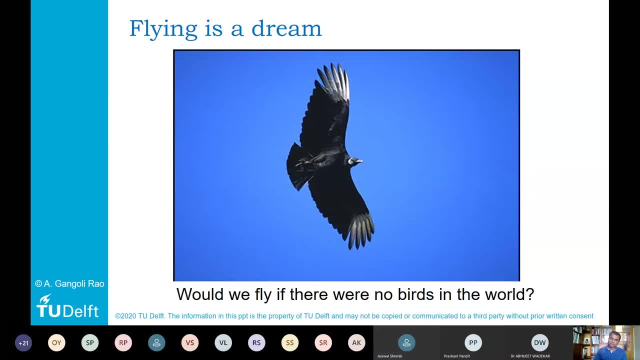 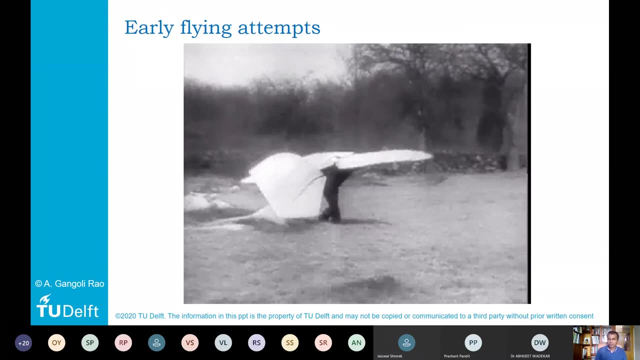 ask you a question you don't have to answer now, but think for yourself. and would we fly if there were no birds in the world? that's, of course, a kind of philosophical question, but think about it okay Now, when you look in terms of the early attempts of flying, of course, 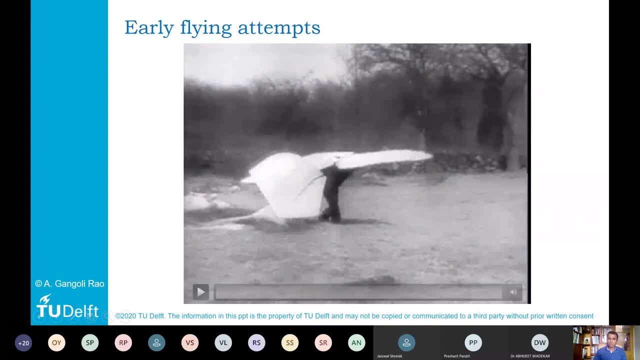 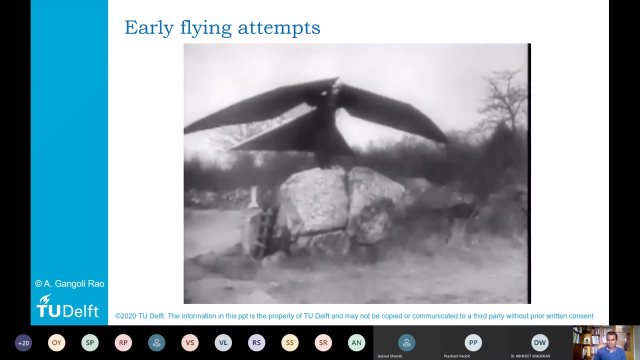 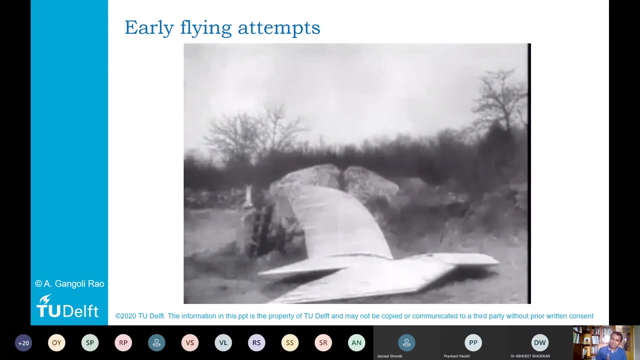 you know, people thought the best way to fly is to imitate birds, and there are some videos that I'm going to show you and that's how sort of people try to fly. Okay, so, yeah, okay, and so this happened. Well, in this case, of course, you know, the person is just jumping off a rock, But 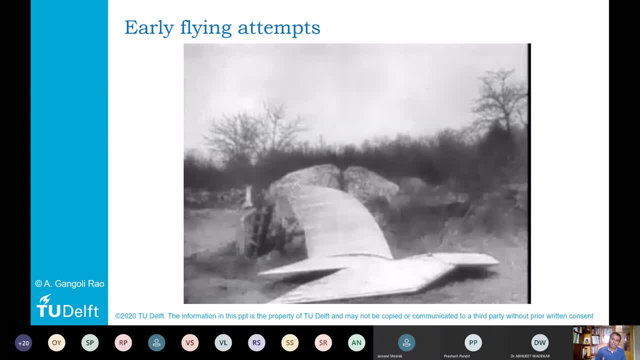 in many cases they they jumped off from cliffs and many people actually ended up losing their lives. now, of course, very soon, we understood that our systems of muscles is not capable to generally to generate enough power to provide a lift. yeah, and so the idea of having a machine to do that. 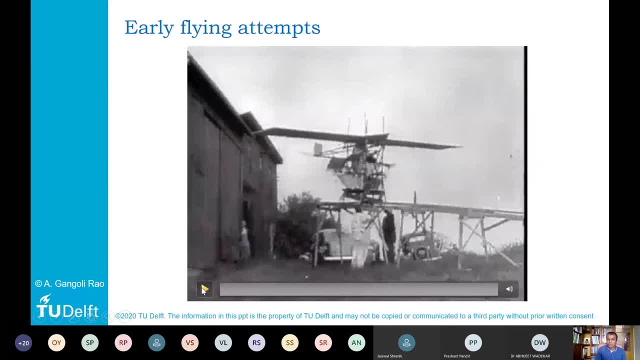 came early on, yeah. so there are some other examples, okay. so here you already see a kind of a machine where there is some kind of a wing, yeah, and there is some kind of a propulsion system, not very elegant, but nevertheless, you know, these were the early days of aviation, and 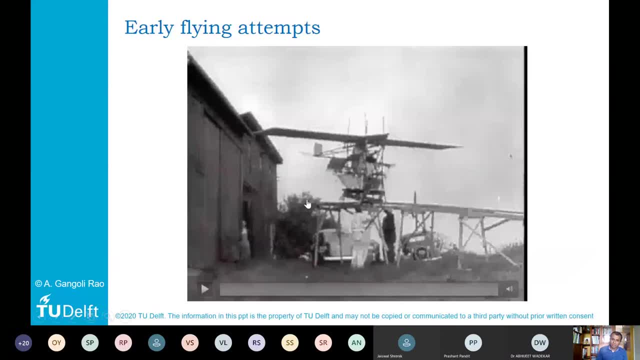 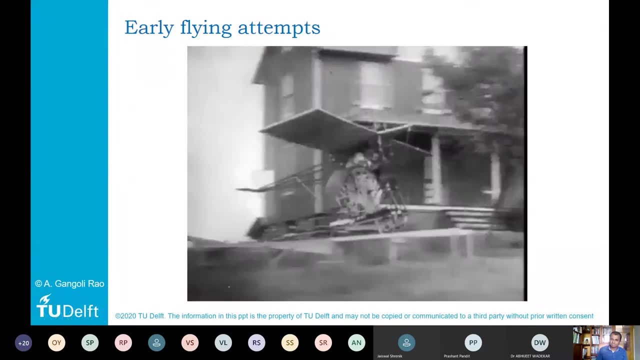 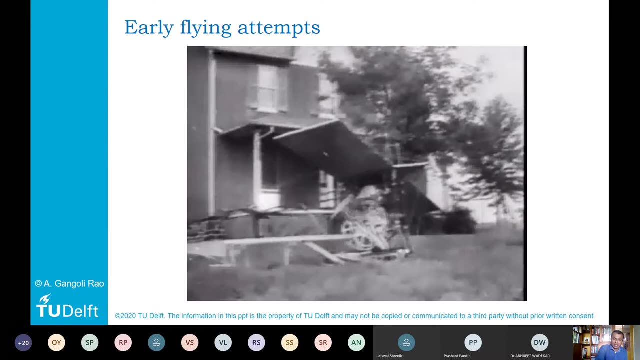 people were trying all kinds of things. yeah, um, so let's go here and see you know. yeah, so you see that a large number of attempts were actually carried out and not many of them were successful. okay, but over a period of time, of course, the thinking evolved. 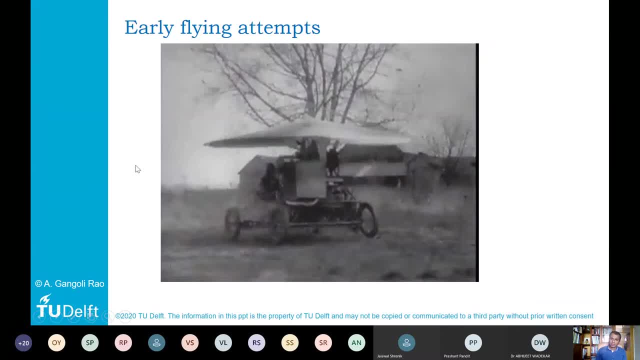 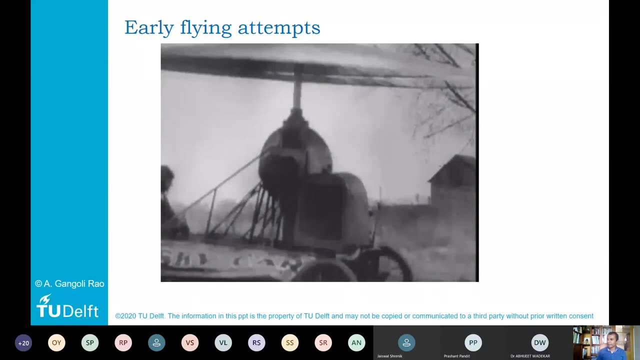 and people learned from their mistakes. and well, there were some other phagy ideas as well, like, for example: so the name of this machine was sky car, but it did not take off from the ground. so so again, there were many, many more attempts. now one of the first persons to actually sort of formalize this. 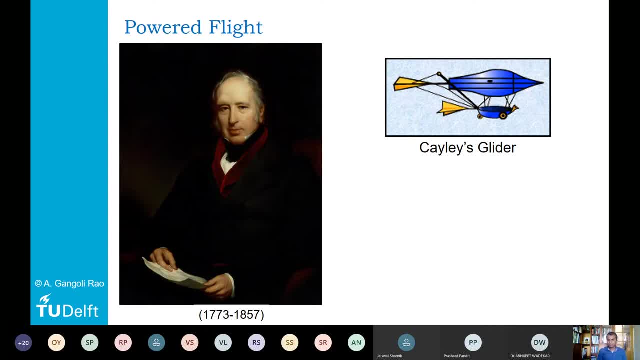 discipline, in a sense, was sir george kalen, and so he was one of the first ones to actually apply scientific methods to study flight, to study the lift that is produced, and so on and so on, and he has he's sort of considered the father of aviation, in a sense, and one of the 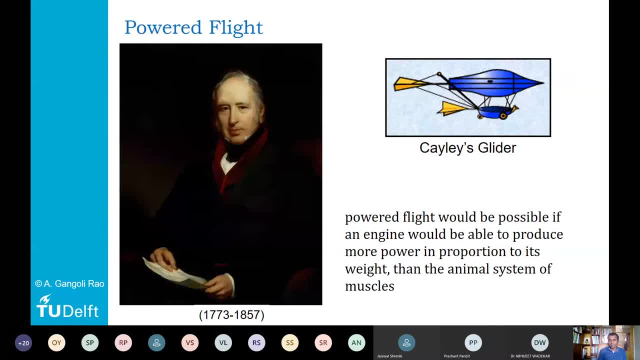 more important things that he sort of pointed out is that power flying would be possible if an engine would be able to produce more power in proportion to its weight. yeah, so, so he, he coined this term that we now refer to as power to weight ratio, and that is very, very critical. so he 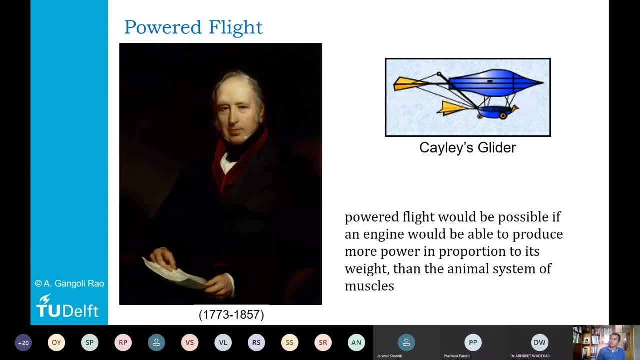 understood the importance of weight and the importance of power, and he also understood that if you want to take off from the ground, then you have to produce a lot of power without being too much. yeah, he was one of the first ones to formalize many of these concepts. 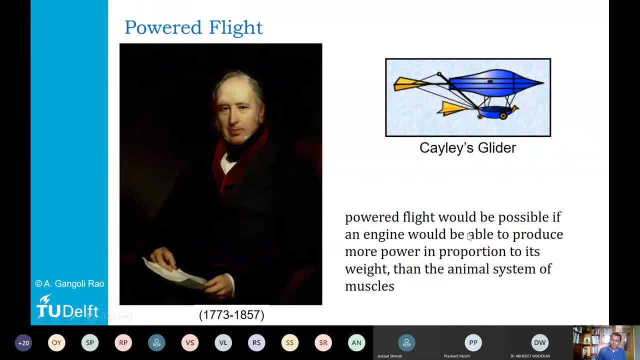 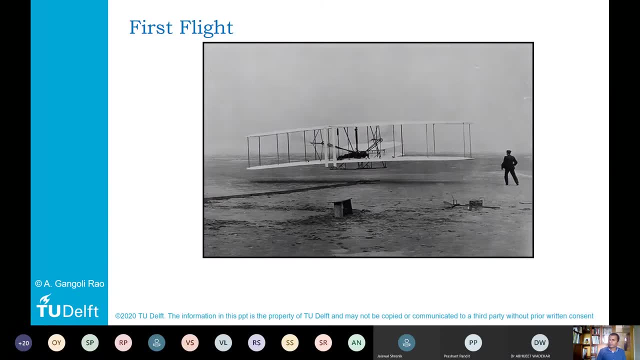 that we take for granted today. of course you know this picture, i think. yeah, this is from the first flight, yeah, from 1903, from the wright brothers. now, if you can use chat function, then could you sort of tell me what was special about this flight? we call it first flight. 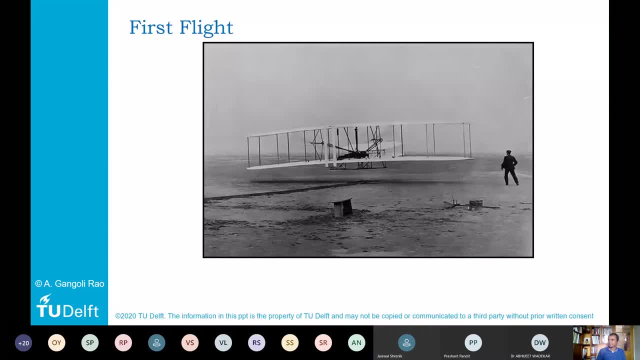 but what was first about anyone? okay. so the first thing about this flight was that it was a powered flight. yeah, it was heavier than air front. yeah, it was controlled flight. okay. so, for example, hot air balloons existed, were existing before this, but they were not heavier than air. hotter balloon is created because, 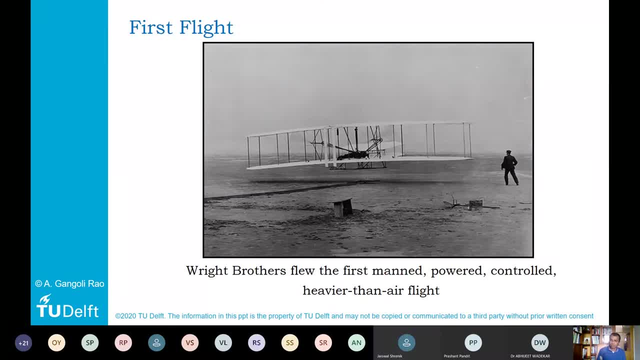 that hot air has lower density and it creates its own lift. okay, so it's lighter than air and, of course, hot air balloons cannot be controlled, so you are always at the mercy of the winds and you go well in state. okay, so this was the first man power control and 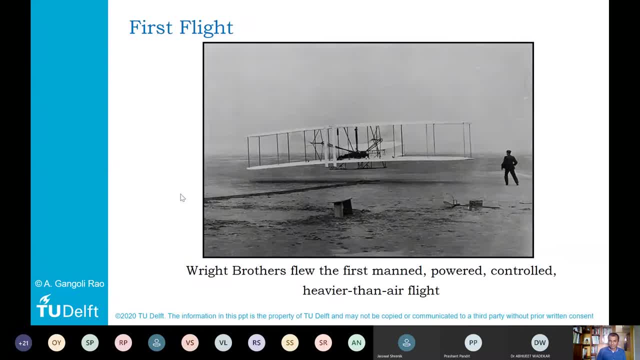 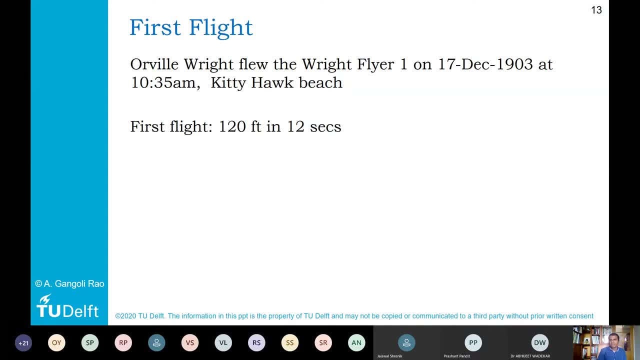 heavier than air flight? yeah, and that's why this is called as the first flight. so when you look at this first flight, which happened in 1903, 17th of December, in Kitty Hawk Beach in Ohio, and what you see is that the first flight was, 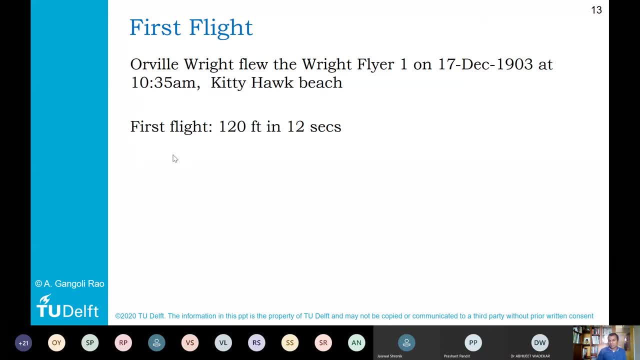 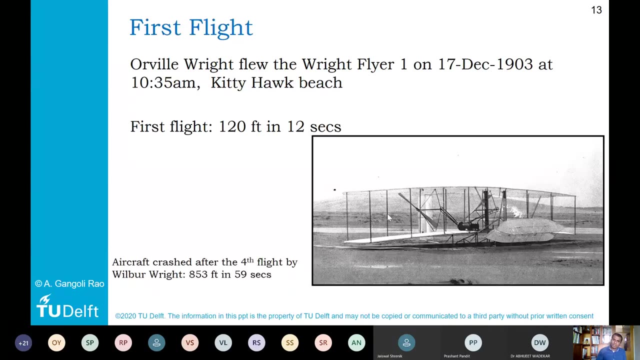 actually not much. um, it was only 120 feet and lasted 12 seconds. I mean, this is, this is actually less as compared to the wingspan of a boeing 747, you know so. so in terms of span it was not much, but it still created history at that point. 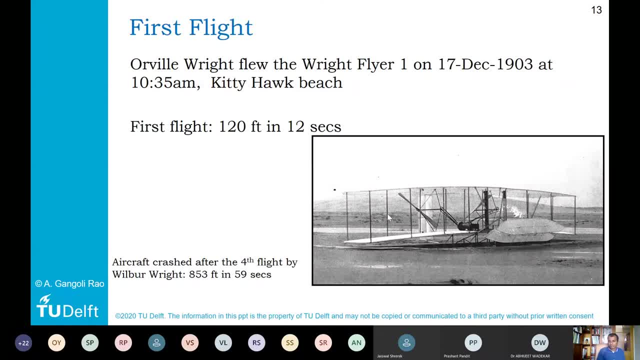 and of course they had several more tests on that day and in the last flight on that day they also crashed. but you already see that they achieved quite a remarkable success. distance actually more than 800 feet and almost flying for a minute- yeah, so you already see that there are quite some improvements. now let's see how did. 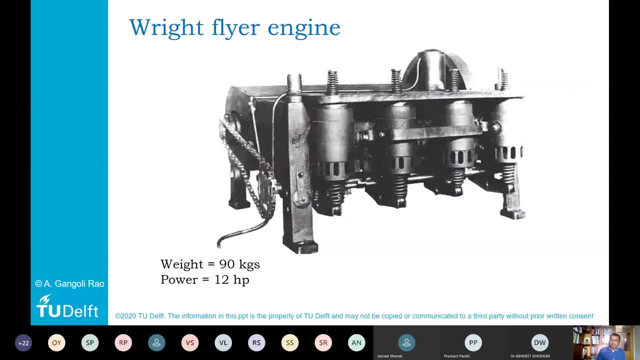 things evolve as we went along, okay. so one of the main things that that was key for for Wright Brothers- apart from the fact that they had to design this biplane and they had to also design the, their own propellers and so on- but one of the key things that enabled them to do- 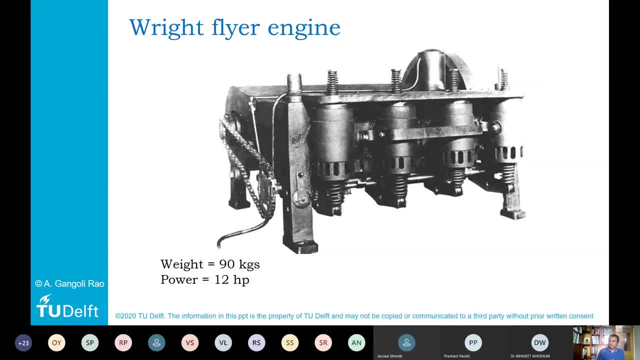 this is actually the IC engine, right? so IC engine was the best power to weight ratio available at that time. I mean, if you look at this, this engine which is, which, from today's standards, is quite rudimentary, but it weighed around 90 kilograms and produced around 12 horsepower. now, 12 horsepower is not much. 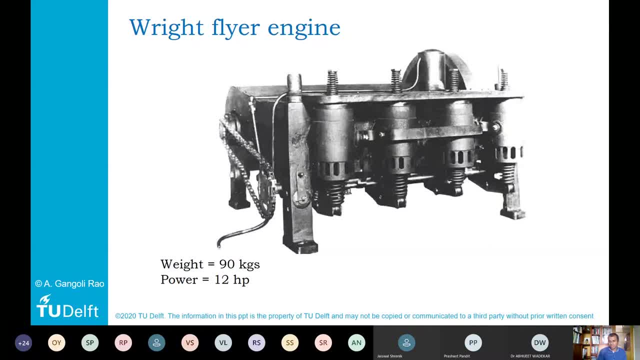 right. I mean most of you use, use- I am I'm sure you must be using bikes or something, or cars, and then they have much more power than this. okay, but for that time this was quite a state of the art, and remember that this was still an uncooled engine, so they could not use this engine for a long. 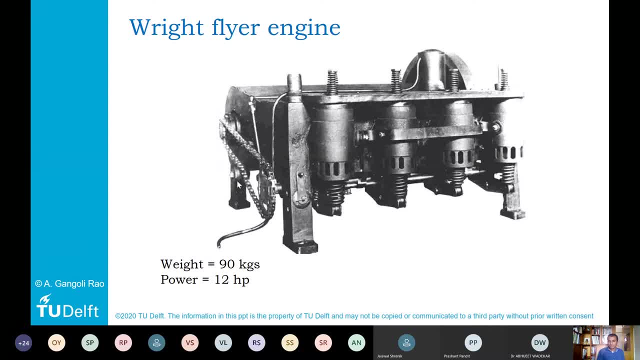 time now. so the propulsion system was sort of one of the key factors in enabling them to provide enough power without having to weigh a lot. and before this actually, there were also other attempts by other people where they try to use something like a steam engine, but steam engine was extremely heavy. so you see that the progress in science. 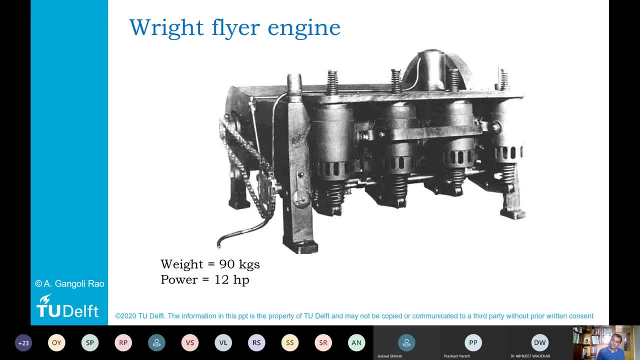 always happens over a period of time and a large number of people are involved, and that's why it is important that, in the scientific community, you always share your understanding, because, yeah, people don't have to repeat the mistakes that someone else has done, and that's why we have all these journal papers. 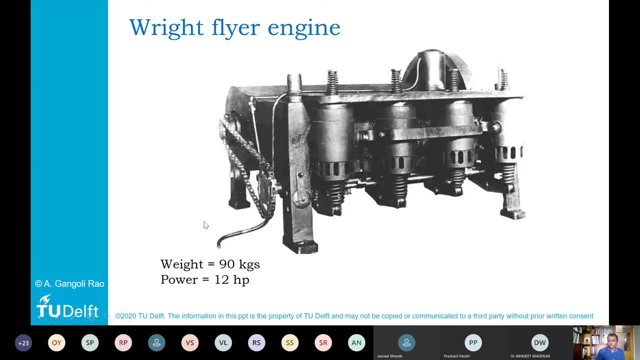 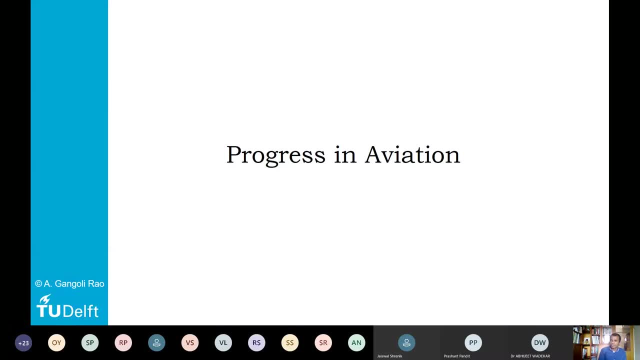 where we sort of disseminate our knowledge. so let's take a kind of a change the gear. so we talked about the first flight, so that was approximately 117 years back, and let's, let's, let's look at how things have progressed. and when you look at aviation, the progress was really in the 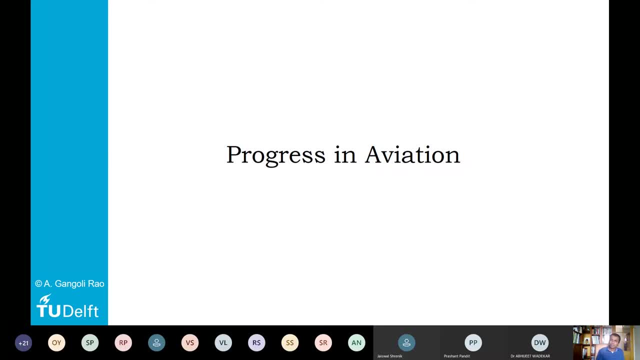 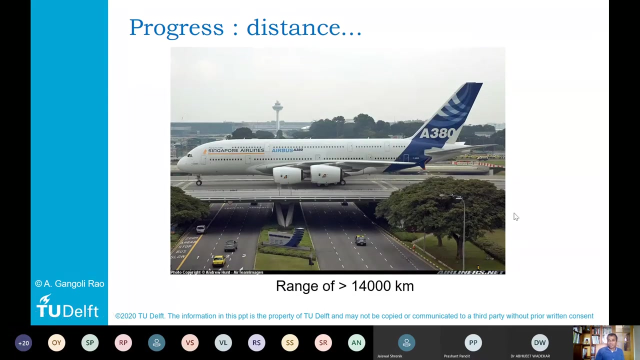 early years was was fantastic. I mean after Second World War, that was a huge, huge change in civil aviation. so in terms of distance, you saw that the first flight was only 853 feet and in. so today you would take a super jumbo like A380, a beautiful aircraft, Airbus stopped. 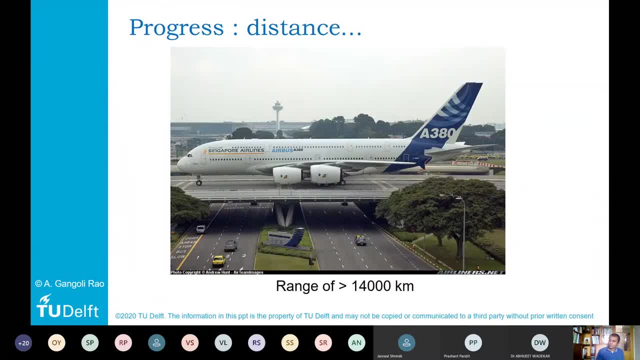 producing this, but I think this is a very elegant aircraft: huge, 550 tons take-off weight and in a single class seating capacity it can go up to almost 800 passengers, so you can take 800 passengers all the way to around 14-15 thousand kilometers. 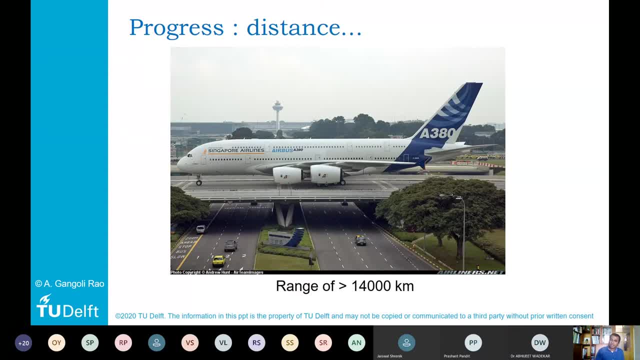 So that's the kind of the distance that an aircraft can cover today. in fact, the the next generation of 777X and also A350 long-range, A350 thousand, they can go almost around 18,000 kilometers or so. yeah, so. so it shows you how much what. 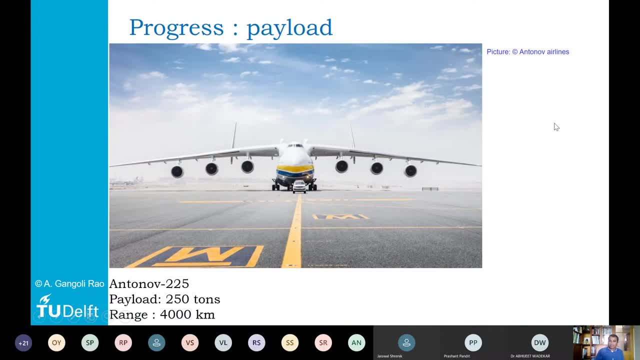 has been the progress made In terms of payload. well, the first flight could carry only a Wilbur Wright as a payload- yeah, one person. but then you see this huge monster that is called as Antenna 225. it's a fantastic and beautiful aircraft. it has a payload of. 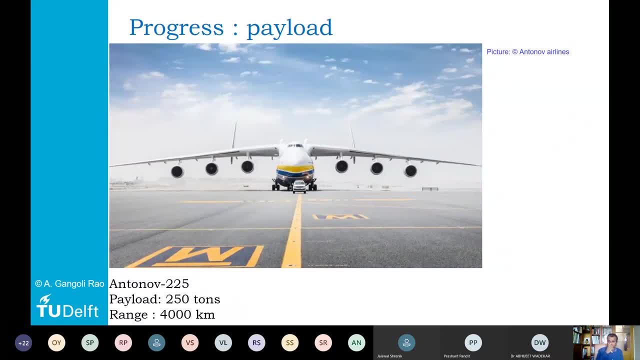 250 tons. yeah, it is. it was designed for the Russian space program, but it has been used all over the places for all kinds of things and it's it's still one of the most reliable ways to transfer any heavy material in a short period of time, and 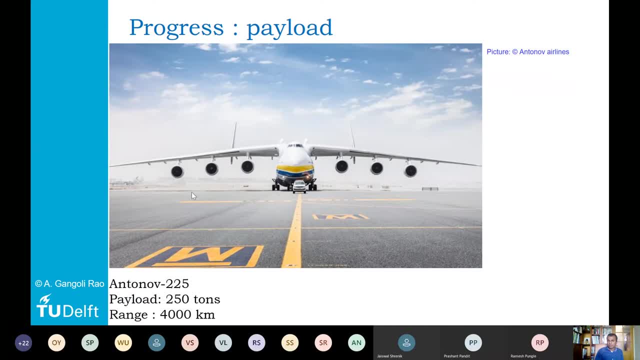 now, and and you see, of course, this huge turbofan engines- six of them, yeah, but one of the interesting features that I find, apart from the engines and the aircraft. of course, every feature of this aircraft is beautiful, but one of the most intriguing feature of this aircraft, which I find, yeah. so when you look at 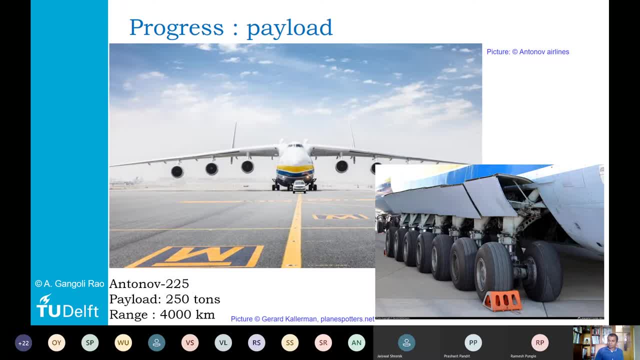 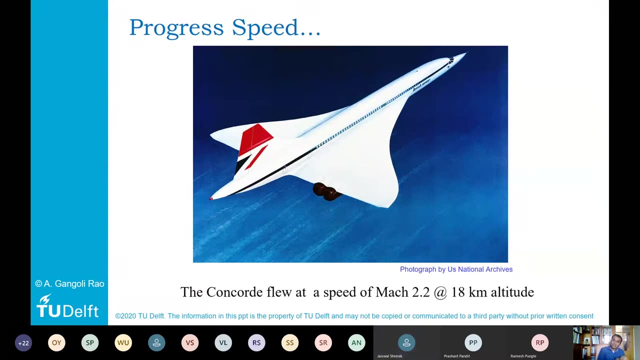 this landing gear. I mean it's, it's huge. it's sort of mind-boggling to see there are some so many landing gears for such an aircraft. okay, in terms of speed. so in terms of speed, of course, you see that Wright brothers the first flight was something like 20 feet per second, or. 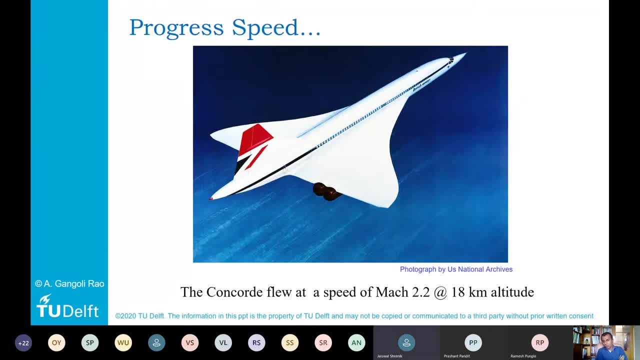 something in that order, whereas of course that was Concorde aircraft, which unfortunately does not fly anymore. but Concorde already broke the speed for civil aviation. it was flying at a Mach 2.2. that means 2.2 times the speed of sound, at around 18 kilometers altitude. so in fact you could. 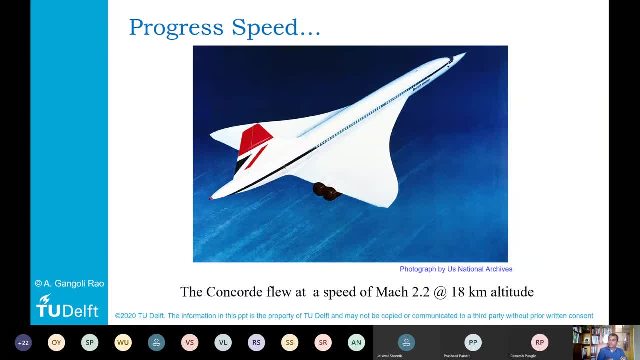 take off from Paris and you could land in New York. and if you take off from Paris at, so let's say, 8 o'clock in the morning, you would, you would land in New York before it becomes 8 in the morning in New York. so you could sort of you. 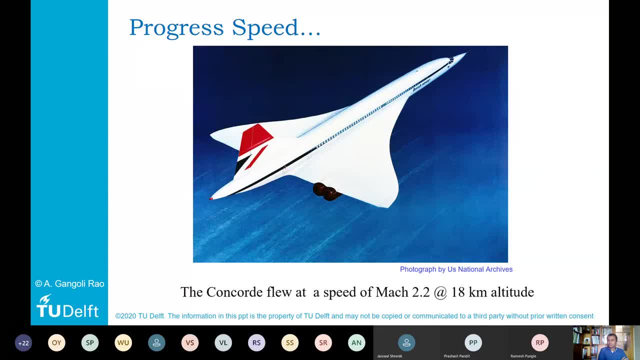 know, cheat the time a bit in a sense. yeah, so so that was a fantastic aircraft, but unfortunately commercially not successful. yeah, and that's well. there are several reasons for it, but one of the main thing is that, of course, when you fly supersonic, the amount of fuel consumption is extremely. 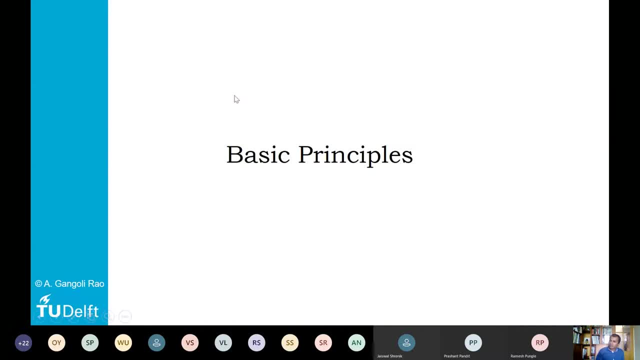 hard and, of course, there are environmental problems and well, as noise problems. okay, so now we have looked at the progress that has been made, so let's look at some of the basic principles of propulsion. yeah, so I'm starting at a very, very basic level. so you know how do you propel, so you know, one way is to take a balloon. we 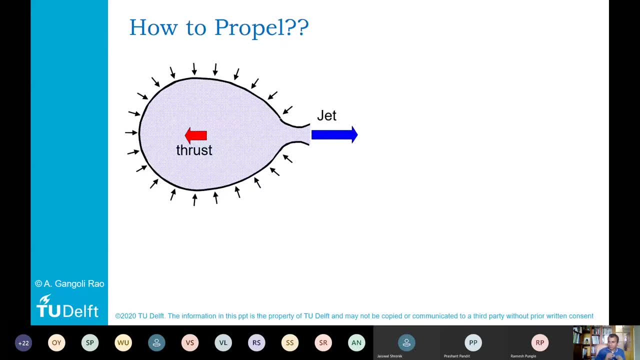 have all done this. we have played as, as children, where we took a balloon, we sort of, you know, blew it, blew air in it, and then we let it go, and then it just goes randomly everywhere, okay, and that's what happens, right. so so, but when you think, 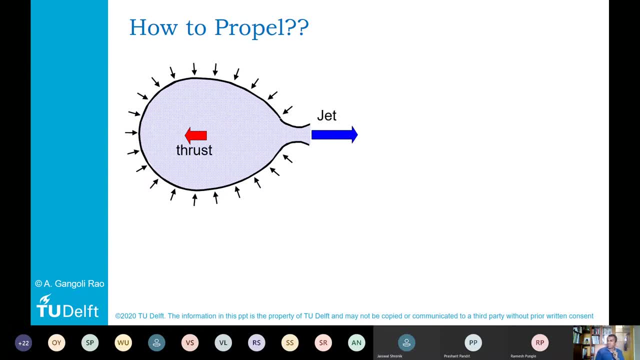 of it. that is a propulsion principle here. so the pressure inside the balloon is high, the pressure outside in the atmosphere is lower than what is inside and because of the pressure difference, the pressure inside the balloon is higher than what is inside and because of the pressure difference, 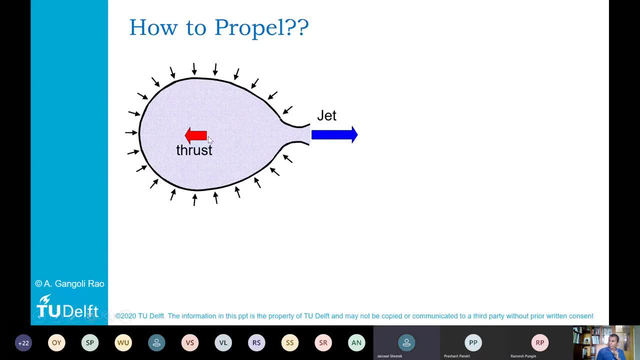 the air actually comes out. okay, and when, as it comes out, it's, it accelerates, right, and so that means that this jet velocity is high, okay, so there is a change in the momentum of the air- the momentum of the air which was inside, as compared to this, and this change of momentum produces force, and that was 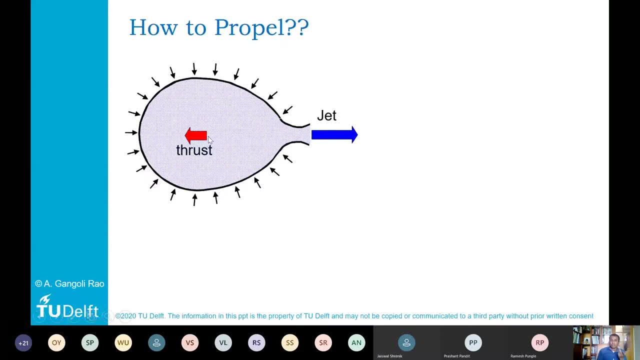 Newton's second law of motion, right, and because every force has an equal and opposite reaction. so you get the thrust, okay, so so you. so from a principal point of view, it is pretty easy, okay. the other toy that we- most of us, we- have used as kids is this kind of this: 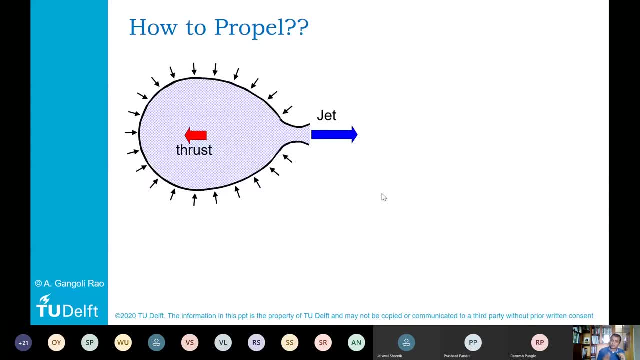 Chinese propeller where you know, you just rotate it and it just goes around, yeah, and it goes up. so so again, the principle is the same. you see that it cuts the air and it accelerates the air, it pushes the air down and that process it sort of creates an upward force, okay, so so this is the basic principle of 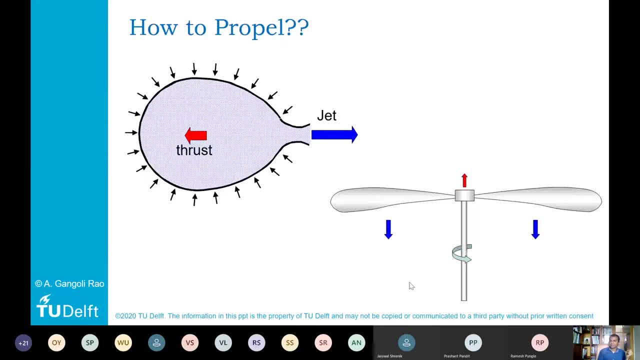 propulsion that you change the momentum of the fluid. okay, and in most of the cases it is air. for airtough, of course it is air. and for rockets it's because air rocket has to operate in environment where air is not available so it can use another fluid. okay. so that's where rocket has to carry the oxygen as well. 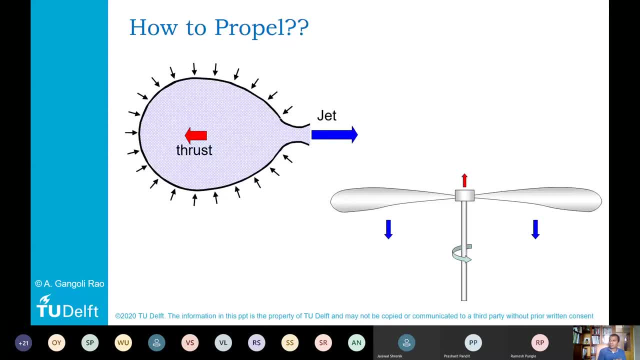 as the propellant? both, yeah, but as in an airtough, you don't have to do that. we always use the ambient air, so there is no way to change the air in this way. so this is another question. okay, so if this is the main principle of 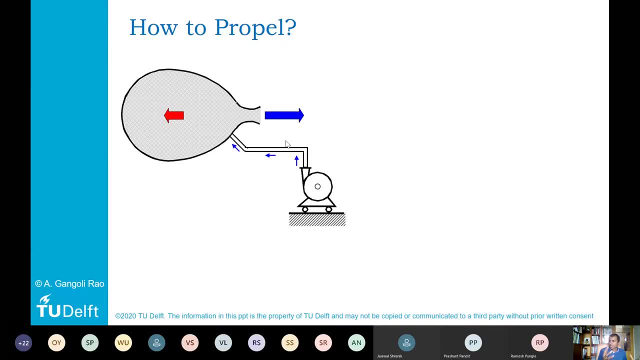 propulsion. let's say then, what can you do? so? so again, let's take this balloon as an example, right? I mean, of course, when you do a balloon, you know it will do only a few meters and that's it. but if you want to sustain this balloon for a 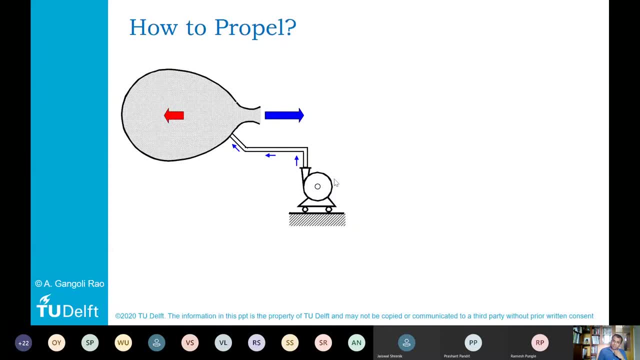 longer time, then maybe you have to connect it with kind of a compressed air. so that's the pipe, that this pipe is now sort of giving continual life, and then say that's how you do it. and the problem is how you do it again. you use the air and that's how you change the air. 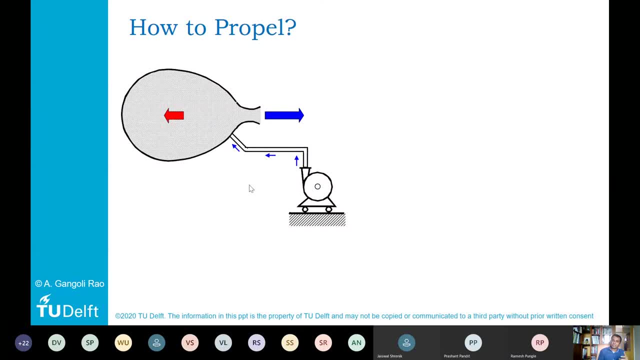 continuous pressurized air to this balloon and then it's coming out. yeah, and in that process then the you know the balloon you will hopefully will go a bit longer, but it's, it's not a smart thing to do, right? i mean, you always need some kind of a connection and so on, but okay, uh, you know one. 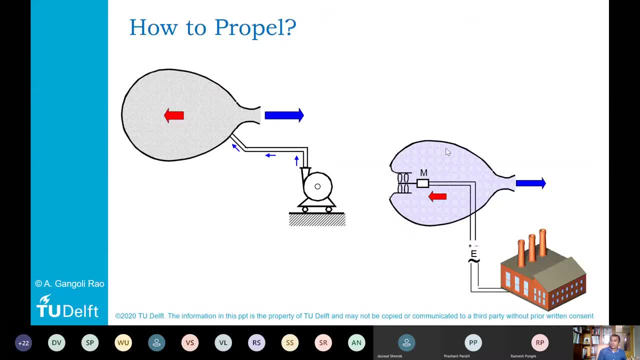 one slight improvement over this concept would be, if you sort of have a kind of a compressor in the balloon itself, yeah, theoretically, hypothetically, you can have it, a small compressor in the balloon, and then that's compressor is rotated by a motor and this motor is then given by electricity. well, if you don't want this electrical wire and so on, you 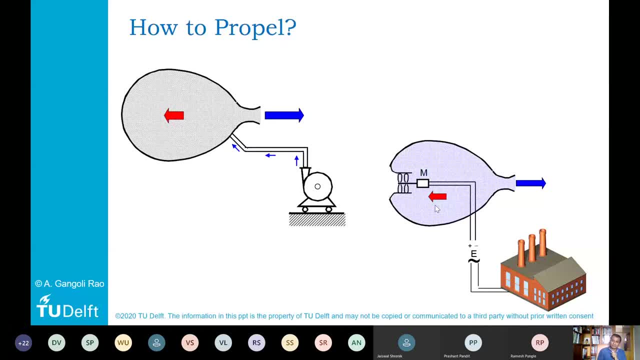 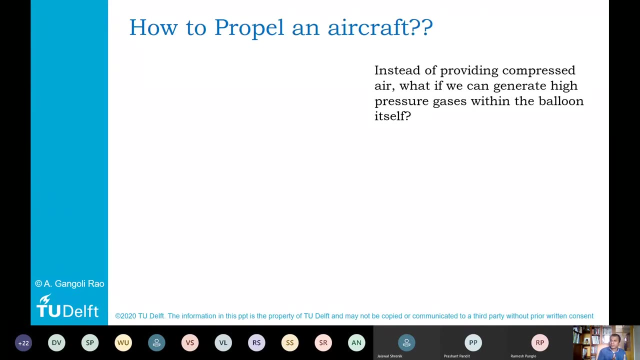 can have some kind of batteries, okay, so, so that's also can be done now, uh, but you know again, uh, the energy that you can carry in the battery or so on is is limited, so so other thing that is actually you can do is, instead of providing a compressed air, yeah, uh, what if we can? 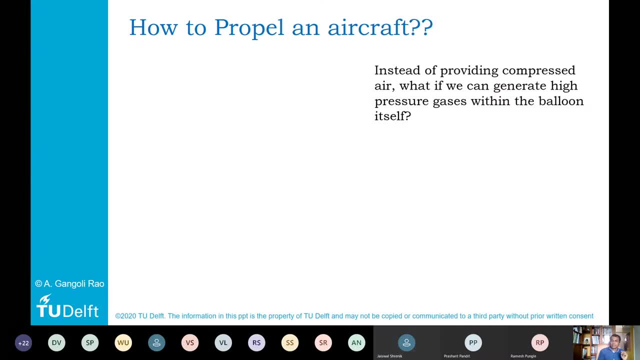 generate this high pressure gas itself. okay, and we can do that by having multiple stages of compressor. now, you can, you can pressurize the air, but how is the compressor driven? the compressor is actually driven by a turbine here. what you see in red now, of course, uh, but this, this cannot. 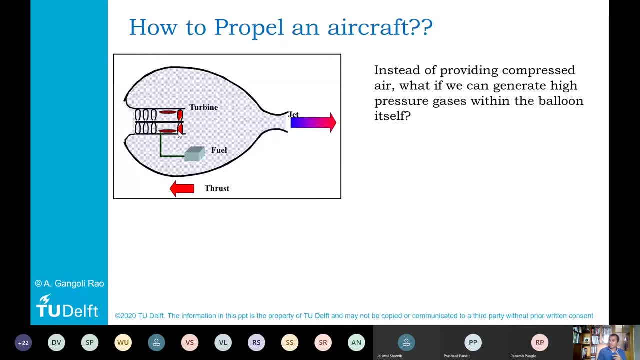 happen in a perpetual way, right? because, um, the power that is produced by turbine is not equal to that of the compressor if you do not add additional energy into it. okay, so? so, in order to sustain the process, you have to have additional energy input to this compressed air. 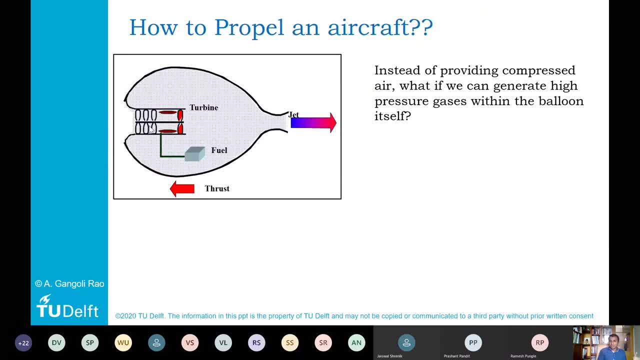 and that is done by a combustion chamber. so what is done is you have a compressor where the air goes in- yeah, it increases in pressure. you add fuel to this compressed air, you burn it. so at the end of the combustion chamber you not only have a high pressure air, but you also have a high pressure. 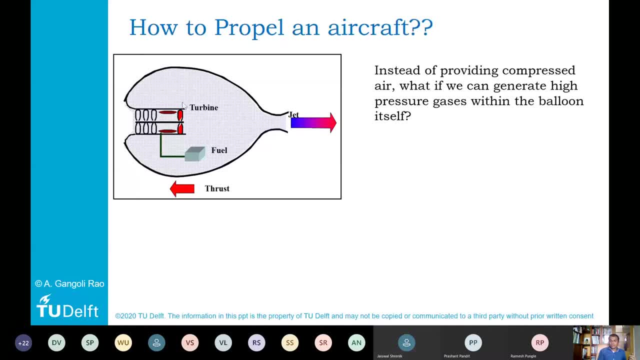 and high temperature air. now the turbine at the end of the compression chamber extracts power from this high pressure height of high temperature air. but even after the turbine has extracted the power required for running this compressor, that is still a part of the power left, and that part of the power which is left is then can be used for propulsion. okay, so this is in a very 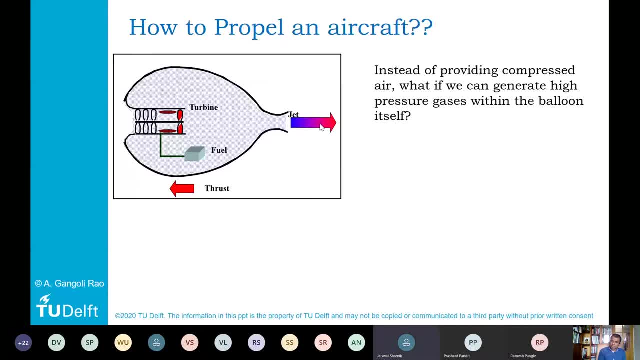 basic and schematic way. yeah, you can visualize this, okay, of course, you can do it in a different way, you can also add a propeller, and you can do it in a different way, you can also add a propeller, and so on. yeah, um, but nevertheless, this is sort of the basic principle of a jet engine, okay, so so, 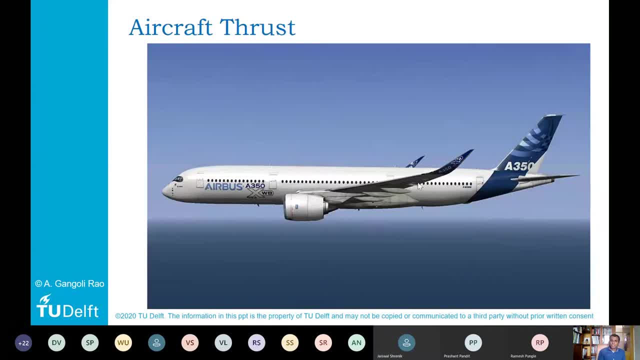 what you see in a beautiful aircraft like this airbus 850, okay, or any other aircraft. so what you see is that the engines are hanging in here, so they what they do is they take in this air and accelerates at a much higher velocity and in that process, of course, 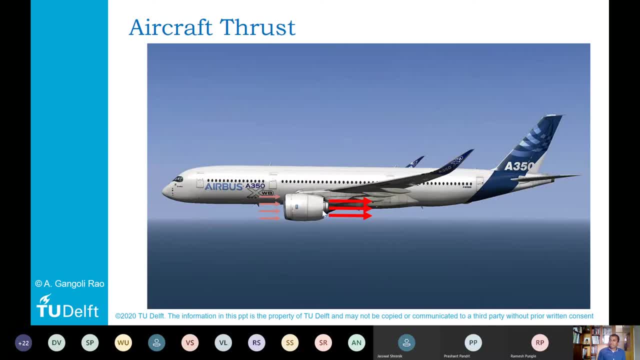 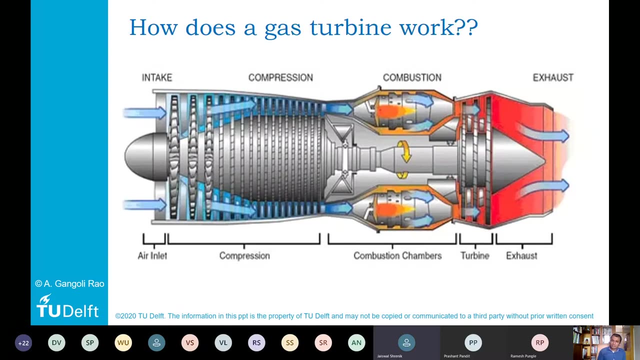 they change the momentum of the air and that's what creates force and thrust. okay, and inside this there is a fan, there is a compressor, there's a turbine, there's combustion chamber. so so these are the main elements, uh, that i showed you in the earlier picture. okay, so, if you look at an engine in a bit more detail, so this is how it works. so this is. 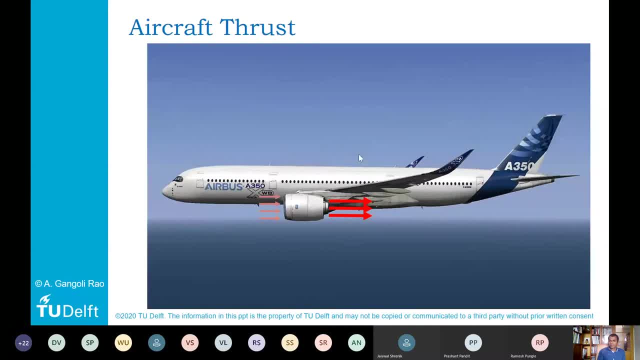 what is called as a turbojet engine. so most of the modern aircraft like this one, they use what is called as a turbofan engine. okay, so there are several differences between turbojet and turbofan, but in the in the view of time today, it's not possible to go into the details. okay, but 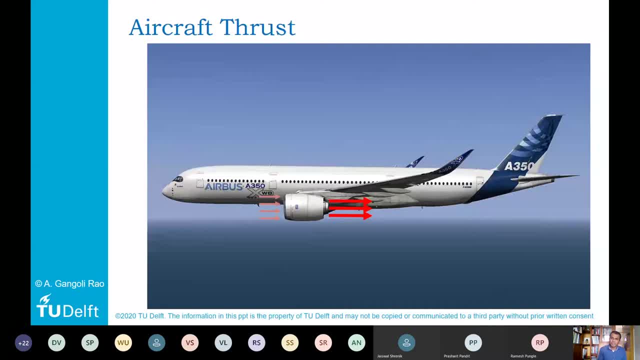 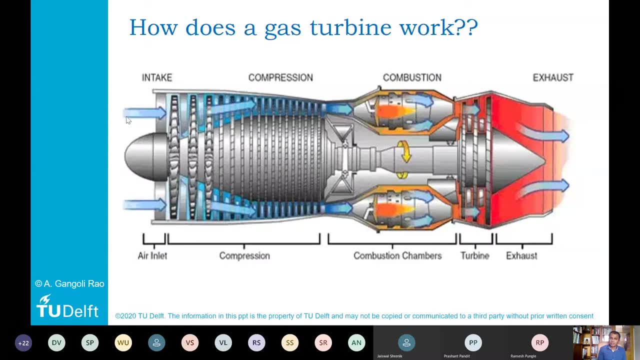 nevertheless, the basic principle is still that you change the momentum of the air. okay, so, in a turbojet engine, what you see is that there is this intake where air is coming, you have several stages of compressor and you can imagine these compressors as some sort of fan. okay so, with every state of 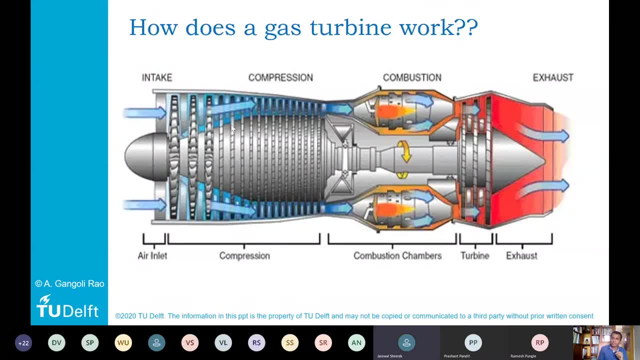 the air. you can see that the air is increasing and that's why the density increases and that's why you have to reduce the area. okay, so you see that the pressure would increase as you go downstream. yeah, at this point after the compressor, the air is at higher pressure, is at higher density. 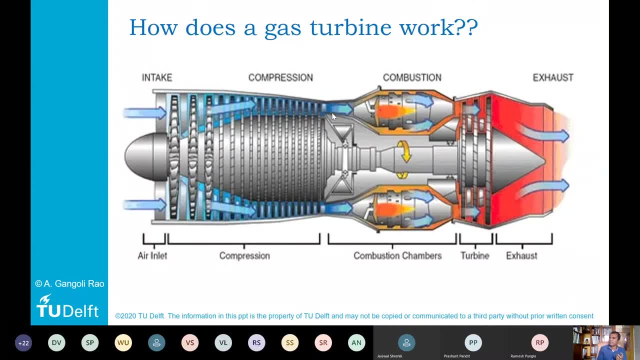 okay, and of course, because, uh, of the compression process, it is also at a higher temperature, okay, so what you can do is, after this compressor, you can see that the air is coming from the combustion chamber where we add fuel and burn. okay, so that's at the end of the compression, sorry, at the end of the combustion chamber we have. 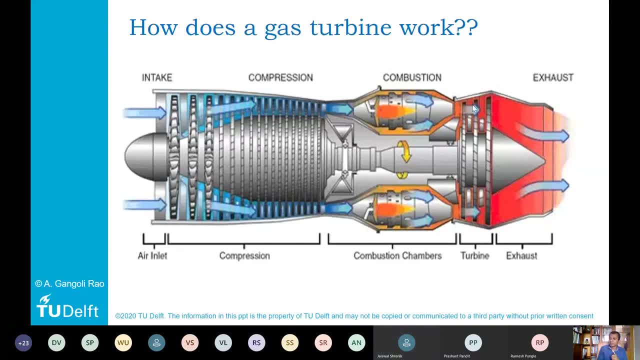 a high pressure and high temperature, and part of that energy in the gases is extracted by this set of turbines which drive these set of compressors, and the rest of the energy is what we can use for propulsion. okay, so you see, there are these five, six main components, and that is air inlet. 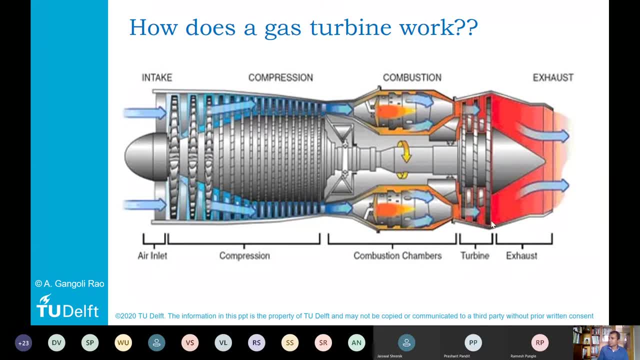 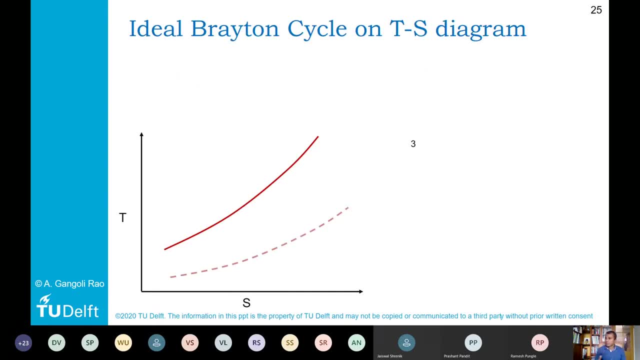 compressor, combustion chamber and exhaust. okay, so, so in in that sense it's not a very complicated process. okay, um, but at least for the mechanical engineering students, you must have learned about the ts diagrams, and they are very, very important actually. so even in my lectures, i mean, i use ts diagram all the time, and with just by using ts diagram, you can. 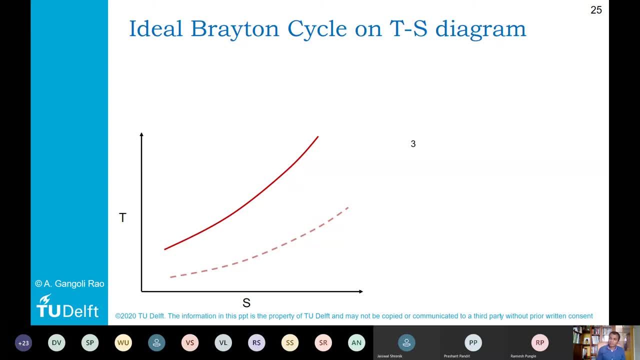 actually do a lot of calculations and you can also explain a lot of phenomena, okay. so of course, you, these are two isobaric lines on a ts diagram, yeah, and what you see is if you you have an inlet here, okay, uh, in the, in the inlet there is nothing much happening. so it's an, it's an isentropic. 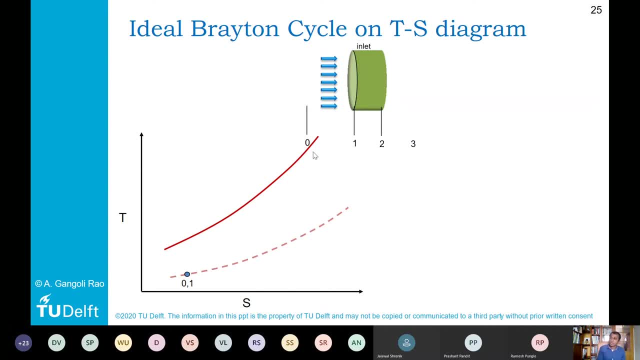 inlet, okay, so there's nothing much happening. uh, of course, in a cruise flight, if the total, uh, the static pressure would increase, okay, but the total pressure will not, yeah, so if we consider it as an ideal inlet, yeah, then more or less this would happen, and then you have a compressor, okay. 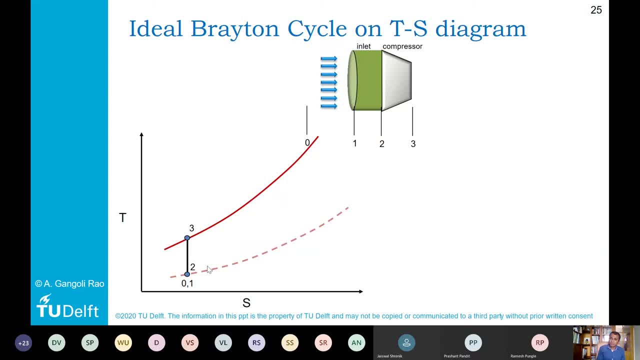 the compressor would increase the pressure as well as temperature. so you see that this, uh, the, the solid line is at a higher pressure and the dotted line is at a lower pressure. okay, assuming isentropic compression. in an ideal case, now your 0.3 would be here. okay, and of course then you would add fuel. 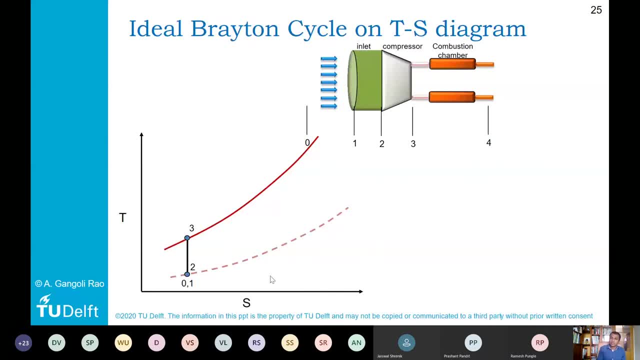 and the combustion chamber is a constant pressure combustion chamber, so that means that it would increase the, the temperature, uh, but the temp, but the pressure would remain the same. so it would go from uh, from on this isobaric line, yeah, upwards. of course the entropy would increase. so your 0.4, which 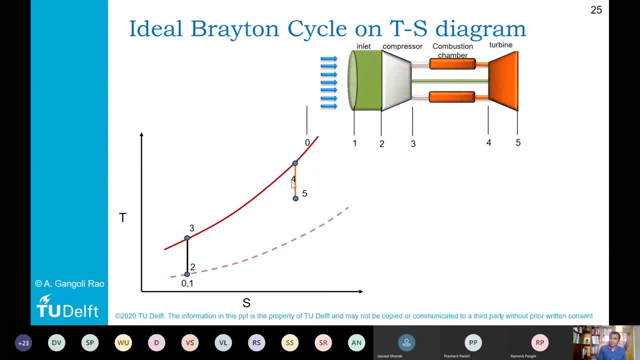 is at the end of the combustion chamber, is somewhere here, and then from four to five, you have an isotopic expansion. okay, so this, this line, should be equal to this line in an ideal case. okay, so that. so the turbine is driving the compass, the compressor and then the remaining power can. 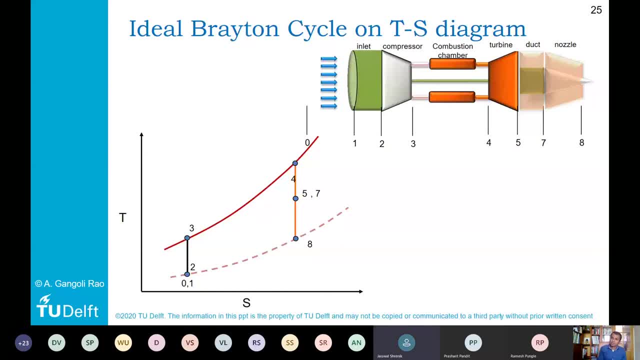 be used for whatever purposes, okay. so in case of a jet engine, of course it is used for uh, for creating thrust, whereas in industrial gas turbines you can add more turbine stages and then you can, you can connect it to a generator, you can produce power, you can also. 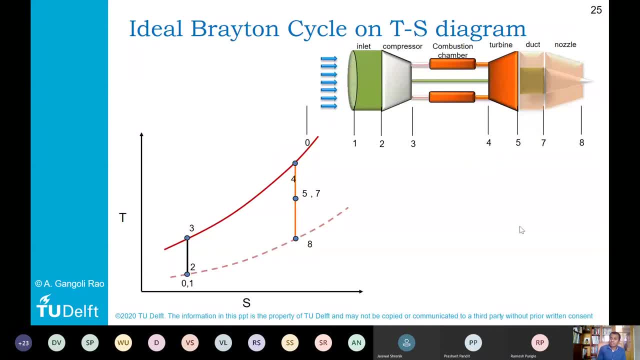 connect more turbine stages and then connect it to a rotor, like in a helicopter engine, or to a propeller, like in a turboprop engine, so you can do all kinds of things, yeah, but the basic working principle is still what is called as the weighton or the joule cycle. 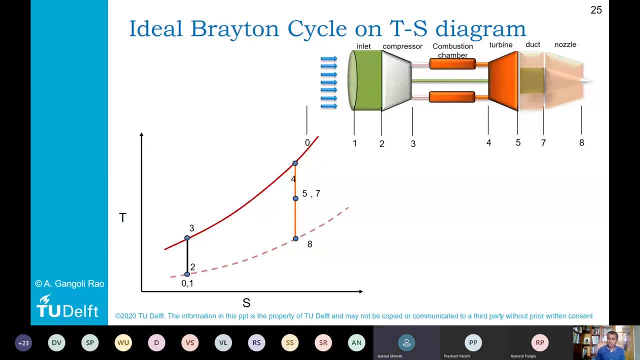 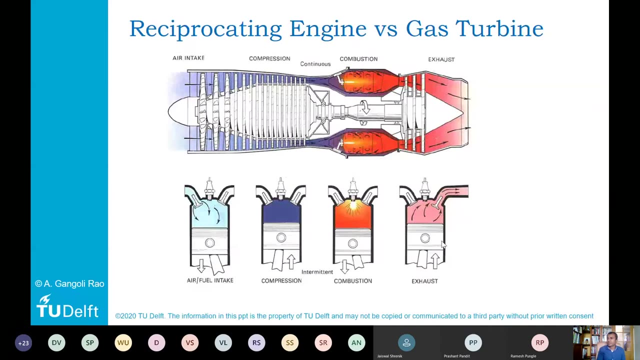 now, if you compare a gas turbine with an internal combustion engine, which you must have studied in your bachelor's, yeah, so the processes are not very different. it's still more or less the same. you, you have an intake, now you have a compression, you have combustion and then you have exhaust. okay, but the main difference is that, first of all, that 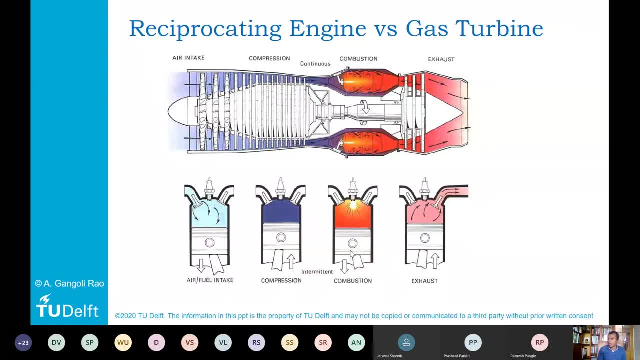 an ic engine in that sense is an intermittent cycle. so you have one power stroke in a four-stroke engine, of course, you have one power stroke in four strokes, whereas in a gas turbine engine, so there's a continuous cycle. yeah, and that's why the specific power output of a gas 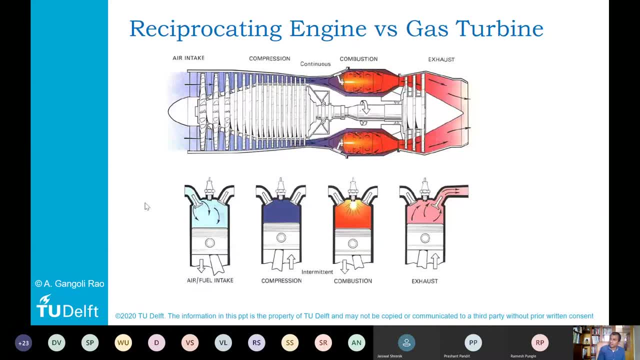 turbine is extremely high as compared to that of an, of an internal combustion engine here, or a reciprocating engine to be more precise. okay, so a reciprocating engine, which is which it has its own advantages, um, but uh is limit it, but it also has its own limitations, uh, whereas when you look at 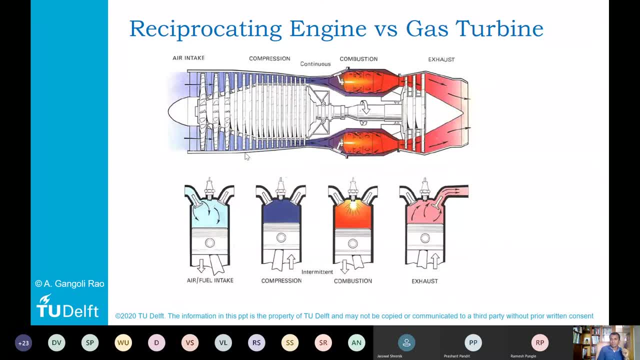 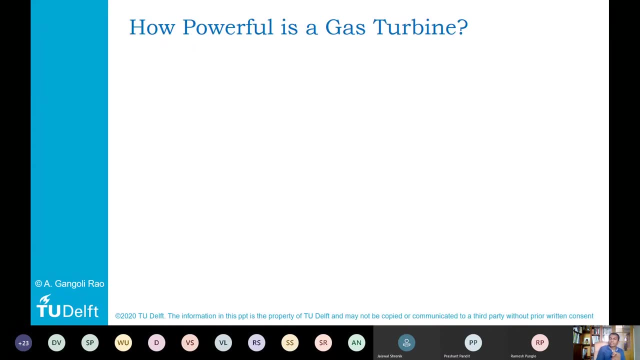 something like a gas turbine cycle. it is a continuous cycle and specific power output can be much higher and also the efficiency can be much higher if the pressure is much higher, if the pressure ratio, if the operating pressure ratio is high. okay, so let's see how powerful is a gas? 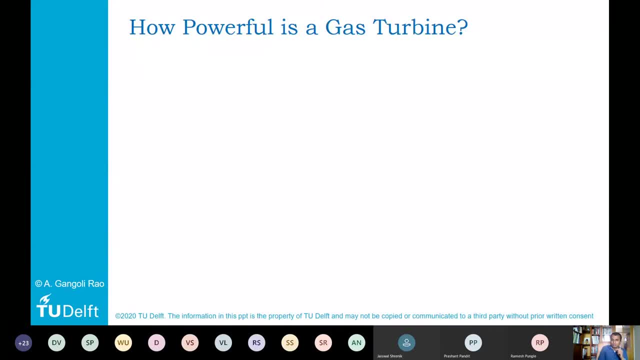 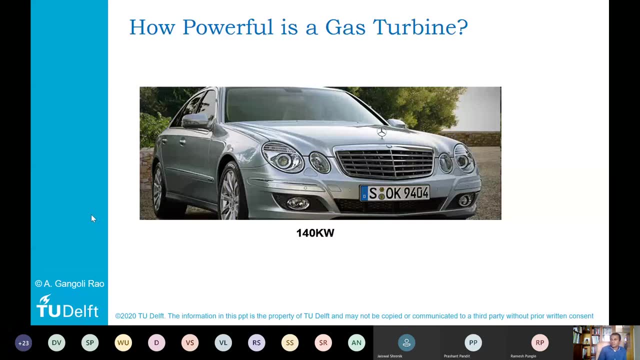 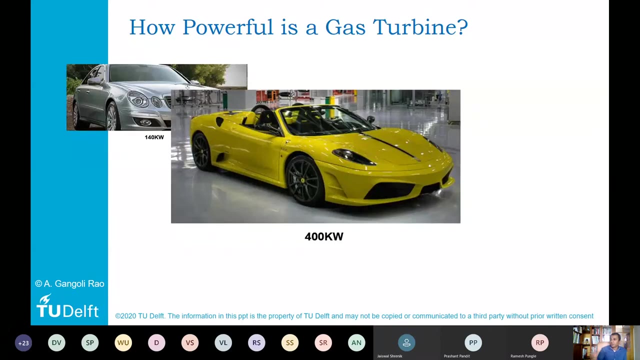 turbine, yeah, um. now, just for the sake of simplicity, you know well, if you have a fancy car, yeah, then you typically have around 150, 200 kilowatts of power, okay, um. and if you have even more fancy car, so people who don't know what to do with their money. 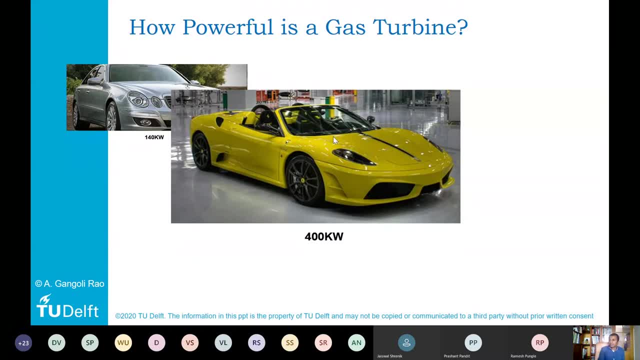 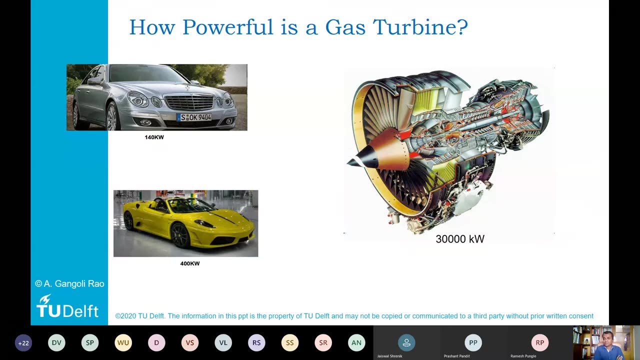 and are mentally not grown up, so they buy these kind of fancy cars like ferrari, yeah, and well, you can see, uh, you can have around 500, 400 kilowatts of power, okay, but then if you look at one engine, um of something like 747, okay, then you have approximately around 30. 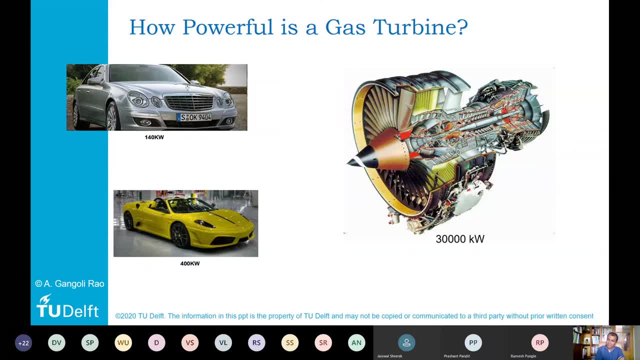 000 kilowatts of power that has that is produced. so you see that the difference in the magnitude of the power, so that means that one turbofan engine, yeah, is almost equal to around 80 ferrari engines. okay, and remember that at full takeoff thrust, uh, your aircraft has a bigger aircraft. 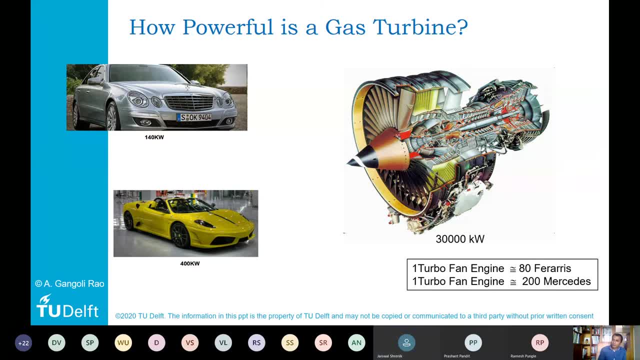 like a380 or, let's say, 747. they have four of these engines. so so that's why, uh, you can accelerate uh from sands stanston to around 250 kilometers per hour in such a short distance, in such such a short time. then you can take off. so so this high amount of power is is something that is. 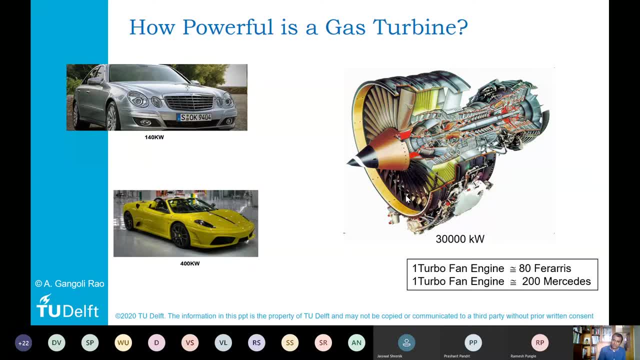 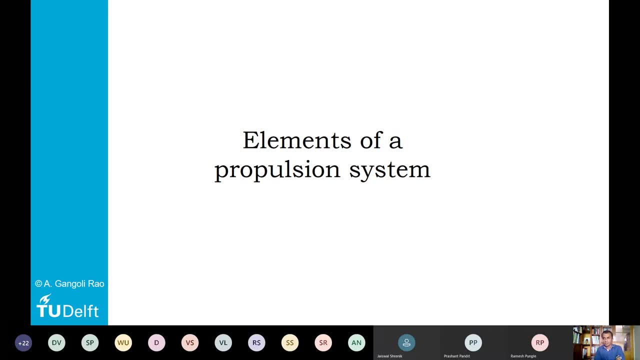 a speciality of gas turbine and that's why we use these in aircraft. again, if you have any questions so far, please put them in the chat box and I will answer them. okay, up till now at least, I don't see any questions. okay, so let's look at. 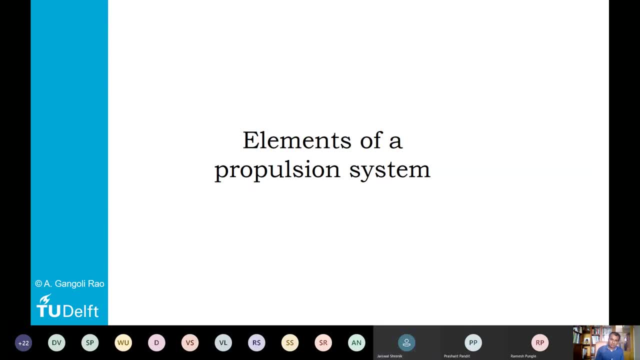 the propulsion system in a different way. okay, so what are the main elements of an aircraft propulsion system? so, first of all is that there are three main elements, okay, first is that energy source. so you have to carry an energy source on board an aircraft, okay, which will provide the energy. now, this you. 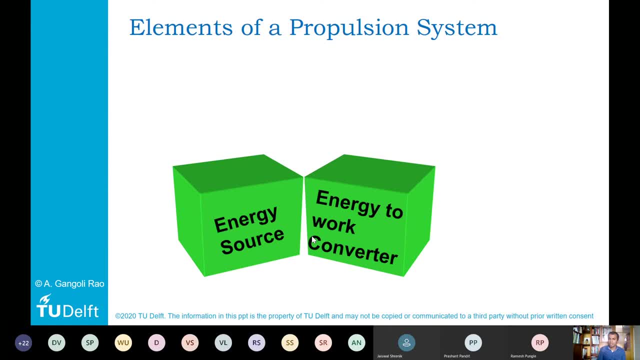 have to convert this energy into work, okay, and this work then has to be converted into thrust, and of course, you have to do this all, sorry, and you have to do this all in conjunction with the aircraft and its mission. okay, and what do I mean by this? I'll give you some examples, so for 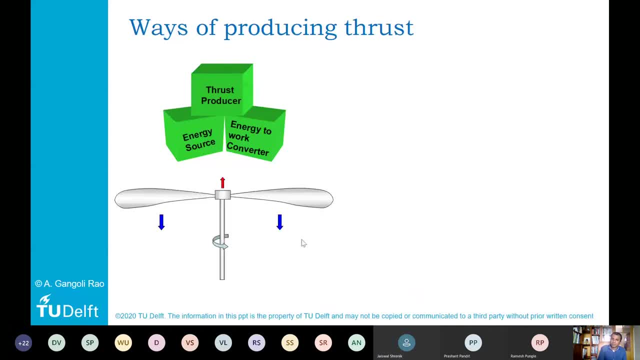 example, in terms of energy source, sorry, in terms of the thrust converter. we already saw these examples, so we could either use a kind of a propeller or, if you have to create thrust, okay, so we already looked at that, okay, so. so, so this part is covered in terms of the energy source. okay, we could use. 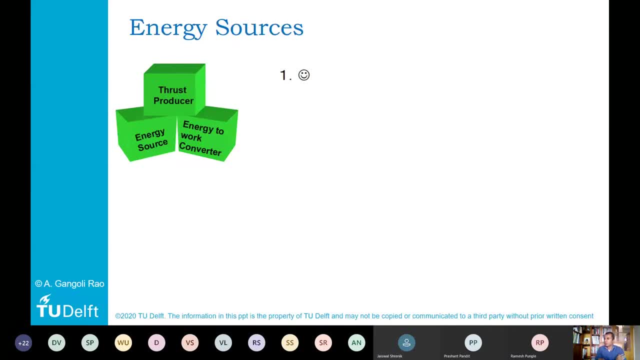 different energy sources. so for the students who are out there, maybe you can write some of the energy sources that you can use for aircraft in the chat box: what do you think of the different types of energy sources that we can use for airfacts? so let's write a few examples that I'm gonna go through just like we have done. 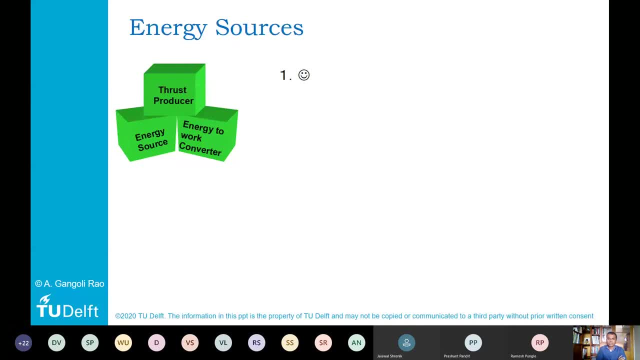 all our classes already and I just wanted to let you know I've done a couple things um. so here, first of all, if you have a like air travel truck, or if you have a ome, it can be, or it can also be, a second type of airfighter. 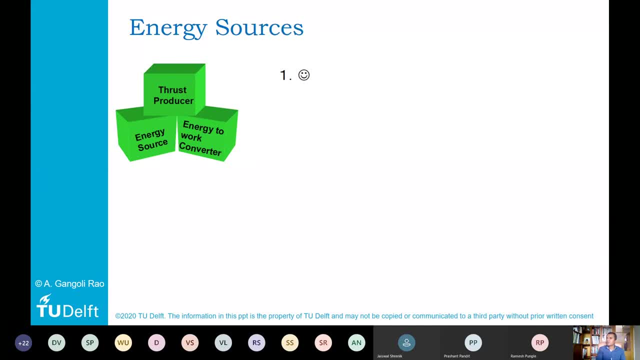 airf를 truck or longer aircraft like a metel Aer квár drift or something, or something else. so don't be shy. is there a problem with the chat box or they are blocked? sorry, they are blocked. the chat is blocked. yes, okay, i'm sorry to hear that, but you could also say, actually, that's not a problem. 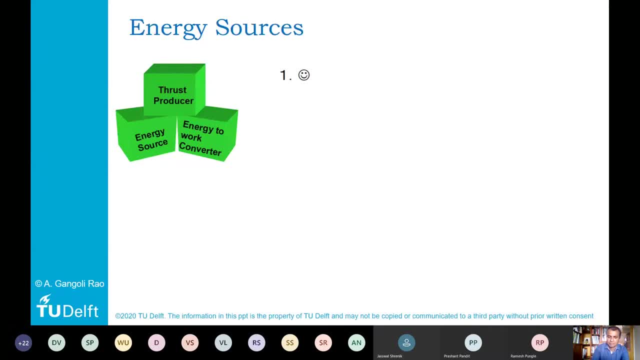 okay, so, um, of course, um, dr puglay said that we can use solar energy. yeah, so, so the solar energy. you can do that now you have to use solar cells and but the amount of solar energy which is coming on an aircraft is much less. but there was one attempt, what was called a solar impulse. 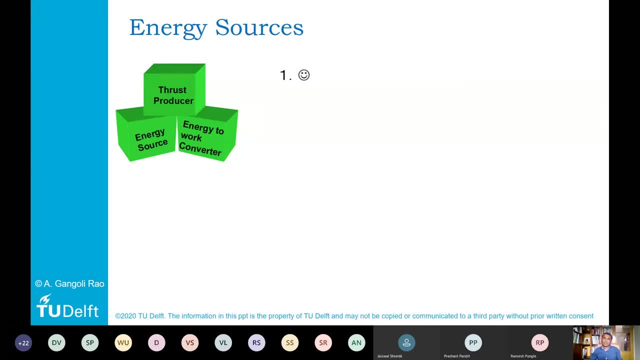 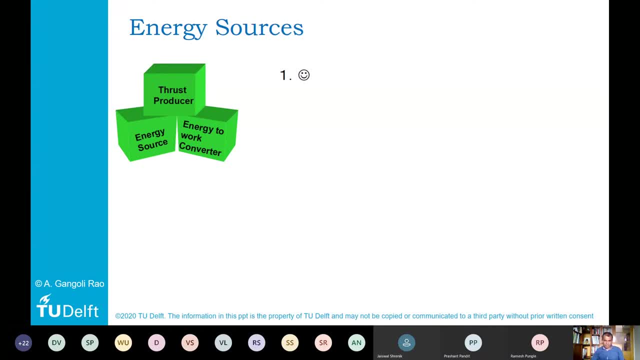 longer than that of 747 aircraft, and so it could generate- that's a sufficient power to just for one person to take off and fly at a very low speed now. so solar energy can be used for also for unmanned aerial vehicles to some extent, in order to sort of charge the batteries. 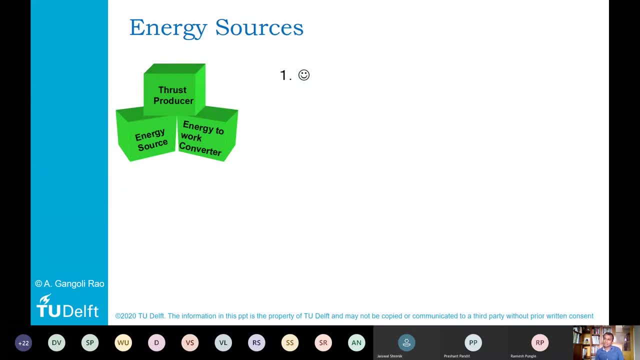 or at least to extend the life of the batteries. but for commercial aviation, solar energy cannot be used. so what is used typically? yeah, so of course, batteries. you can charge batteries and this is all always used for drones. yeah, and one of the characteristics that is used to characterize 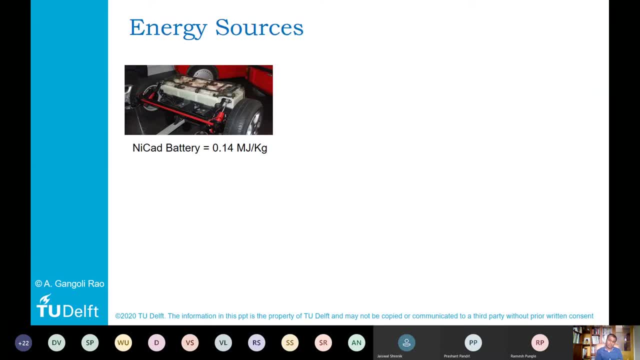 the energy sources is to see how much amount of energy can you store per kilogram of that energy source. yeah, so energy density, okay. so if you have a solar power plant you can charge batteries. so when you look at a battery, uh say, for example, some nickel cadmium battery, of course there's. 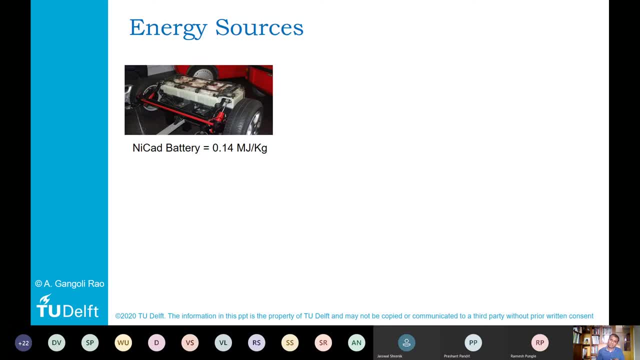 always a range, but these are some typical values that i'm mentioning here. yeah, so it's approximately around 0.14.15 mega joules per kilogram. okay, so not much, yeah, but if you take something like lithium ion batteries, then you can go up to almost one mega joule per kilogram. 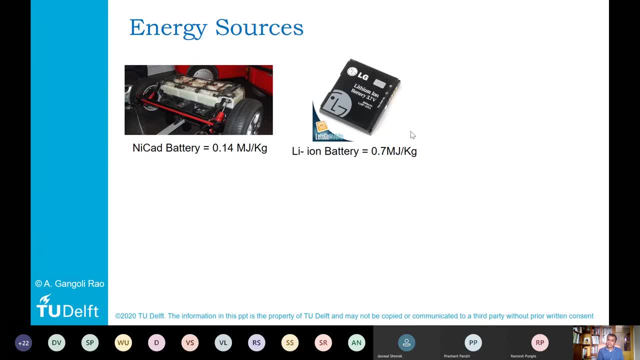 so, uh, you see that the energy density is already better for lithium ion batteries. yeah, of course there are some experimental uh batteries, like lithium, sulfur, sulfur and metal air batteries, where, uh, at least the hope is that uh, the energy density can go up to around two or 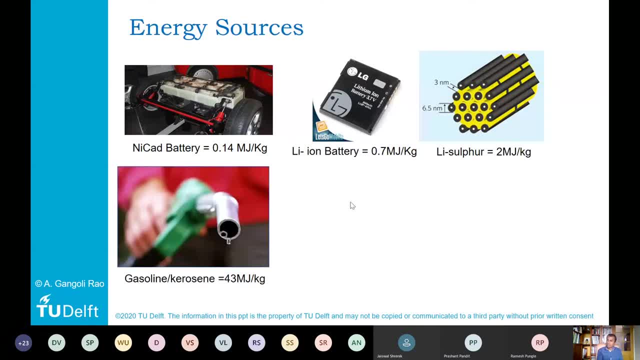 three mega joules per kilogram. but when you look at kerosene, that is typically used in aircraft, yeah, so you see that it's approximately around 43 mega joules per kilogram. so it's a kerosene is a very energy dense fuel. it is similar to a diesel, by the way, so so, so that's why, um, it's uh. 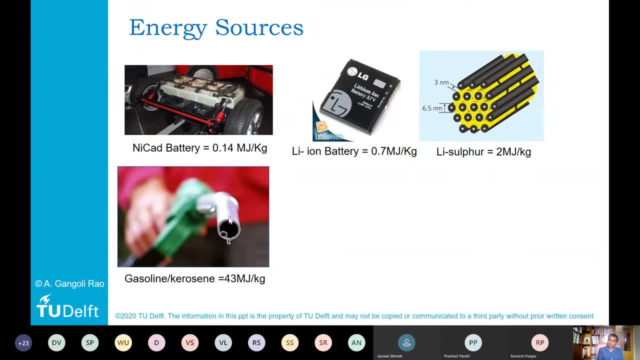 an aircraft can go to a very long distance because of this energy density. yeah, of course you could also. you think of hydrogen. yeah, hydrogen also has very high energy density, but it also requires more volume, and so if you want to carry hydrogen in an aircraft, of course you have to do it in a 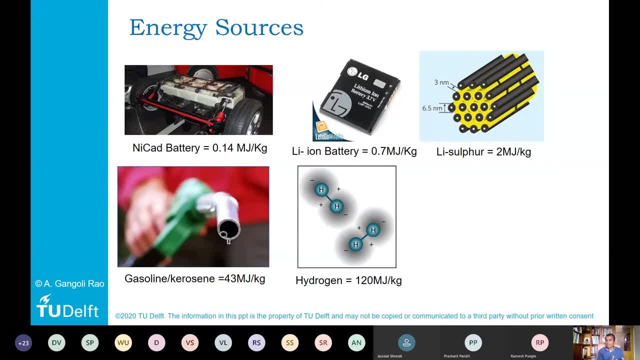 liquefied form, liquid hydrogen, and then liquid hydrogen has to be stored at under very cold temperatures, and that means that you cannot store it in the in the wings, and you have to store it in fuselage. i'll give you some examples of this later on. yeah, and, and that is a problem with hydrogen. 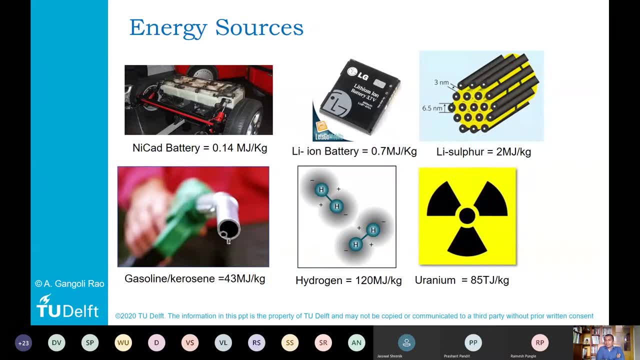 well, believe it or not, but uh, after the second world war, uh, in the in the 50s- actually in the late 14 in the 50s in fact- there were serious attempts of using uranium, or let's say a nuclear powered aircraft, both in us as well as in russia, and of course you see nuclear powered submarines. 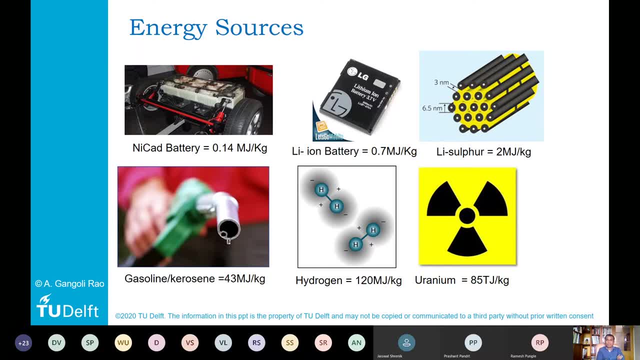 nuclear powered ships. so when you take something like a, an aircraft carrier, yeah, some, many of these aircraft carriers, they tend to be nuclear powered, so you can, you know, use these aircraft carriers for years. so approximately 15 years without refueling. yeah, of course, the problem with 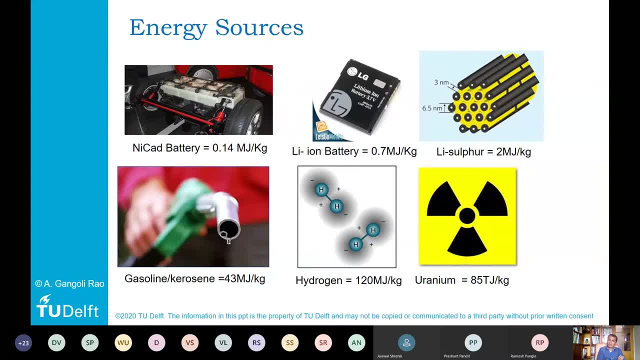 nuclear power on board an aircraft is that the weight of the shielding is is extremely high and, of course, in in in case of an unlikely scenario of a crash, something, then there is a there's a huge danger of radiation leakage. yeah, so that's why this is. 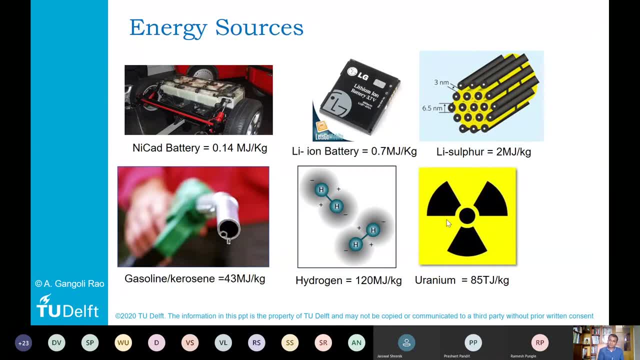 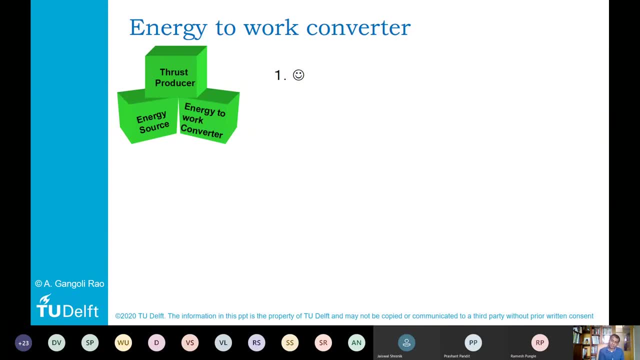 ruled out, but in principle, you can use different kinds of energy sources. okay, of course, you also have to convert this energy into work. yeah, to drive the propeller or to produce hot gases, which can then be used from the nozzle. okay, so when you look at different examples, of course 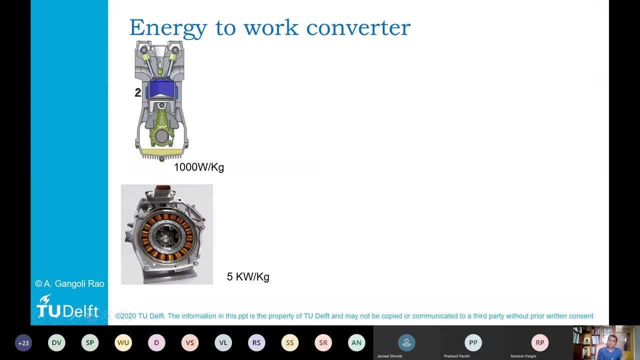 you. you talk about, let's say, ic engine, internal combustion engine, reciprocating engine. when you look at some of these engines- at least the state of the art- that are used for high performance cars, yeah, then you have approximately one kilowatt per kilogram. yeah, maybe a bit more. 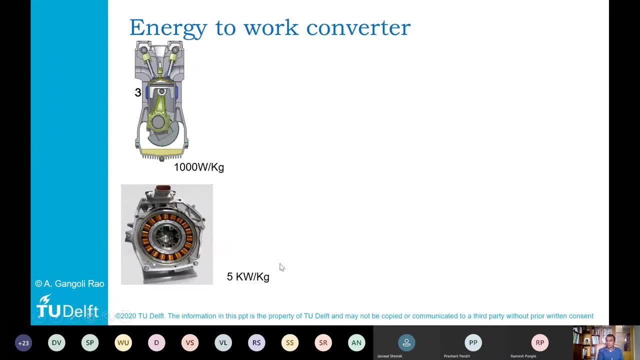 and, of course, if you use electrical motors, then they're approximately five kilowatt per kilogram. if you use bankers engines then they are around two and a half kilowatt per kilogram, but if you use a gas turbine then approximately it's around 10 kilowatts. 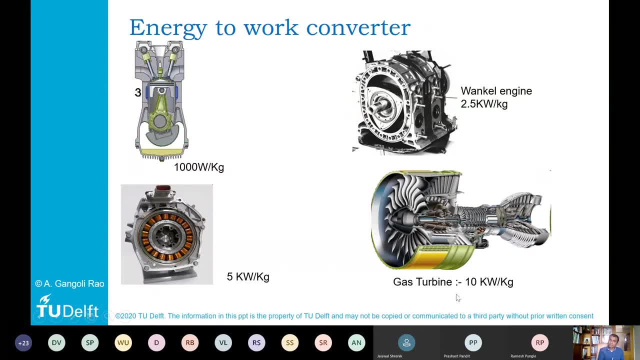 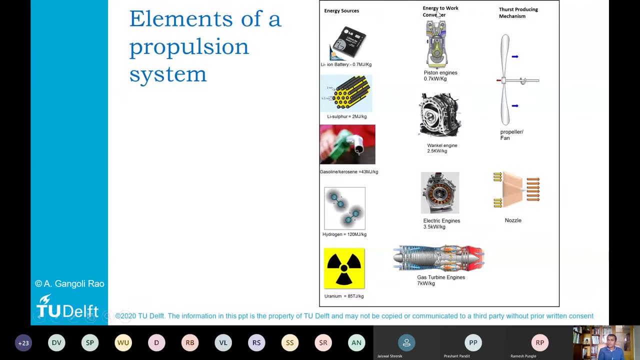 even more uh per kilogram. yeah, so. so, so you see that, uh, why a gas turbine is used? because it has- not only, i mean, it has- extremely high uh power density. yeah, um, so in a sense, you can use different types of energy sources- what you see on the left here. yeah, with different kinds of energy converters. 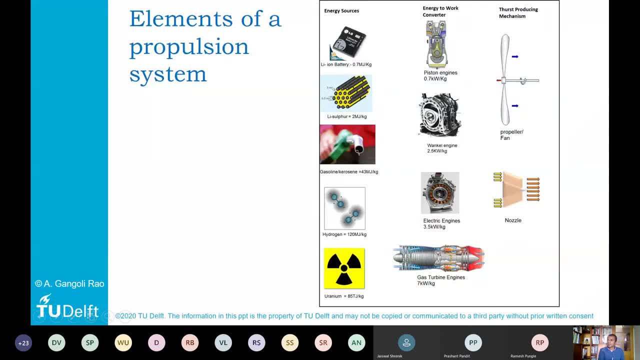 in the middle and different thrust producers. okay, so, for example, for a, for a drone, what is typically done is, of course, you use something like a battery with an electric motor with a propeller. okay, um, of course, as and when different kinds of batteries are available, you can use different kinds of batteries. yeah, with electrical motors and. 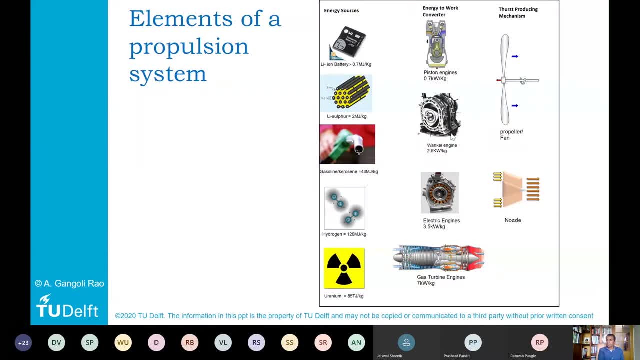 propellers- okay, you could also use the gasoline and a vehicle engine and a propeller- okay. or you could use hydrogen with gas turbine and a propeller, or hydrogen with gas turbine with a nozzle- yeah, so you can use different permutations and combinations depending on the aircraft type and the mission. 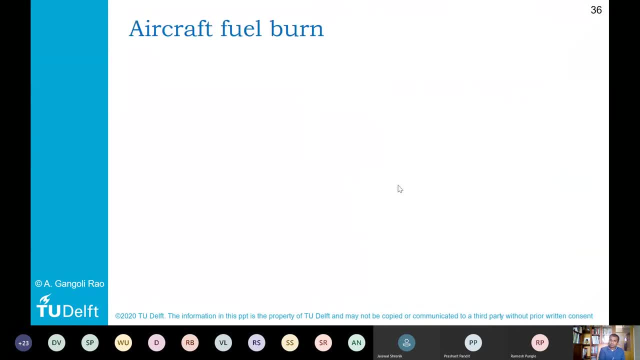 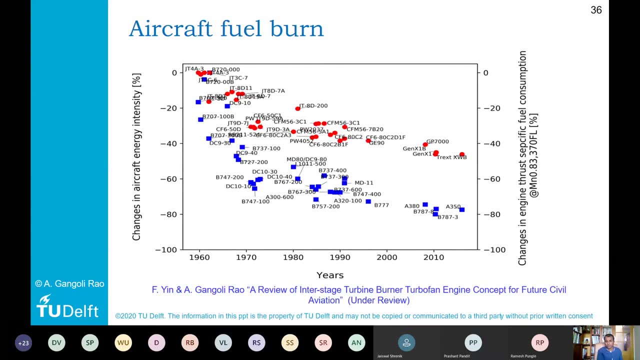 okay, um, okay. so let's look at, um the fuel burn. so what this graph shows you is the increase in the efficiency of aircraft over the period of time. okay, so on the left axis, what you see is, let's say in a non-dimensionalized way, um the amount of fuel consumption per passenger per kilometer over the years. and all these blue. 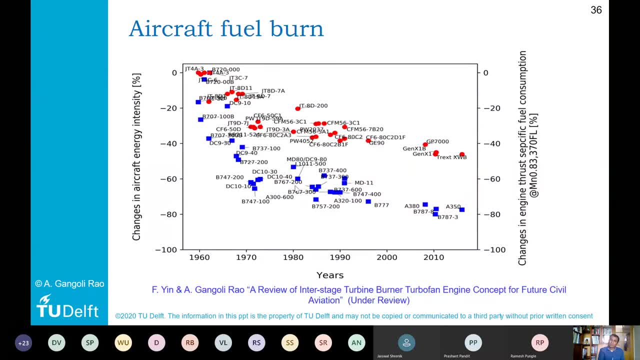 dots, you see, are the different engines okay. so as compared to the earlier jet engines in the in the late 50s and the early 60s, so when you look at a state-of-the-art, let's say a350, for example, then the fuel consumption is approximately 75 less okay, and that is also one of the reasons why. 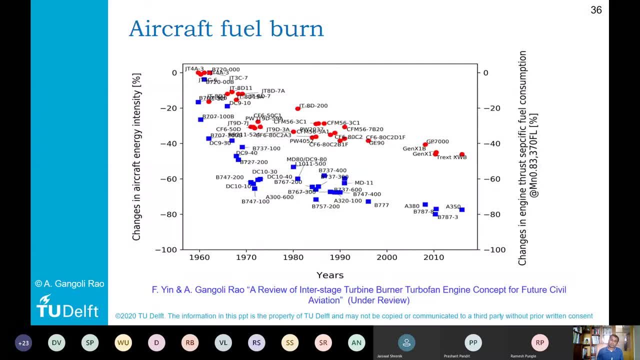 over a period of time, aircraft tickets have become much cheaper. i mean, more and more people in the world fly today than ever before. of course, i'm talking about pre-corona times, yeah, and, and flying through in an aircraft is not so expensive anymore, and one of the main reasons 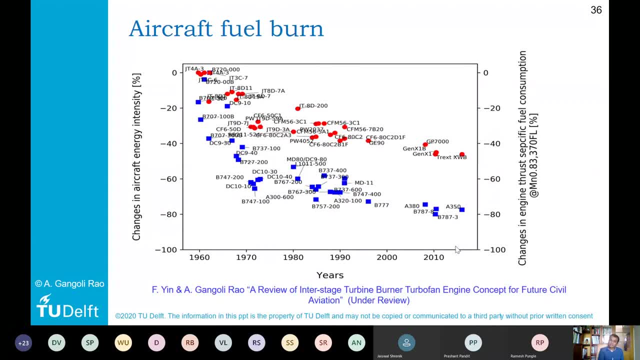 is because of the decrease in the fuel consumption, because fuel cost is one of the main cost for an airline. okay, and these red dots that you see are the engine fuel consumption. okay, so of course, if the engine fuel consumption reduces, then the aircraft efficiency increases quite a lot. 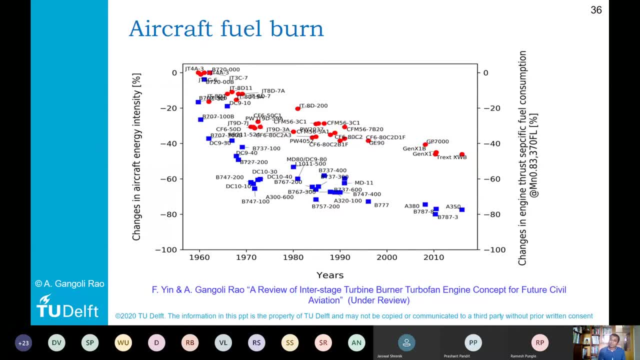 the aircraft not only has to carry less fuel, but also because it has to carry less fuel then it can be lighter, and so on and so forth. so there is a kind of a snowball effect. okay, so engines have become much more efficient, and that means that the aircraft also has become. 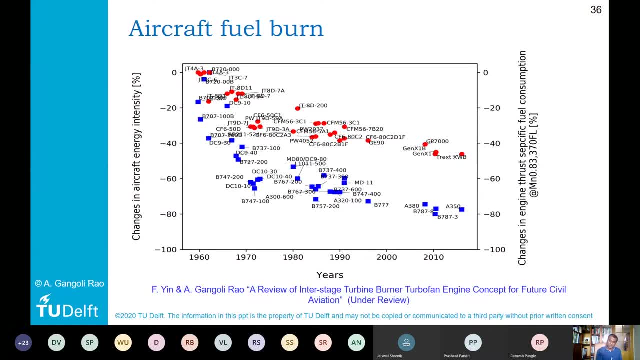 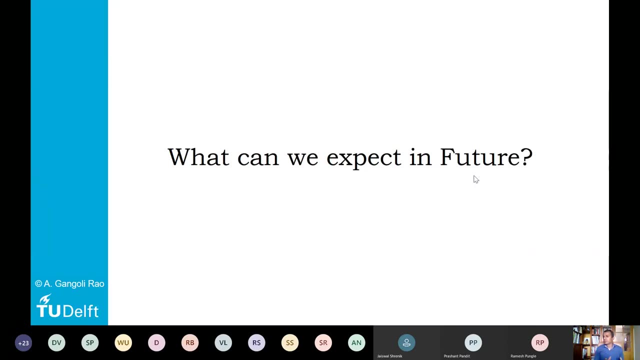 more efficient. of course, there are other things as well. for example, the aerodynamics of the aircraft has improved, the the structural weight has reduced, so on, okay, okay. so we covered a bit about the history, a bit about the basics of propulsion, and the question is: what can we expect for the future? okay, so let's take a look at that now. one of the things, what you 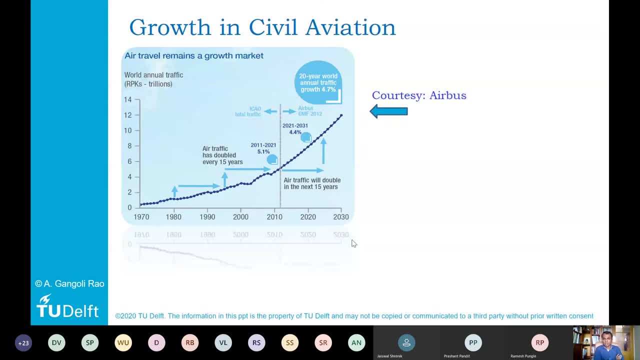 see here. sorry, one of the things is, as we were talking about, is because more and more people are traveling, okay, so you see more and more aircraft going there at any point of time, yeah, so what you see here are: these are the passenger numbers of the aircraft, and they do it pre-corona. 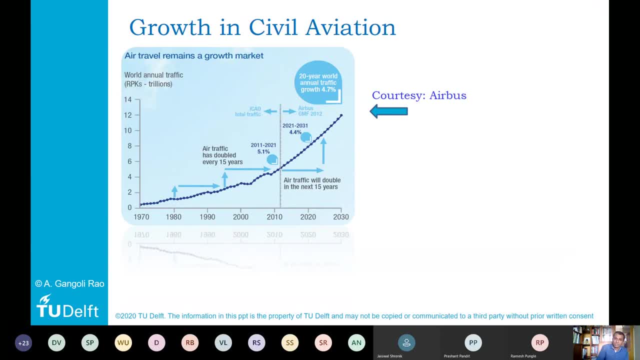 times um. so there are around 25 000 aircraft in the air being used worldwide, um, and what you see here is the increase in the passenger numbers. so, right from the- uh- let's early 70s to now, so this is so approximately around four and a half billion people. 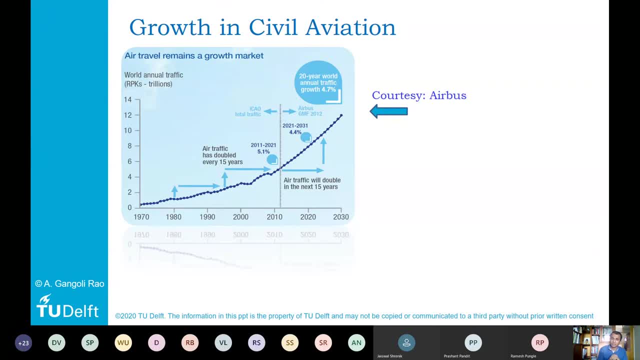 or passengers late 2019 or early to 2020, before governor crisis happened, and it is expected. i mean the air traffic is growing at around four, five percent every year. of course, in it depends uh from region to region. for example, in india it grew at in double digits uh 12, 13, 15 uh, whereas in europe and so on, because 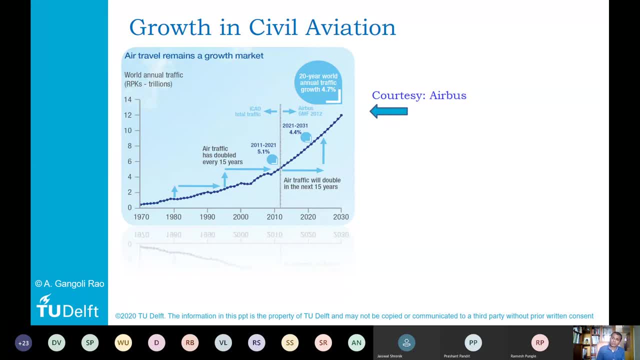 of: uh, we are already at a developed stage, so the growth was not as much, okay, but still, uh. when you look at the worldwide average, it has grown over more than five percent over the last 10, 15 years. okay, so, which means that the air traffic actually doubles every 15 years? yeah, um, and so, so that is. 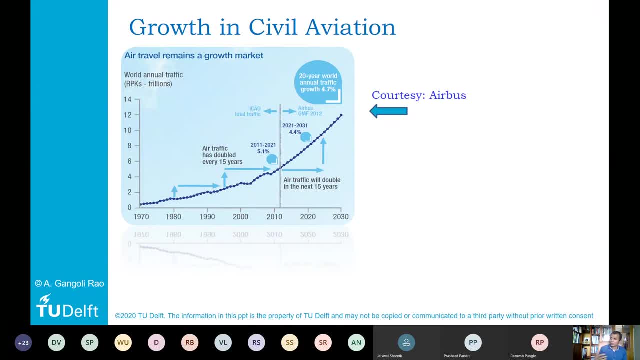 a huge challenge, of course, uh, and that's why you know there are longer lines in airport, and so on and so forth. okay, so what you see here, uh, in this graph, is, um, and this is coming from our own book now- what you see here is, uh, the: the number of passenger. 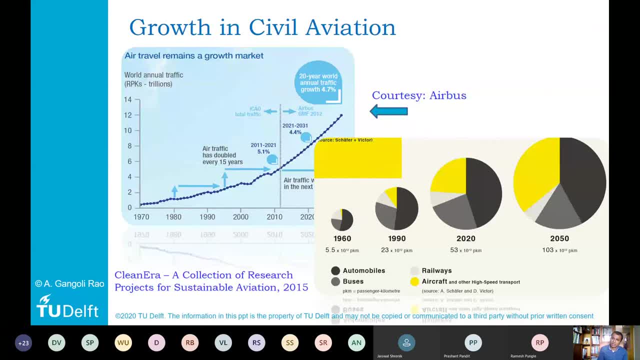 uh, kilometers traveled by different modes of transport. okay, so, so, so that, um so, the black represents automobiles, the grays buses, and then you have the light gravities rails and, uh, the yellow is aircraft. and, of course, in the 60s hardly anyone traveled with air traffic. but um, 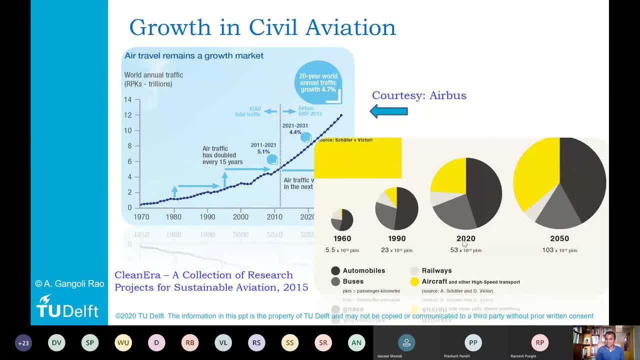 coming coming today. um well, incidentally, in this year we used 2020 as a baseline and, uh, but nevertheless, if corona wouldn't have happened, uh, so we would have gone here. okay, so we already see that a large number of passenger kilometers is actually covered by 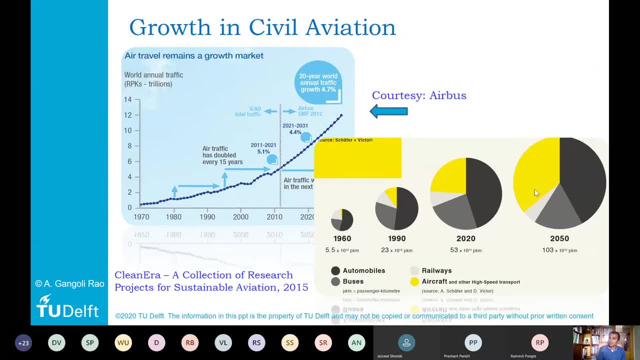 aircraft and in by 2050. so air travel as much as road travel, of course. what you see is that in road travel, electric batteries are coming into and electric vehicles are coming into, and not so much in india but in rest of the world. if you look at china, for example, a large around half a percent- i. 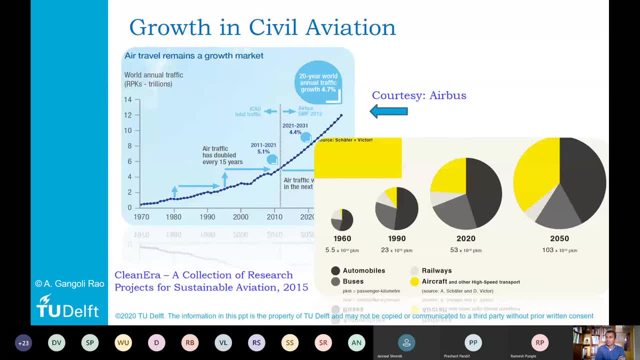 think, approximately around 50 percent of all the new uh cars that were sold. a large majority of them were electric cars. okay, so this is very good for from a local environment perspective. of course, you also have to take into account how the electricity is generated from. if the 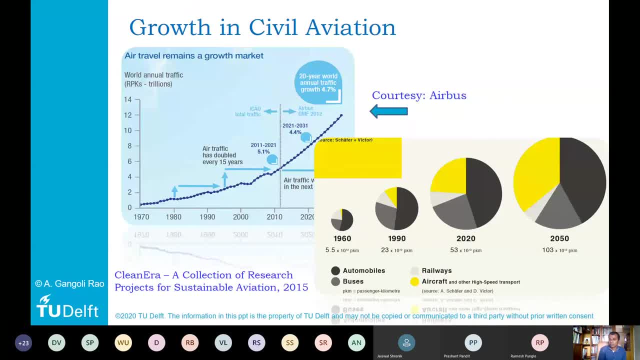 electricity is generated from a coal-fired power plant, then it's not good, but if the electricity is generated from a wind turbine or using solar energy, then it is good. okay, but coming back to aviation, you see that it is projected that, because of the increase in the 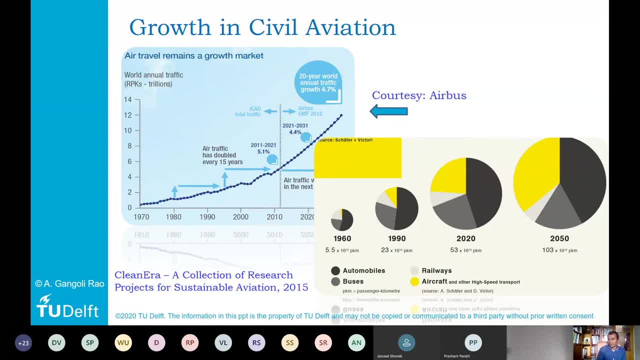 growth of aviation. so, in terms of passenger kilometer, aviation would be as much as as road transport, which means that the emissions from aviation will actually surpass all of the emissions. okay, and that is quite a big challenge, okay, uh, already, uh, people who live around airway. 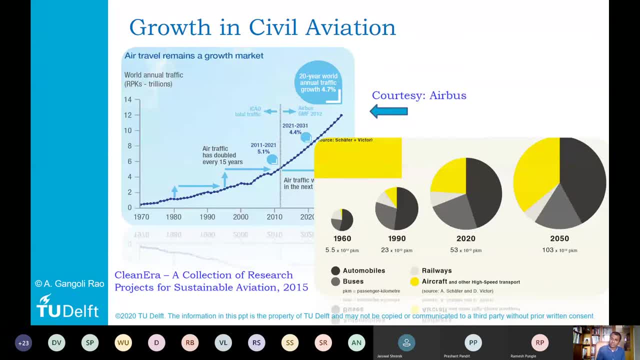 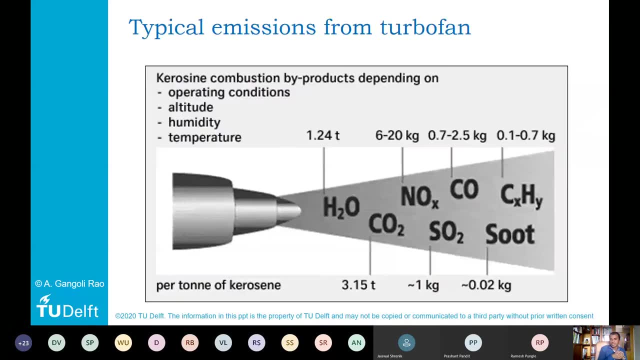 airport and so on. they complain a lot about pollution, about emissions, about noise and so on. so so that has to reduce, okay. so when you look in terms of um emissions that come out from an aircraft, of course it's burning kerosene, so there are emissions and apart from water vapor and co2, 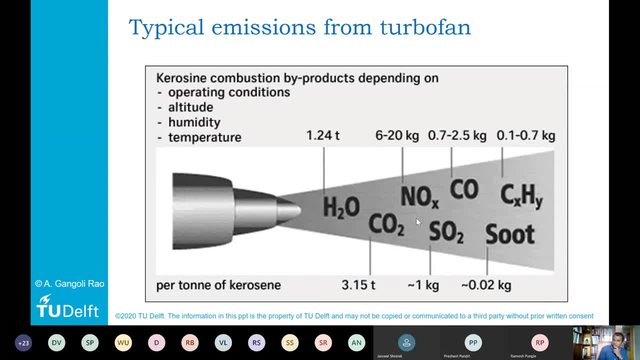 which is the product of any hydrocarbon combustion. so you also have nox, which is called no no2, and then there you have sulfur dioxide, you have carbon monoxide, you have unburned hydrocarbons and you have soot. so all these emissions, they have different impacts. so at the ground level, of course, near the airport, 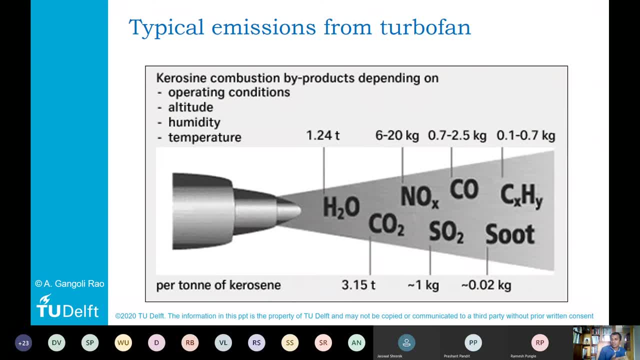 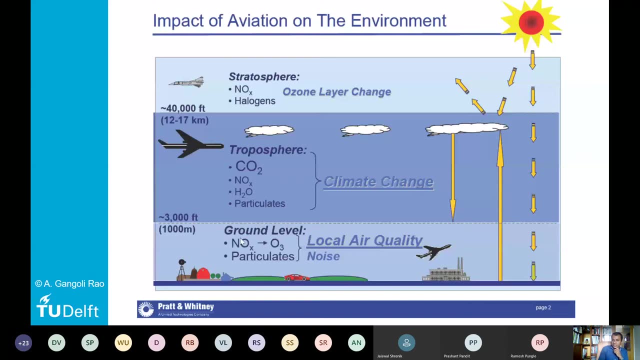 they have a different impact, but when the aircraft is cruising at 10 or 11 kilometers altitude, then it it has a quite a big impact on the global warming. okay, so, so these are the things that have to be reduced. so around, uh, up till around thousand meters, let's say, around a kilometer. 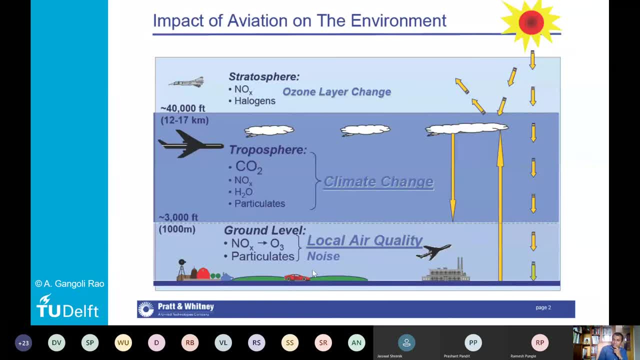 of course, uh, the local air quality uh is, uh is changed because of uh aircraft, but when it is flying at uh 10, 11 kilometers altitude, then it changes the climate. yeah, um. so so that are, of course, and these are for military aviation, but uh, that, um, i mean from a, from a volume. 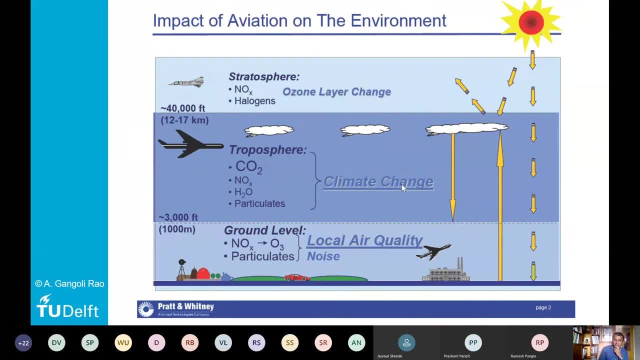 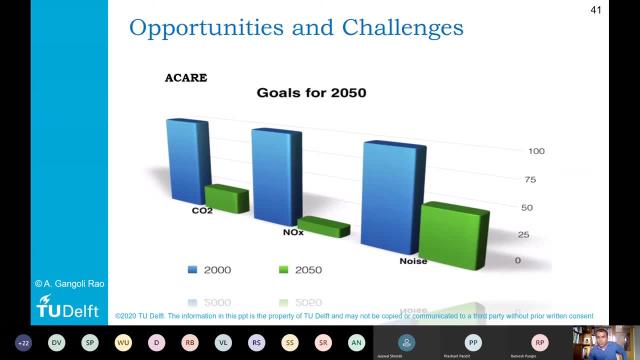 point of view, it is not so much as compared to civil aviation. okay, okay, so, um, now, at least in europe and also in us, um, so there is this advisory committee for aeronautics research in europe and, uh, the aim is that, uh, you know how, how will aviation grow in the coming years? 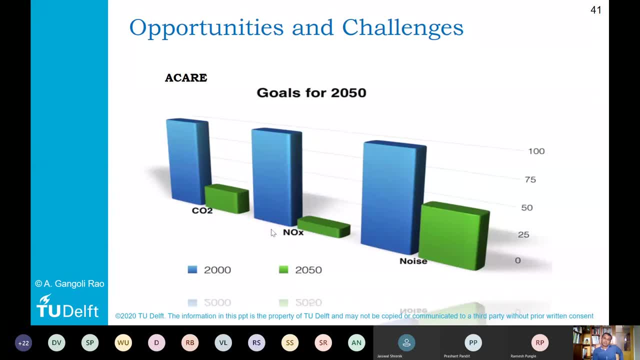 and the idea, or at least the goal, is that, um foreign uh for an aircraft, let's say for a new aircraft in 2050, um, the aim is to reduce uh the co2 emission by approximately around 75 percent as compared to an aircraft in 2000, okay, and uh the nox emission by around 90 as compared to an. 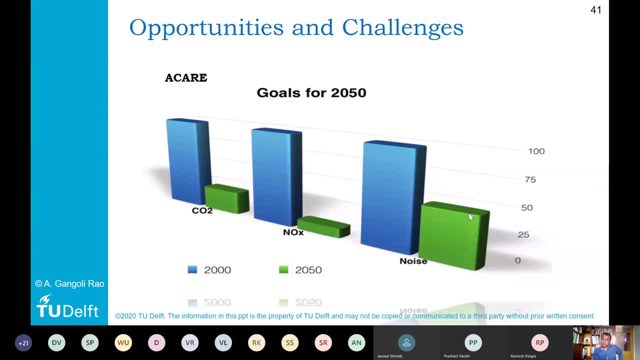 aircraft in 2000 and the noise emission by around 65 as compared to an aircraft in 2000. okay so, and these are extremely ambitious goals, and this is where let's say, um, europe, and as well as the european commission, is putting a lot of emphasis on uh and money in terms of making sure that our 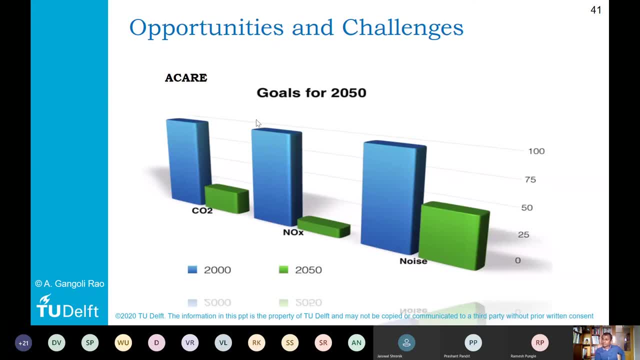 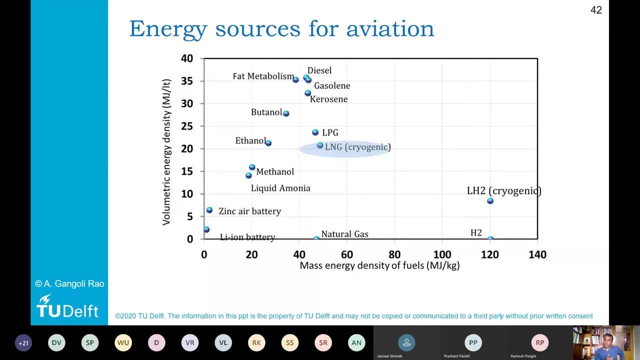 aircraft become more sustainable. okay, so that is a. there's a huge political drive also to reduce emissions from aviation, and one, of course. you see, we have to make the engines better, we have to improve the aerodynamics, we have to reduce the structural weight. but one way to reduce the emissions from aircraft is also. 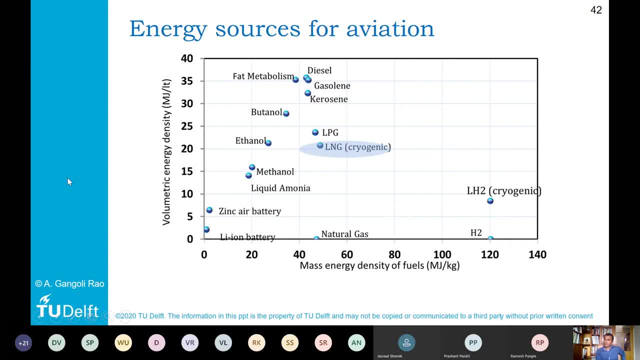 to look at different energy sources. yeah, so, of course, when we talk about energy sources, uh, again coming back to mass energy density, this is one of the main criteria, yeah, and the other criteria is what is called as the volumetric energy density. okay, um, well, i see a question here, uh, from dr pungle, and that is: can different layers affect the? 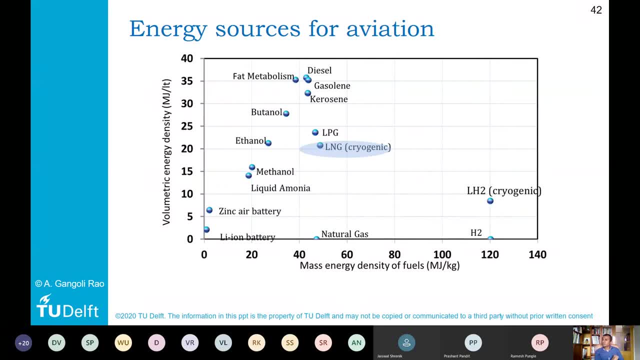 performance of the aircraft. um, i think, uh, do you mean different atmospheric layers? and if that is the case, then yes, i mean, uh and a normal simulation atmospheric layers. okay, yeah, thanks, uh, so a normal aircraft is always designed to go around in, in the edge of uh. 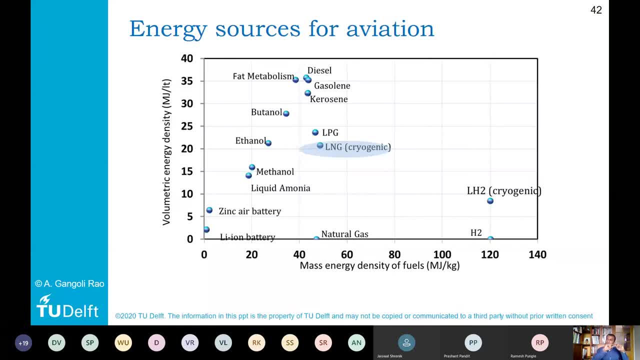 troposphere. so we have the troposphere and then what is called as the tropopause, and then you have the stratosphere in the atmosphere. yeah, and typically that occurs at an altitude of around 10- 11 kilometers. yeah, so the temperature reduces as you go up above in the troposphere, at around 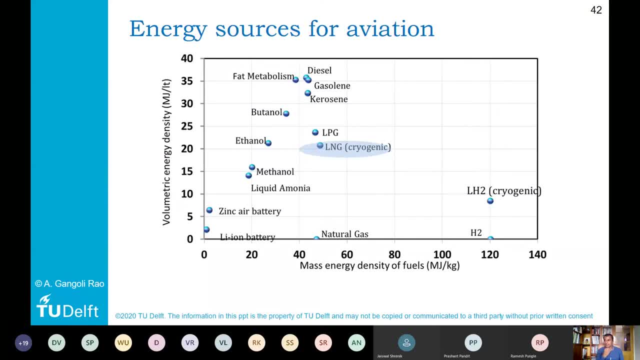 six and a half degrees per kilometer, yeah, and the weather phenomena that we all experience happens at much lower altitude. so typically, the aircraft is flying above the weather. okay, so it's tough. it's flying at around 5 degrees and the weather phenomenon is at much lower altitude. so the aircraft is flying above the weather. okay, so it's talking, it's flying at. 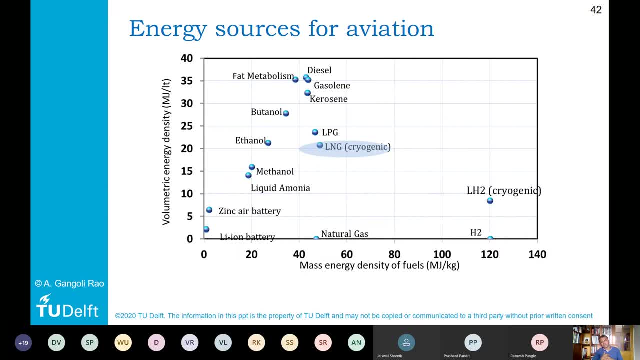 around 10, 11 kilometers altitude. now the air pressure at that ambient, at that altitude, is pretty low actually. so the air pressure is approximately one-fifth of- uh, one-fourth to one-fifth of what you experience on the ground, yeah, which means that the cabin, the air cabin, 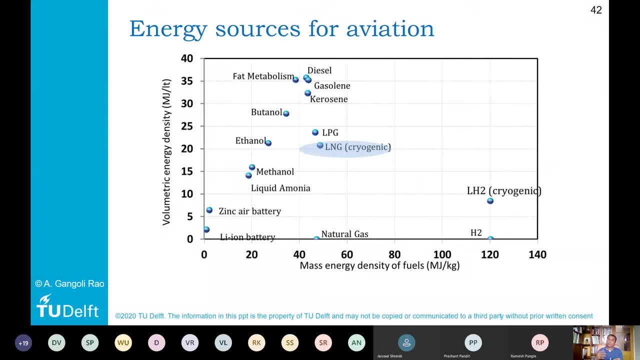 has to be pressurized, okay, and the temperature outside is typically around minus 40- minus 50 degrees, which means that the air conditioning system has to account not only for the pressure but also for the temperature. yeah, and you have to have a lot of insulation, otherwise. 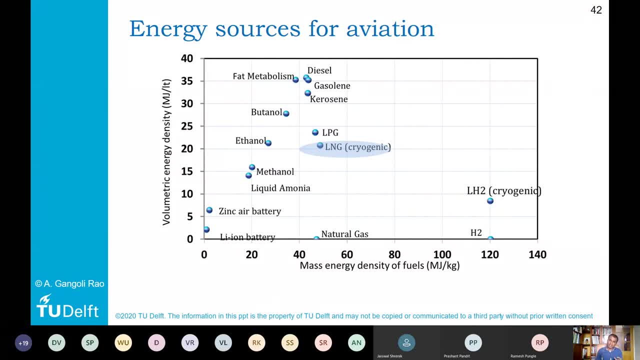 we would all freeze inside an aircraft. okay, so, yes, so. so that is in terms of the aircraft design, let's say, but the advantage that we are flying about, the weather, um, and the fuel consumption of the aircraft also reduces because you, because the air density is quite low. 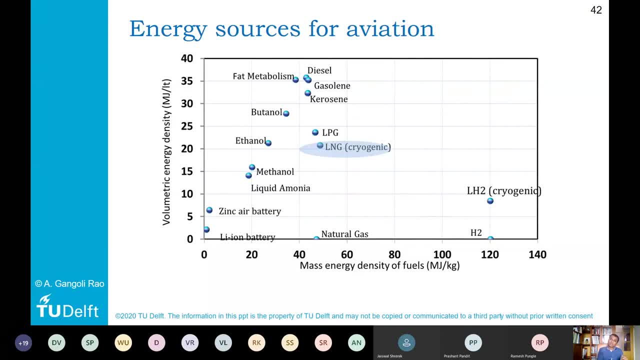 and it's less than half of what is at atmosphere, so the drag of the aircraft reduces quite a lot. okay, so then, aircraft is typically designed to cruise at around 10- 11 kilometers altitude- most of the civil aviation aircraft, of course business aircraft- they go a bit higher, so business. 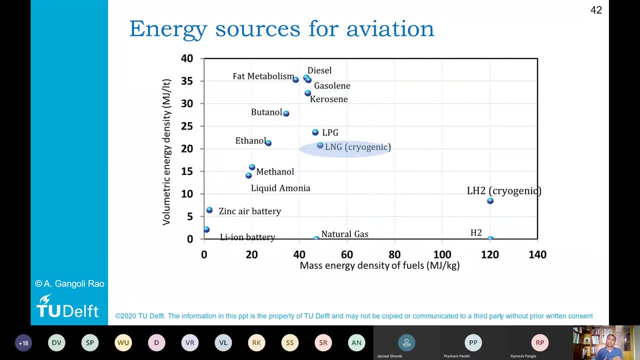 aircraft: jet aircraft- they are typically going at around 12- 13 kilometers altitude. turboprop aircraft: they go at much lower altitude, approximately around five, six kilometers, but they go much slower, yeah, so even when you look at the airspace, there are actually highways, yeah, and these highways are uh, sort of differentiated, uh with respect to the speed of the of the jet. 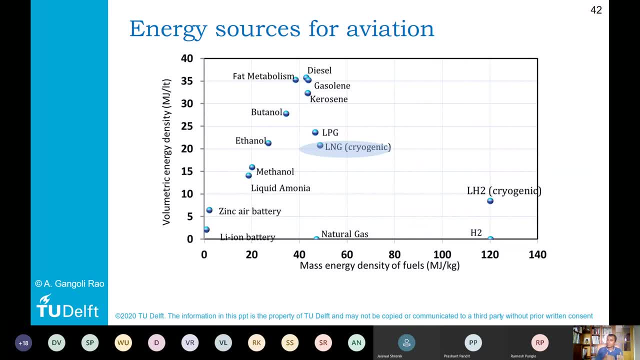 of the aircraft. the turboprop aircraft are typically slow, so you cannot put them in the same um line with jet engines, because then you will create all kinds of traffic jams and so on, and you don't want any crashes there, yeah, so turboprop aircraft, they go at a much lower altitude. 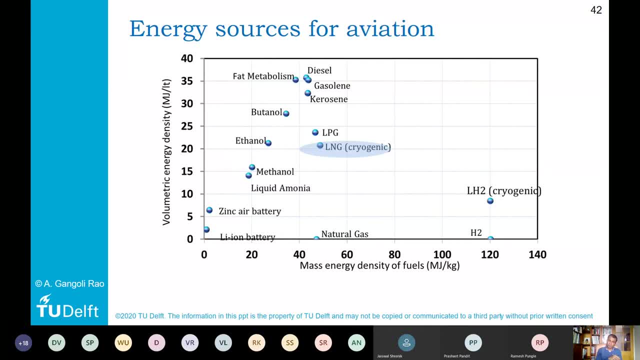 and turbo fan or turbojet uh aircraft, they go at a higher altitude. now the military aircraft, they can go at a much higher altitude as well. so typically military aircraft, they go supersonic. and in order to fly supersonic you really have to go higher, because then the air density is. 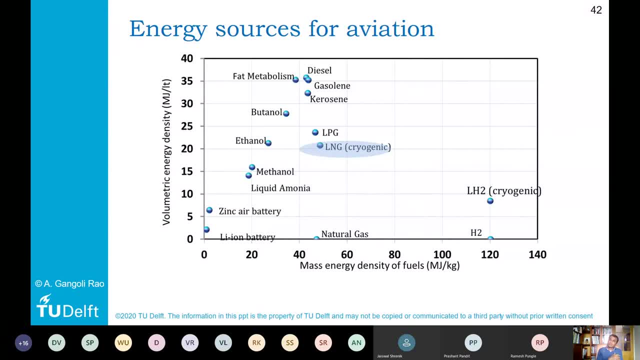 lower and then the drag reduces further, but anyway, so they can go up to 18, 19 kilometers or 20 kilometers in altitude. yeah, so they are. i mean, a military aircraft in that sense is much more difficult to be designed. um, yeah, okay, so of course. uh, so the different layers of 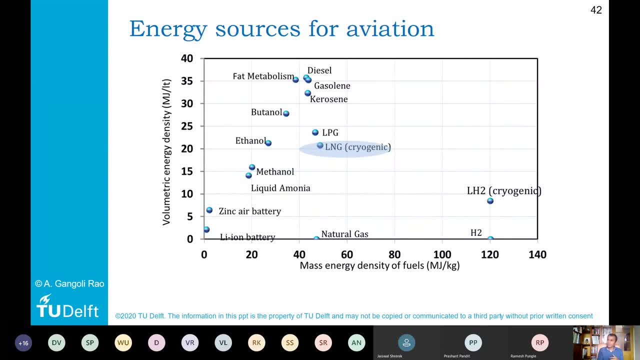 atmosphere. they have quite a big influence in terms of their performance. okay, now coming back to energy source. so you see that, for example, kerosene is here, yeah, uh. well, incidentally, fat metabolism is also here, uh, we can all use here. you see, batteries are here, so batteries are pretty. 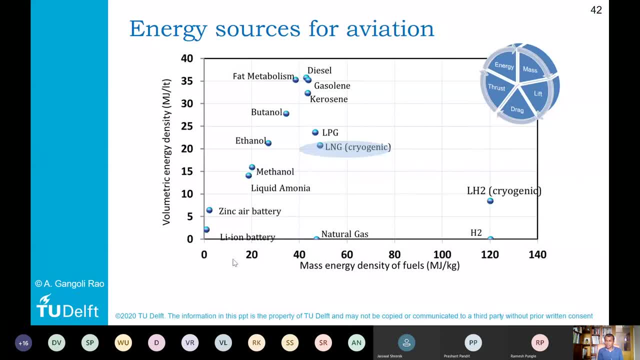 poor in terms of energy density. they're both volumetric as well as mass energy density. now, um lng is something interesting. lng is liquefied natural gas, so natural gas has quite high energy density but very low volumetric energy density, so which means that you require large volume to store natural gas, and that's why natural gas is either always compressed, 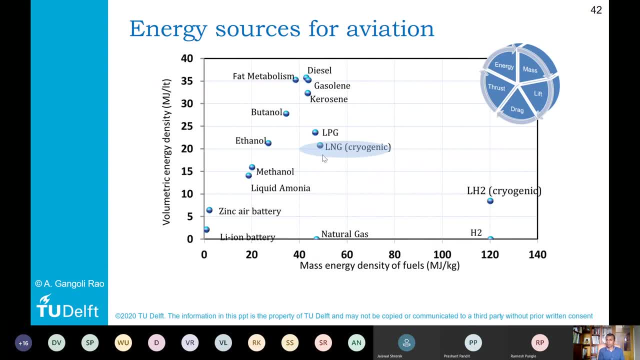 or liquefied, and if you liquefy it, then the energy density increases quite a lot. okay, and when you look at hydrogen again, hydrogen has a very high energy density: 120 joules per kilogram. so that's approximately three times more energy dense as compared to kerosene. 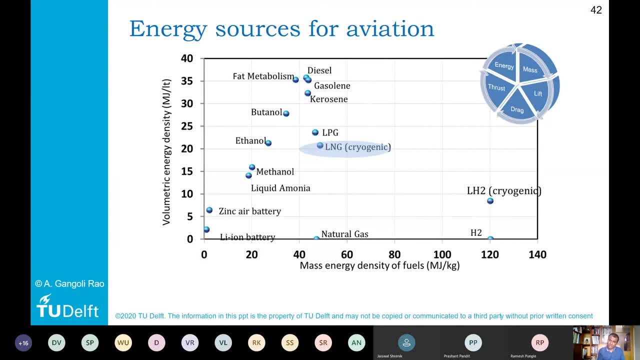 so that's very good, which means that, in terms of mass, you don't have to carry a lot of hydrogen. but the problem is that when you, even when you- liquefy hydrogen, the volumetric energy density is lower, which means that the volume of the aircraft will increase. okay, so? so these are. 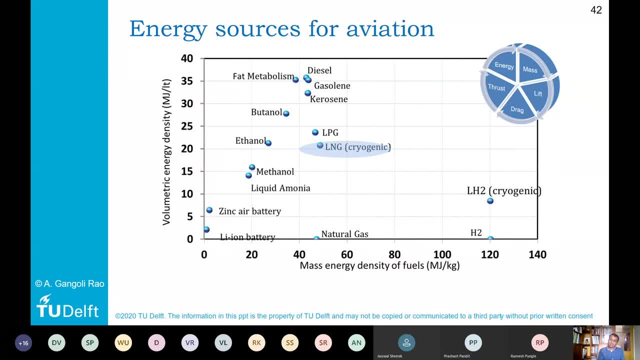 some of the trade-off criteria which we have to always take into account whenever we design the propulsion system as well as the aircraft, and one of the main things that we have to keep in mind is that if the mass of the aircraft increases for some reason, yeah, either it is because the poor 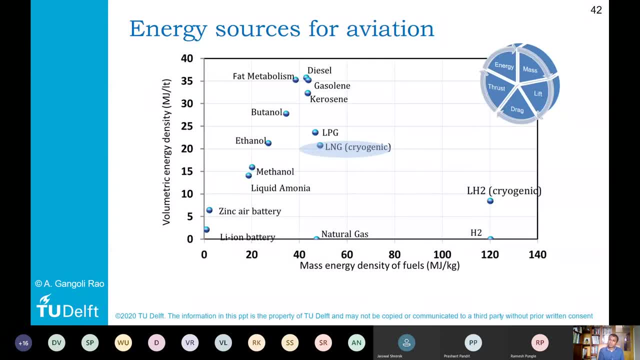 structure, or is because of the additional mass of the fuel or something, and so on. so then that means that, uh, because of the mass increases, and the lift of the aircraft has to increase, and because the lift increases, the drag of the aircraft increases as well. okay, which means that the thrust produced 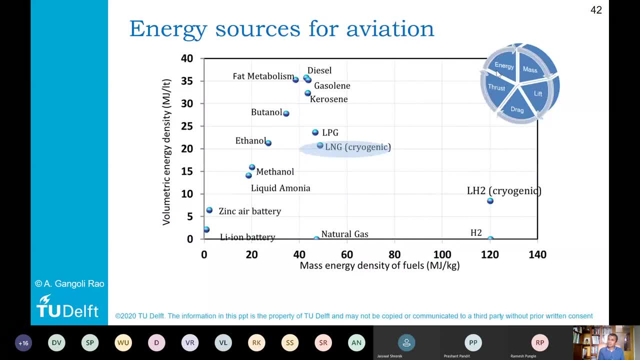 by the engines, they have to increase. and if the thrust produced by the engine has to increase, that means that the amount of energy that they consume also increases and that means that the weight increases as well. so when you look at at a, at a big aircraft, let's say, for example, uh a380 for 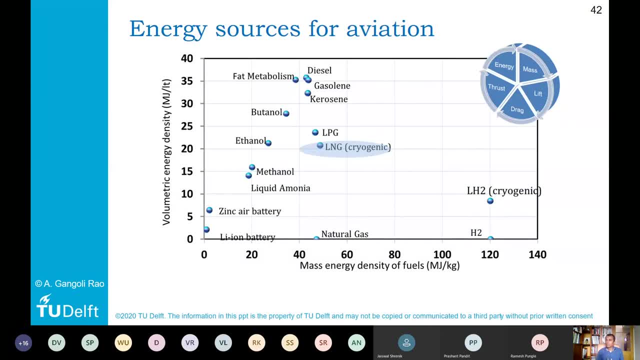 example, on a long range mission, then the amount of fuel is approximately 200 tons. yeah, that's huge okay, even when you look at uh, seven, seven, three, seven or a320 kind of an aircraft, uh, which goes on a on a 2000 kilometer range, yeah, the amount of fuel that is required is around eight, nine tons. 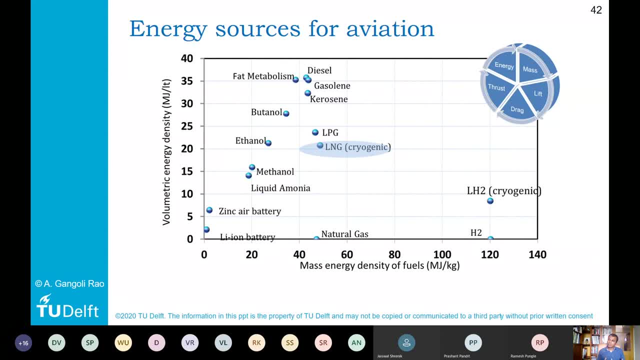 okay, so, so you see that, um, uh, you know, the amount of fuel that is carried on by an aircraft is actually, uh, sometimes even more, as compared to the, to the payload weight, which means that the passengers and the luggage and the payload and so on. okay so, the fuel weight cannot be neglected at all in a car. it's a. 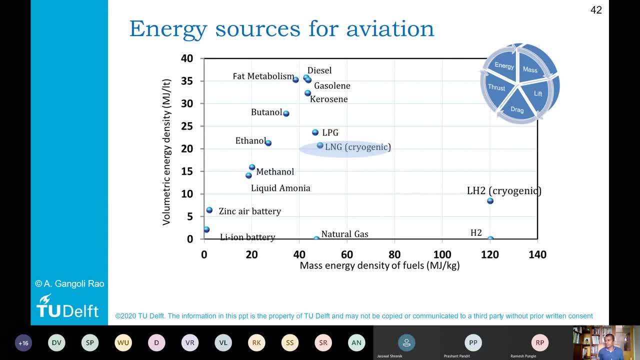 different case. yeah, right, so in a car is typically around 40- 50 liter tank, yeah, and the. the weight of the fuel and the tank is roughly several hundred kilograms per hour. but when you look at the klimat- not you know it's- it's sort of negligible as compared to the way that. 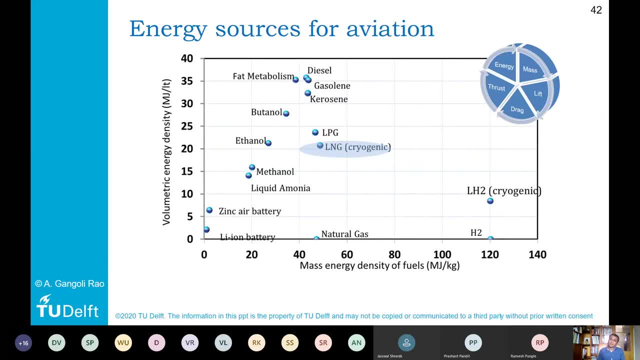 of the car or the weight of the passengers, but in an aircraft it is completely different. now, just for the fun of it, I put here: sugar has also very high calories. so in case, if you want to reduce weight, then avoid sugar, okay. well, we also have to keep in mind that if you start using other fuels, then they might. 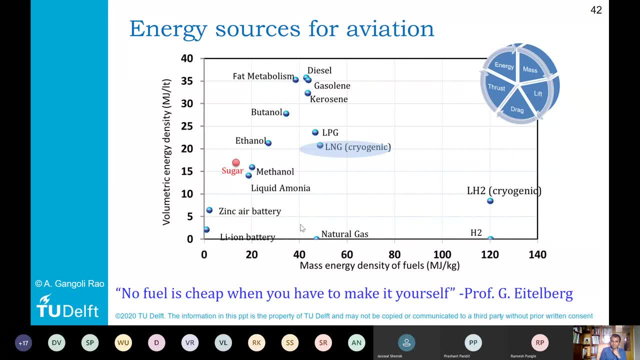 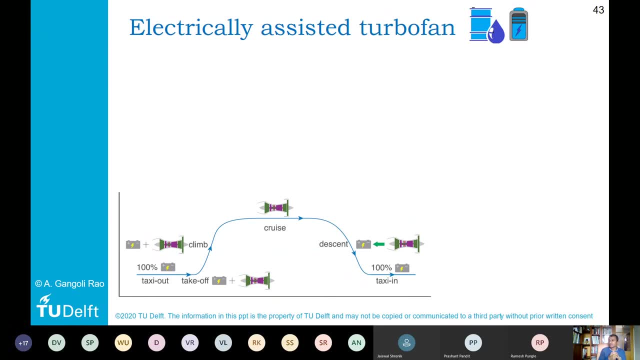 be expensive as compared to kerosene. now, now, what are we looking at, actually? so most of the projects that we are doing are in conjunction with Airbus or European Commission? yeah, and we are looking at ways in terms of how to make aircraft more efficient and less. 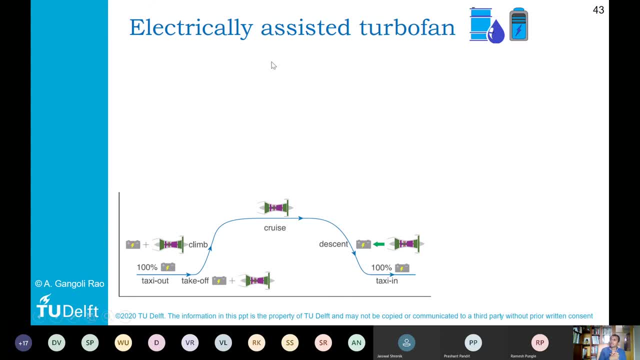 polluting, okay, so how to make them sustainable? and this is an example where how we are looking- I mean we are looking at, let's say, hybrid electric systems as well- to see if we can use electric motors to boost the power of the of the engine at some phases, so that we can design it for a 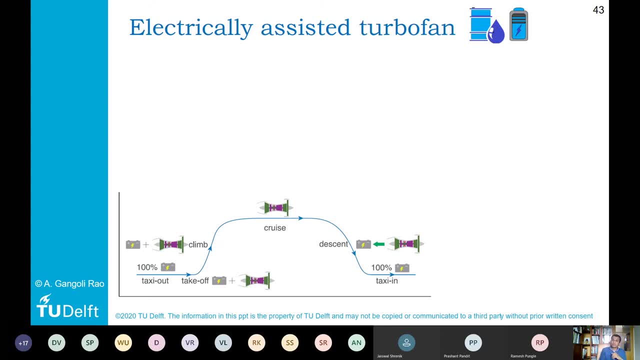 better operating point and that is during the cruise. so we have looked at hybrid electric systems, where we have looked at, let's say, incorporation of electric motors within the gas turbine in order to for the electric motor to boost, and also for taxiing and so on, we can use only motors instead of engines. 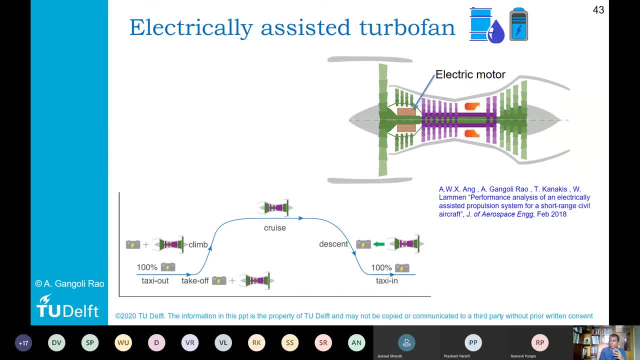 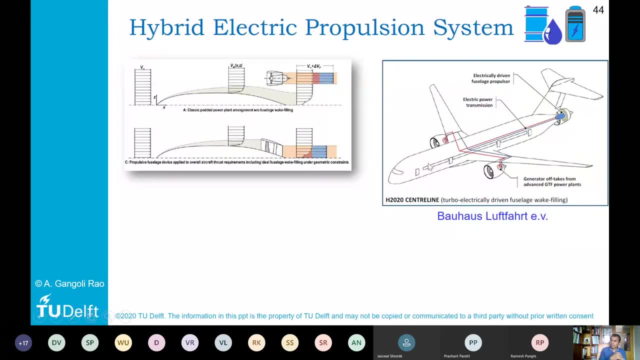 so that can reduce a lot of local air pollution. so these are become. these are some of the concept that we have looked at. I have also mentioned some of the publications. now we are also active in another European project along with Airbus and Bauhaus-Lutfarm from Germany and some other universities. so 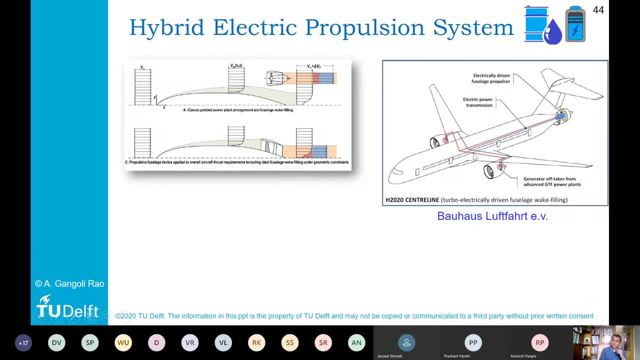 where we are looking at again a hybrid electric architecture where we use a very interesting technology, what is called as boundary layer ingestion. I do not have the time to go inside to the details of this technology, but nevertheless this is a very interesting technology in terms of how we can integrate engines as well. 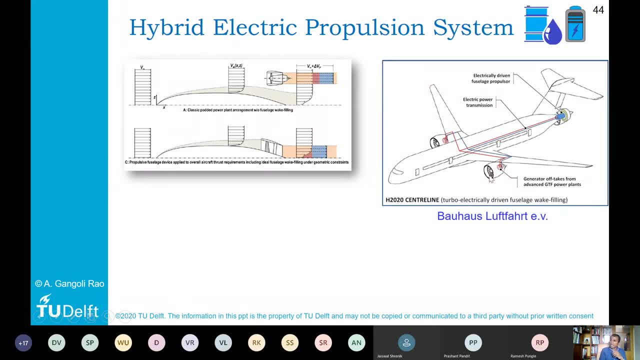 as aircraft and we are using hybrid engine, hybrid electric architecture to see if we can design, let's say, a future twin-aisle aircraft using this technology. and yeah, so this is. this project is almost ending now. okay, so this is a schematic of the aircraft, what you see here. so these are the two regular gas. 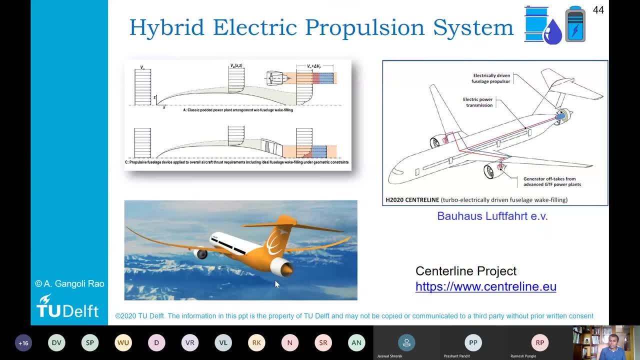 turbines. so this one and this one, yeah, and the third one at the back. what you see here is an electrical driven fan, and the electricity required to drive this fan is actually coming from a generator, which is actually also driven by this engine as well. okay, and now there are. 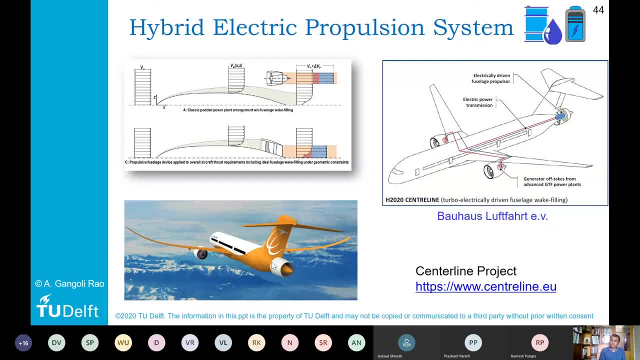 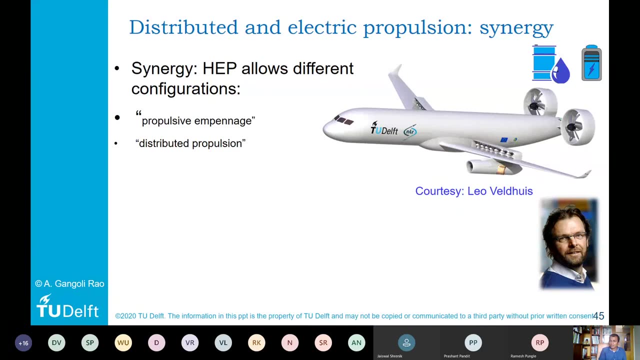 some advantages of putting in a fan here. this is what is called as the boundary layer ingestion. if you want to have some more details, then I have given the link of the project here. now we are also looking again along with Airbus, as well as NLR, which is the Dutch aerospace laboratories. we are looking at hybrid. 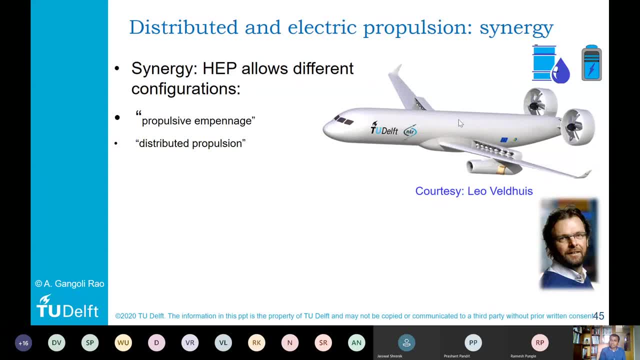 electric aircraft for single aisle aircraft, yeah, and here are some of the concepts. what you see is a what we call as a distributed propulsion. so there are several. so so these gas turbines, they generate only electricity and then it is distributed to, or a large number of propulsors here, as well as to some big. 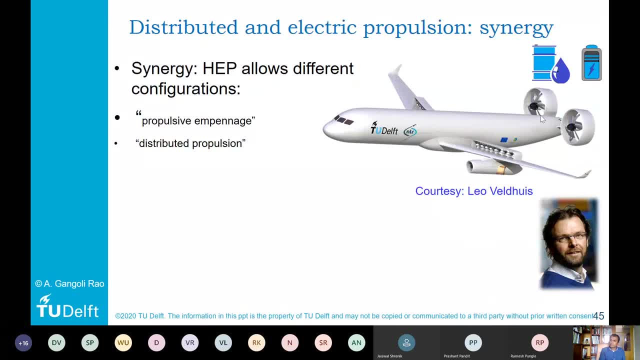 electric motors at the back, and what you see is that there is no tail. here is the tailless aircraft. in fact, all the stability characteristics required to make this, to control this aircraft, is coming from these two ducted fans. yeah, and they have thrust vector control at the back, and this is so. this is being. 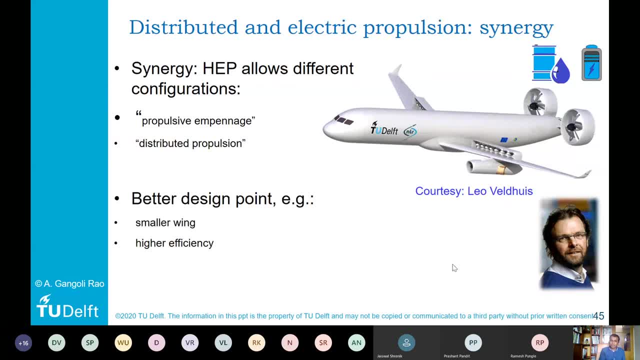 done by a one of my colleagues, professor Leo Felthaus. yeah, and while we are looking to exploit synergies between how we can sort of integrate distributed propulsion system with aircraft aerodynamics and aircraft design in general. okay, so here also, you see that we are looking at hybrid electric propulsion. so this: 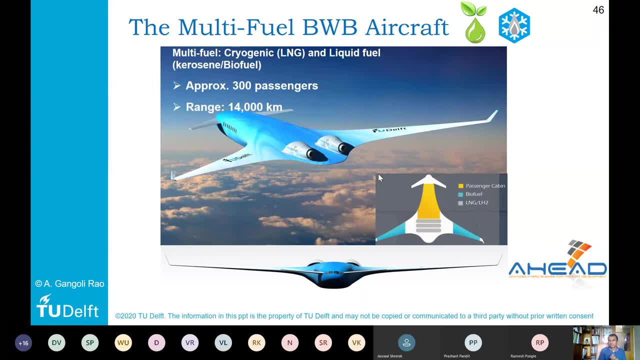 kerosene as well as electric propulsion. now, this is an example of a project that we did along with Pratt & Whitney and MTE and Airbus, and also by European Commission a few years back, and so this project has already ended in 2015, so I was heading this project where we 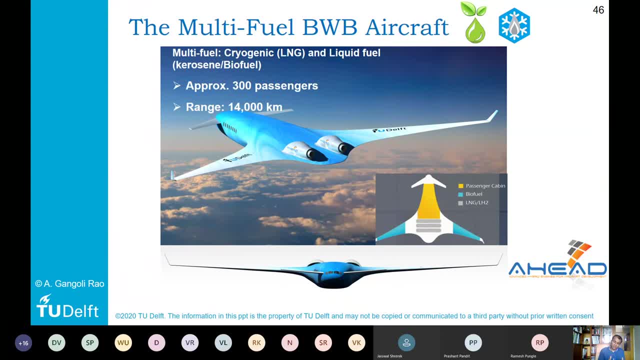 were looking into the future of aviation and asking: how are, how is, how are people going to fly in 2050? okay, so we looked at the applicability of cryogenic fuels like LNG, each defined carbons, gas and and liquid hydrogen, as well as biofuels, in aviation now. so 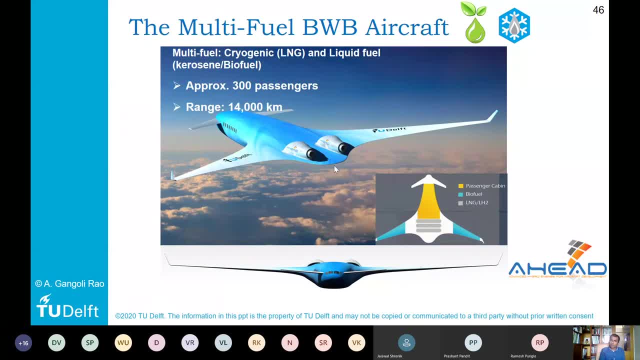 so you see this, what is called as a blended wing body aircraft. it had two engines and these two engines what we call as hybrid engines, because they use two energy source- i'll show you a schematic in a while- and it uses canards as a stabilizing surface, yeah, as a controlling surface, yeah, um. 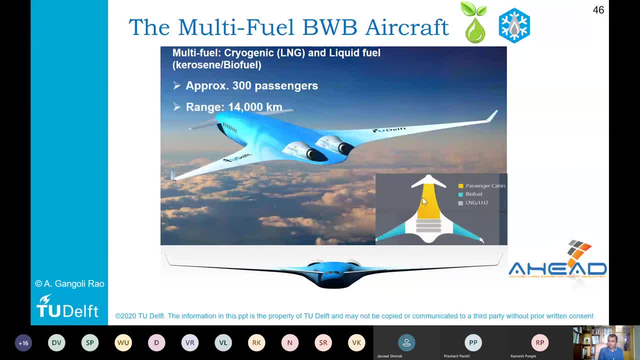 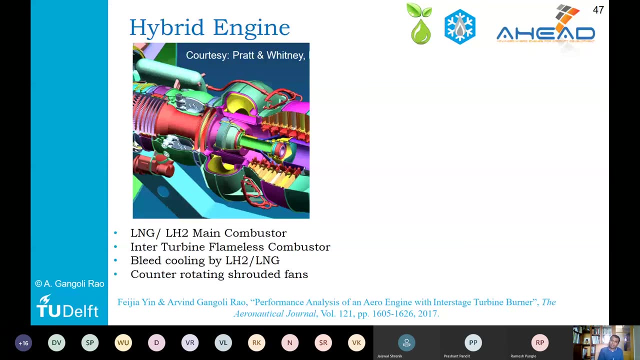 so here you see the schematic of this aircraft. so the blue- sorry, the yellow- one is the passenger section, these are the tanks to store lng and these the the blue one- what you see here is the biofuel. okay, so one of the things highlights of this project was 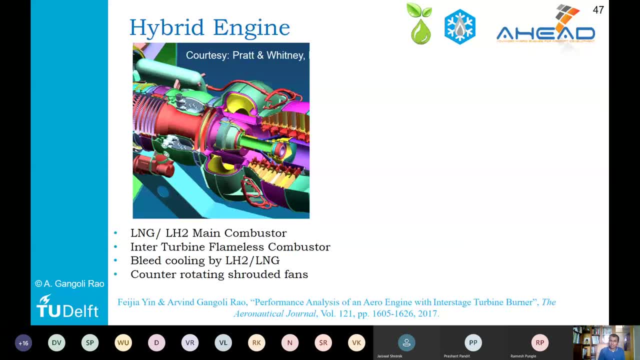 we designed a different kind of engine and so it had two combustion chambers. so the first combustion chamber uh was in between the compressor and the turbine, like what i showed you in a normal turbojet. but it also had a second combustion chamber and this, this toroidal second combustion chamber, between the high pressure turbine and 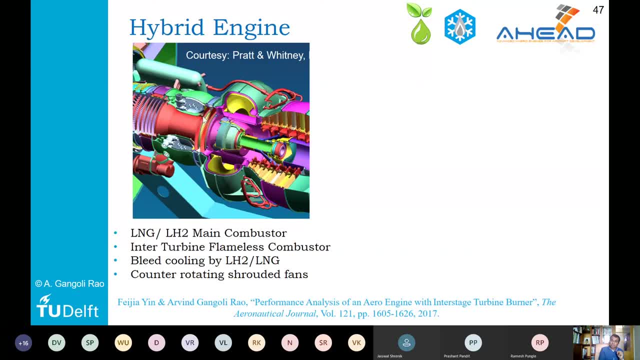 the low pressure turbine. okay, um, and so, which means that this, the first combustion chamber, could use uh, lng or methane or hydrogen, whereas the second combustion chamber could use biofuels. yeah, so this was a what was called as an hybrid engine, and it had some several advantages, and 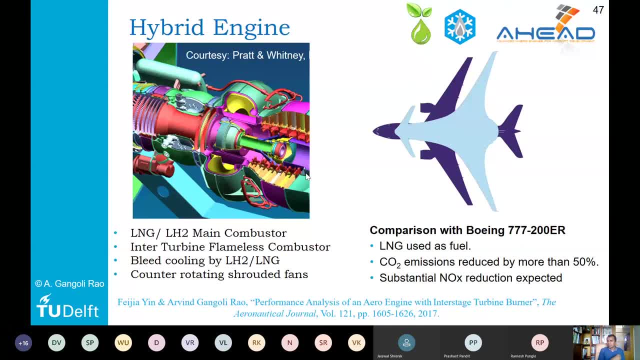 we proved that by using such a architecture, uh, such a novel engine, as well as aircraft architecture, we could reduce the fuel consumption for a long range emission as compared to a triple seven aircraft going triple seven. so this dark blue one that you see here is a going triple seven. 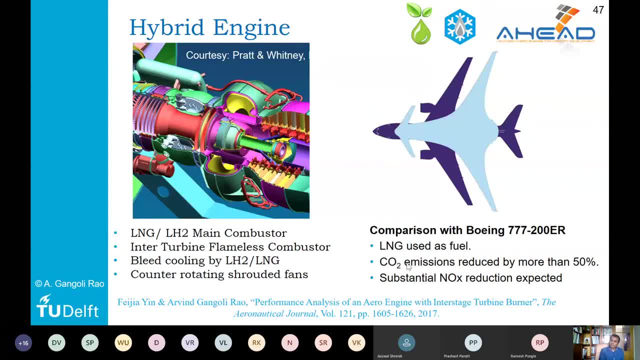 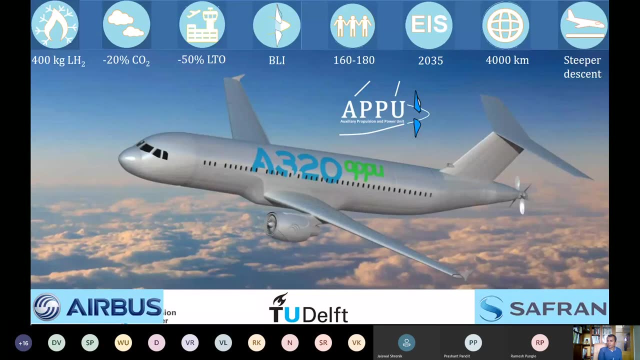 and the light blue one is the aircraft that was designed by us, and what you see is that we could reduce co2 emission by approximately 50 percent and we could reduce nox emission by approximately around 85 to 90 percent, and this is an example of a very new, latest project that we started. 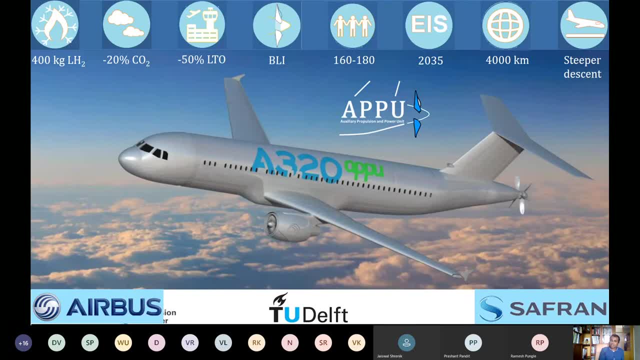 just a couple of weeks back, also with airbus, as well as with safran, where we are looking at using also hydrogen along with kerosene in aviation. this is supposed to be for the next generation of a320 neo that will come in around 2035.. 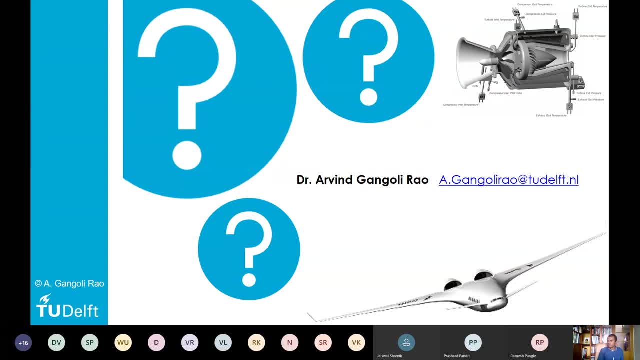 yes, so with that i would like to close my presentation. of course, if you have any questions, then please feel free to ask. thank you, thank you, sir. you're welcome. if anybody has question, please ask the questions now. one question from my side. yes, now you have shown one slide that during climbing 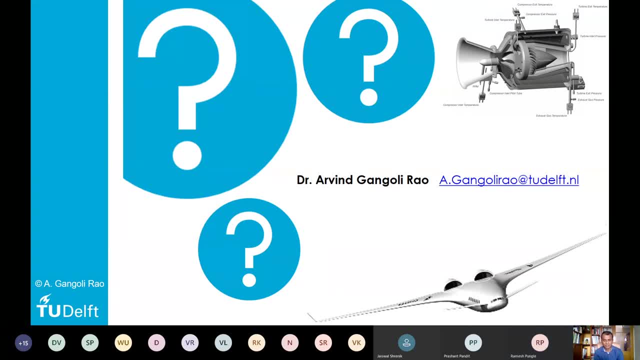 every time atmospheric conditions are not constant, so how the engine take that particular load and adjust the power during climbing. so that's a very good question actually, because at taking off you have a temperature of, let's say, around 30 degrees and then atmospheric pressure of, you know, 1.01 bars. but when you are climbing, of course the altitude is changing, so the pressure is reduced. now thebodys said: take care of theentedima budget, so that the visual function changes every time because the temperature is reduced but that atmosphere is reduced, So thebere edges are different, So that we will have to control the entire structure. tension there you, Africa, so you don't face the extreme atmospheric Really? yes, So that's a very good question actually, because at take off you have a temperature of this, are on 30 degrees, and then atmospheric pressure of you know, dig the s, but when you are climbing, of course the altitude is changing, so the pressure is reduced. but then, whenever you are climbing, of course if you have a load- Ó Gary Berry has it within the wholeements这个 liggervä. 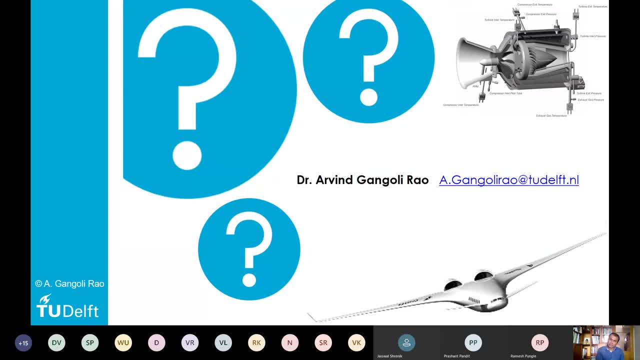 and the temperature is also reducing. but that is not a problem actually, in the sense that the engine is designed for that. okay, so the inlet conditions are changing, but- and of course the velocity of the aircraft is also changing. but the inlet is designed so that it provides the sufficient mass flow rate at all. 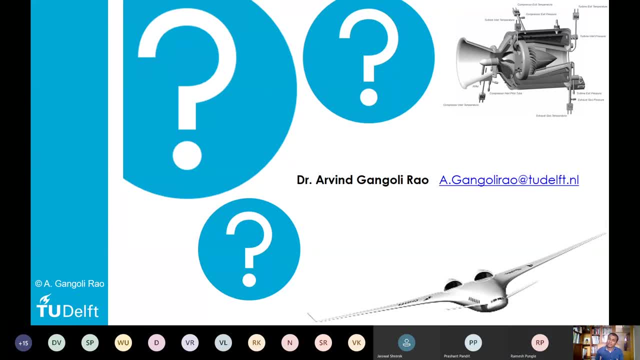 conditions, and the compressor and the fan are also designed to work on different operating conditions. okay, so, yeah, so the aircraft engine is designed for that- I'm the turbo machinery, especially the design for this. okay, and we elaborate that how different forces is balanced so that we get the resultant. 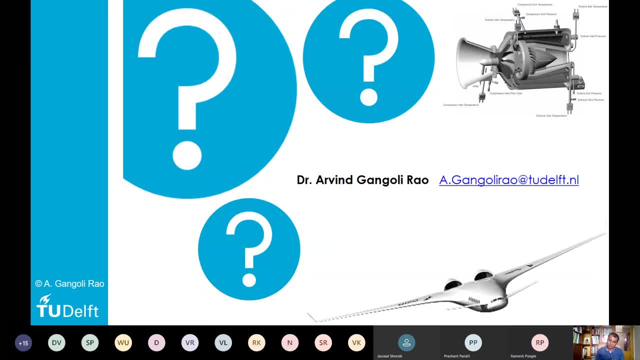 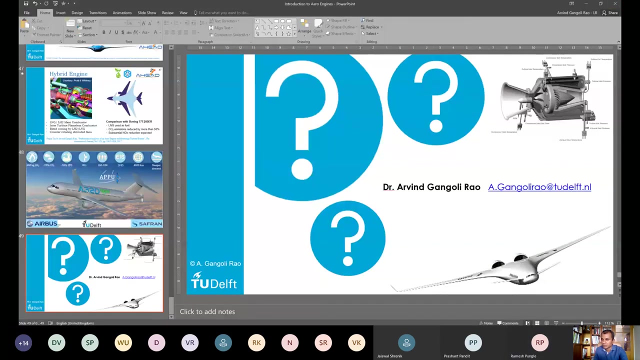 force that will climb the aircraft, okay. I don't have a schematic at the moment to show that, but you see that during a climb, let's say first we have to look at what happens in a cruise, let's say okay, and then we can discuss what would happen in climb. yeah, let me see if I can pull out. 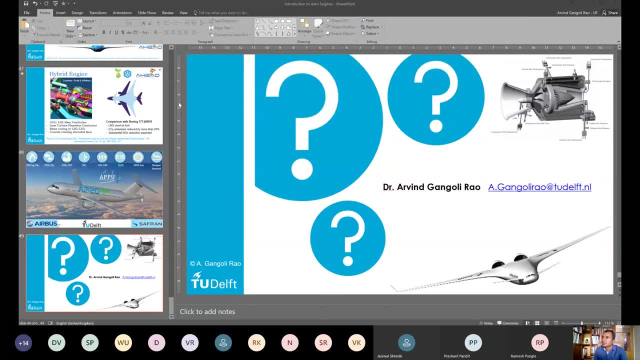 you just one second. do you see a slide? yes, yes, okay, so so this is again. so let's see what happens in in air during cruise conditions. so this is an equipped cruise condition. right then, equilibrium condition: you have the weight of the aircraft. okay, now this weight of the aircraft has to be balanced by the lift that is generated by the wings. yes, and so. 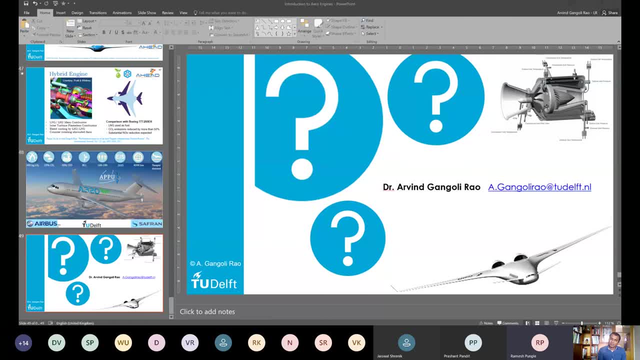 that the wing is the main, the lifting surface. okay, yes, now in in the process of creating this lift, it also creates drag, okay, and so this is the resultant of the drag, and this drag has to be then balanced by the thrust. okay, now what happens, of course, is, during climb, there are, there are a 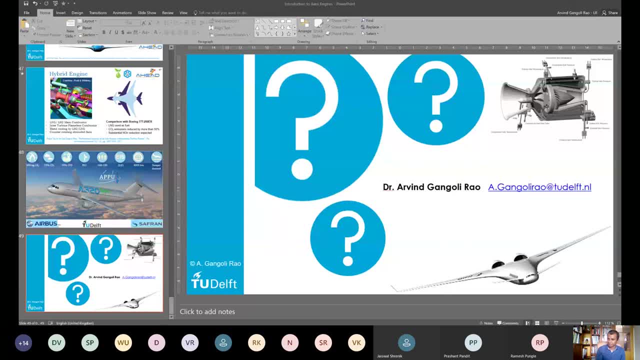 couple of more things. first of all is that the aircraft is also accelerating. yes, so that power has to be. so you, you require energy to accelerate, so so that means that that energy has to be provided by the thrust. secondly is that, let's say, during cruise, the angle of attack is not so much so, it's more or less horizontal, like what? 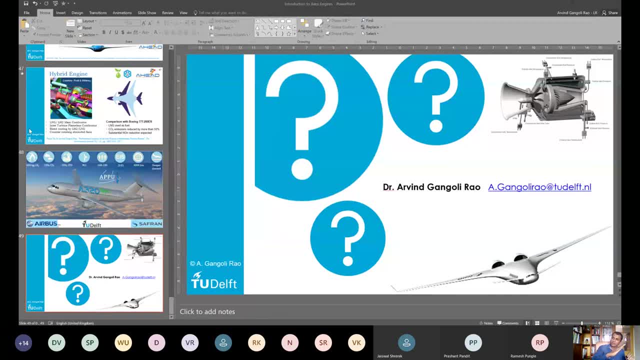 is shown here. but in incline it is also climbing, so you, so you have a gradient, so of course then you have to take the components of the weight and the lift in the respective directions. that means the a large part of the lift. so because, because the wings are like this, so a large part. 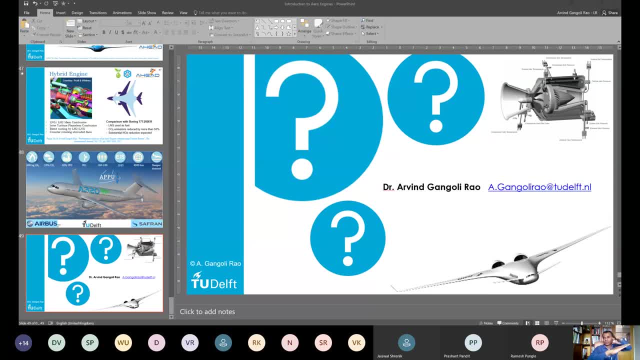 of the. you know you have to uh so the, so the lift is like more or less like this: so you have one vertical component and then the, then the horizontal component as well, and that horizontal component is actually, uh, that's sort of the drag, okay. so so these uh things, uh, you have to take into account. 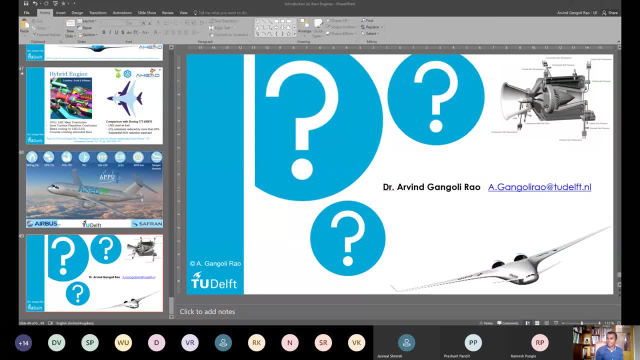